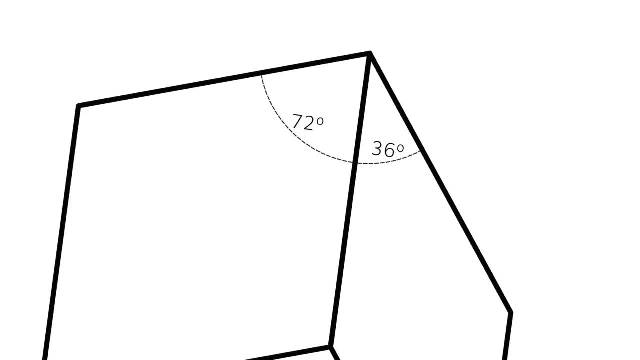 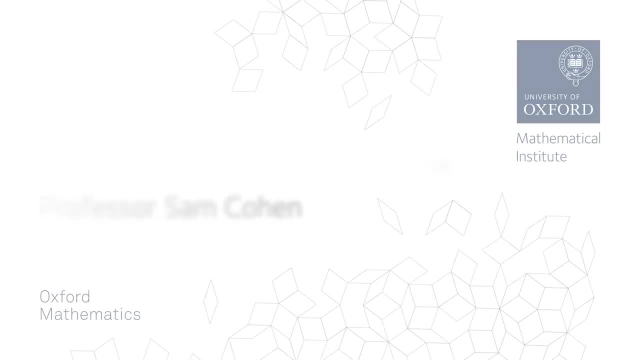 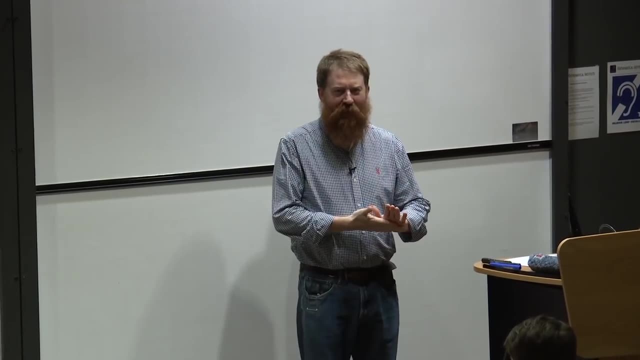 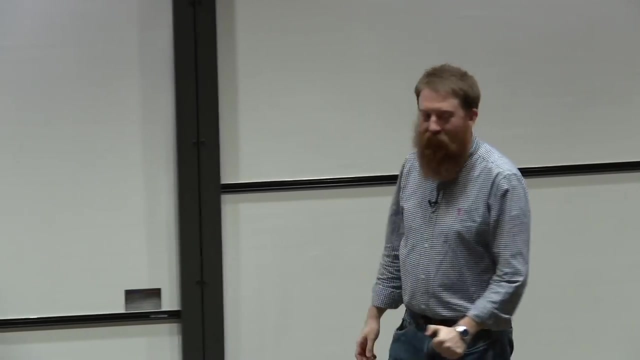 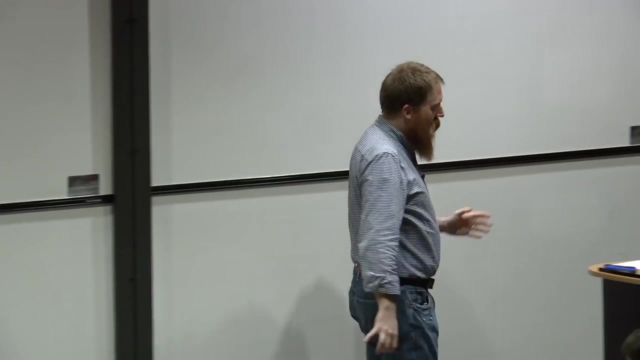 Okay, good morning, Welcome to 2020.. I guess this is the first lecture for at least some of you, So we're here today for mathematical models of financial derivatives. I'm Sam Cohen, I'm one of the lecturers here in Math Finance, And what we're going to do is 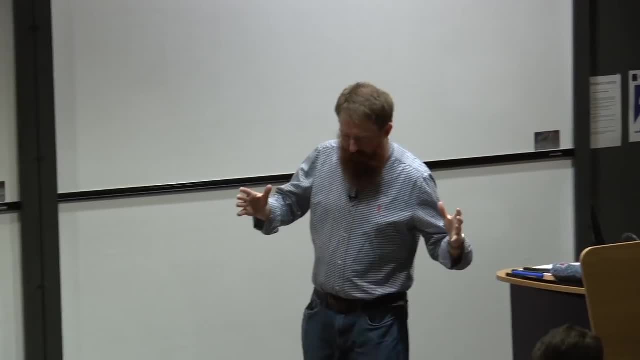 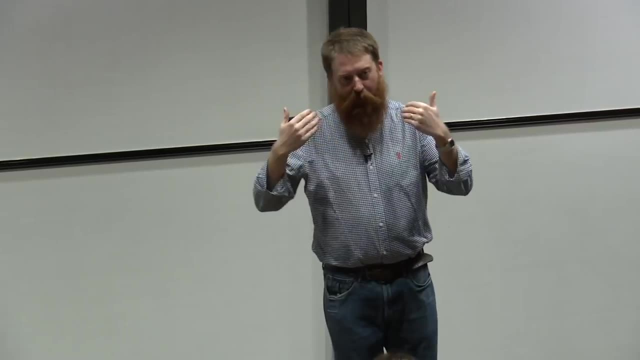 in this course we are going to try and understand some of the contracts that are commonly traded in finance. We're going to try and ask ourselves: how can we use mathematics to understand them better, How can we understand the risk, How can we manage it, How can we price it, Etc. 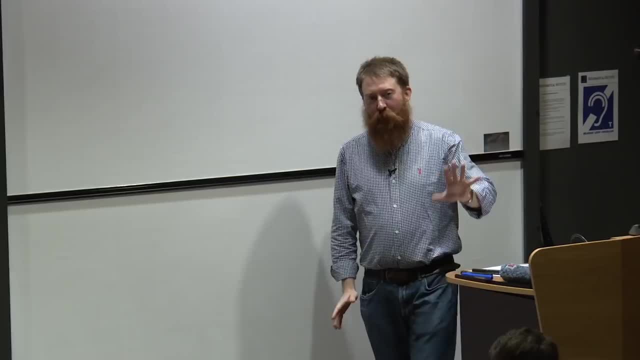 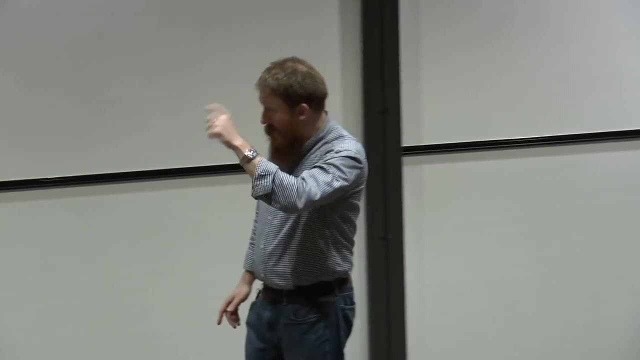 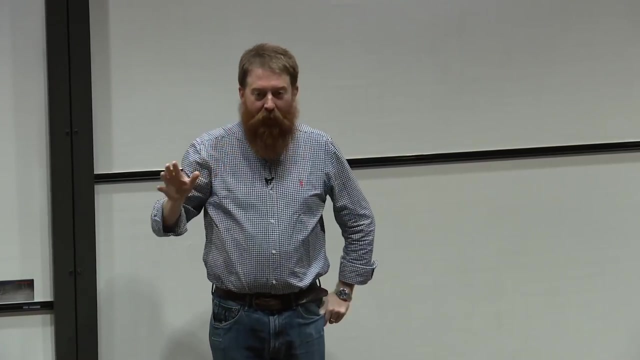 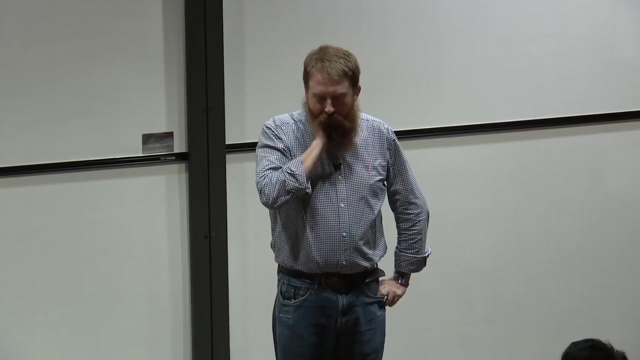 So, before we begin, we really should be asking ourselves: why are we wanting to do this? And it's a pertinent question because mathematical models of financial derivatives have been more than a little bit controversial. Now, you guys may not remember it as well as I do, but 12,, 13 years ago, 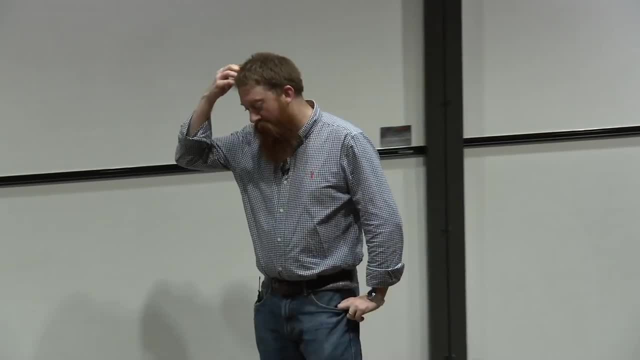 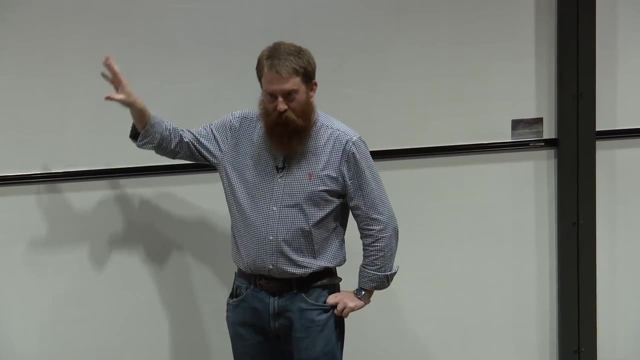 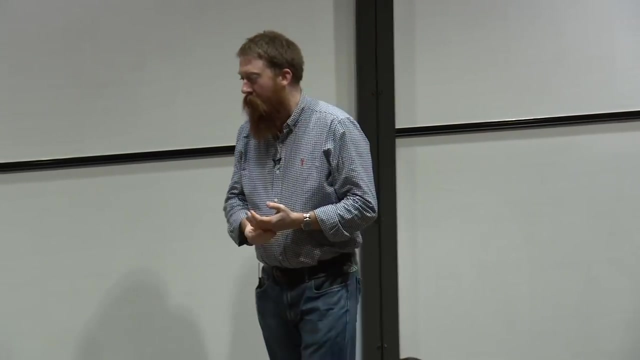 there was a very large financial crisis- the GFC- And one of the things that have been blamed for this was an over-reliance on mathematical models of financial derivatives. You've got the article, the formula that killed Wall Street, So is this a sensible thing for us to be studying at all? 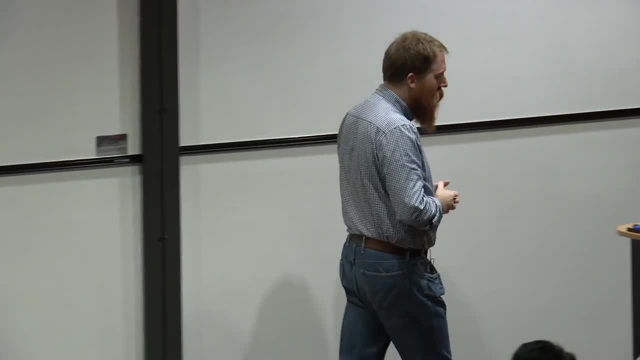 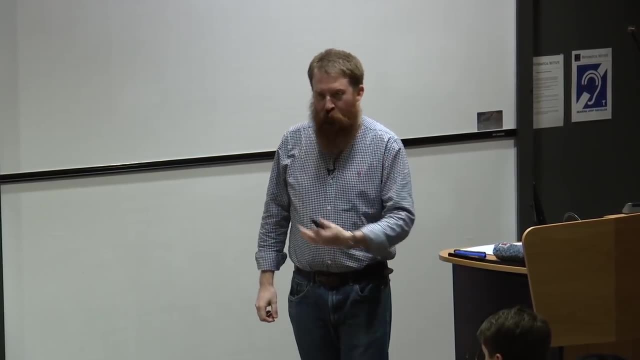 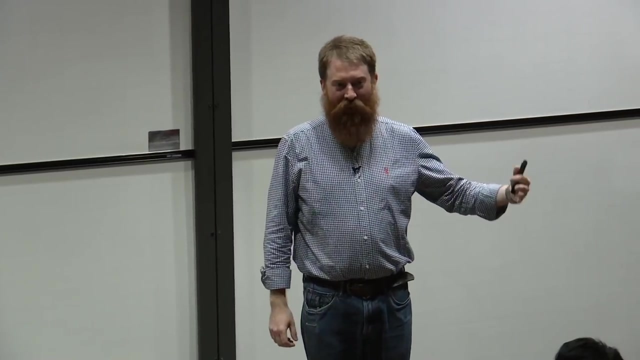 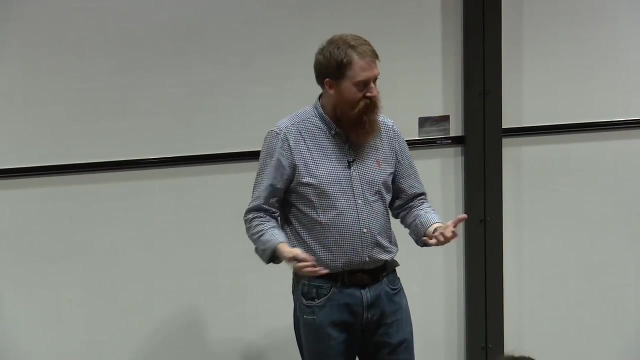 It's an open question, It's a serious one, I would argue. it is for a variety of reasons. As we'll see, financial derivatives have always existed. Pretty much since agriculture, we have had financial derivatives and because of that we we can't close our eyes to the fact that these things exist, that they are traded. 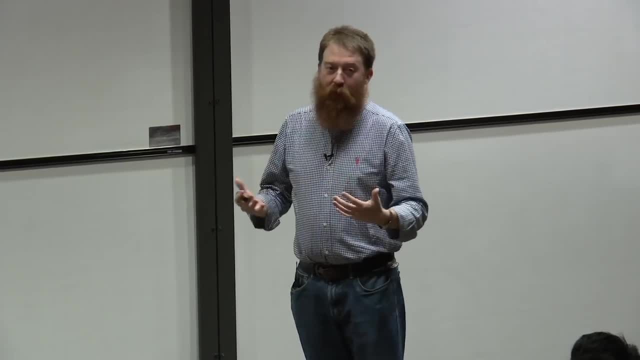 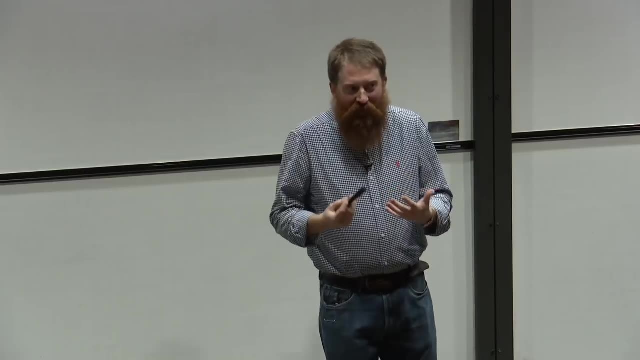 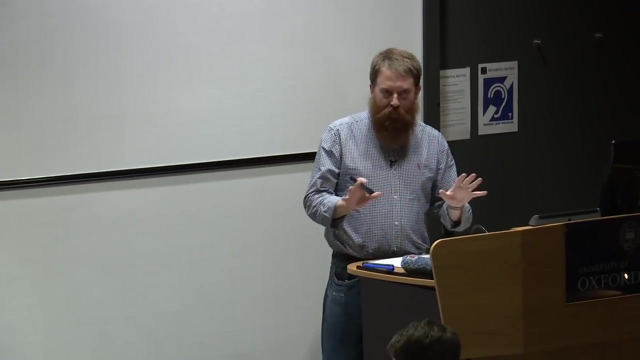 that they are real, and building models of them, trying to understand their risk, is a sensible thing to do. we also need to understand where those models are going to fail. we need to understand the restrictions of what we're doing, and so that's something I'm hoping that we'll touch on quite a lot in this course. 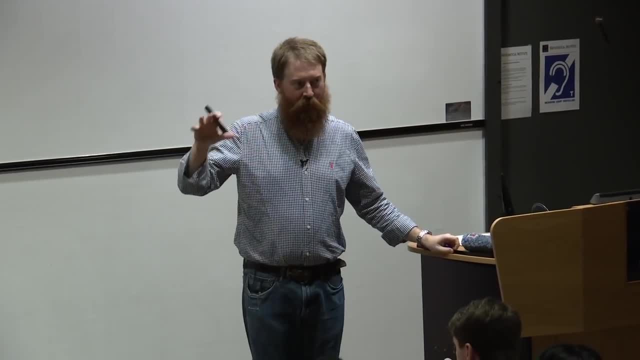 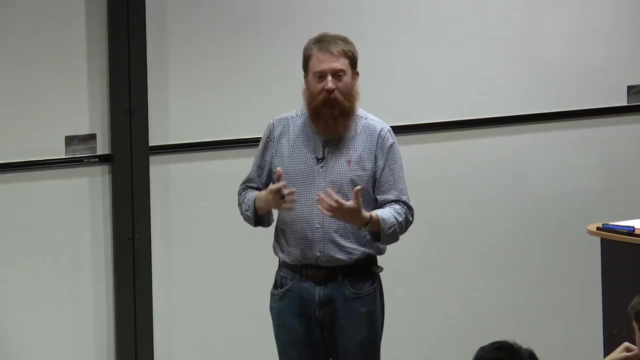 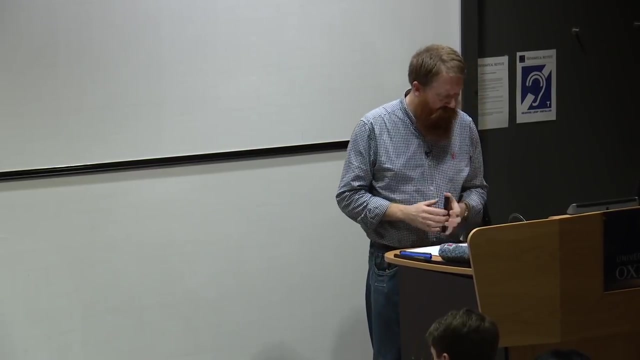 where is the model going to go wrong? where are the restrictions? where have we made abstractions or simplifications that are a little too brave, a little too far from reality, and I'm hoping that we'll cover some of those things as we go along. so what are we trying to actually do in this course? we are trying 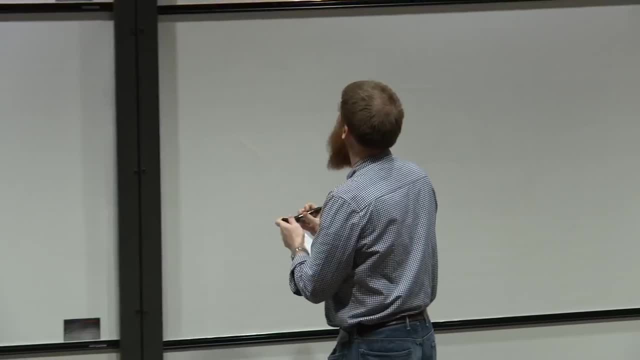 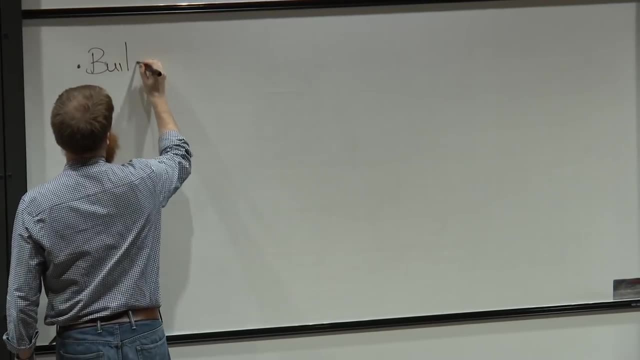 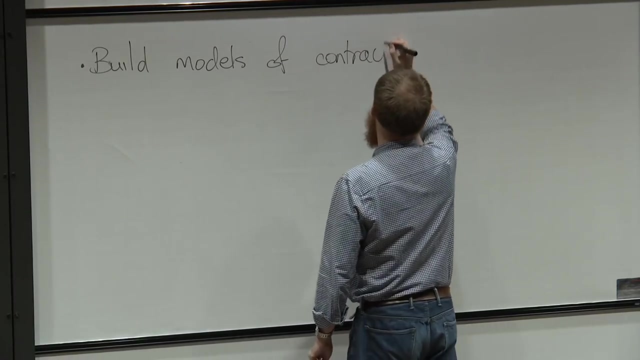 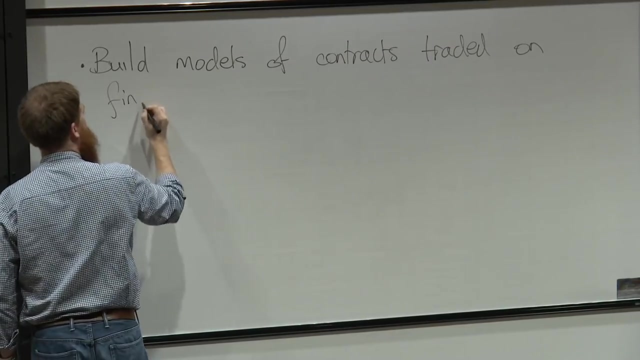 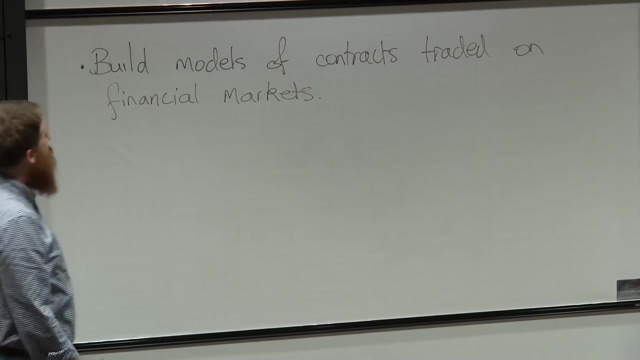 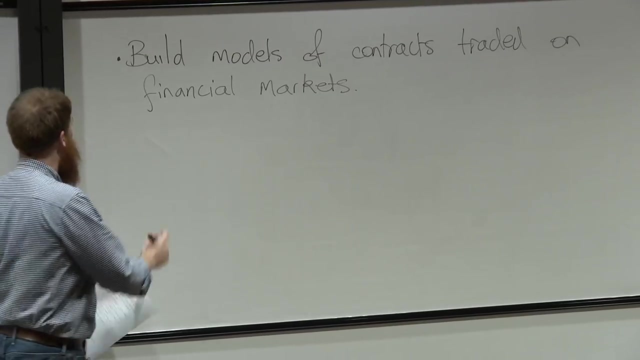 as I say, three broad goals. the first is to build models of contracts traded on financial markets. so that's the the basic idea of what we're going to be doing. we're going to try and build models of some of these contracts, we're going to try and understand their payoffs and then from that we want to. 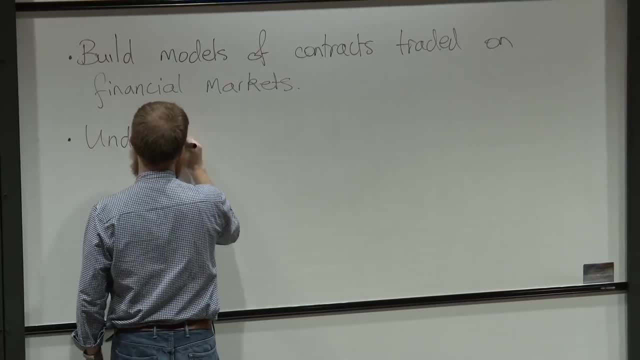 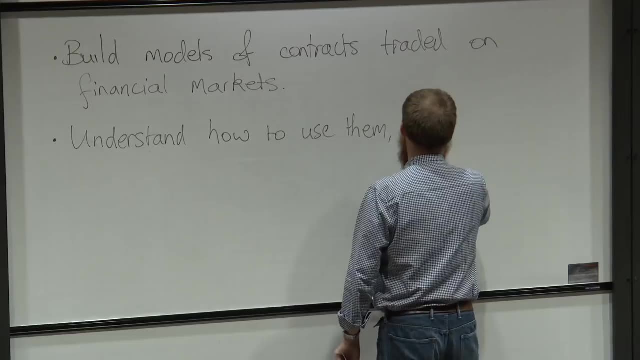 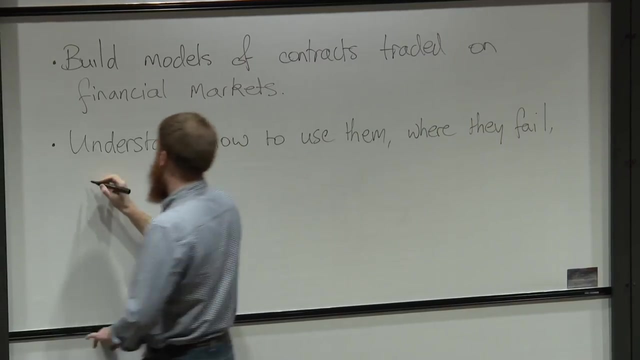 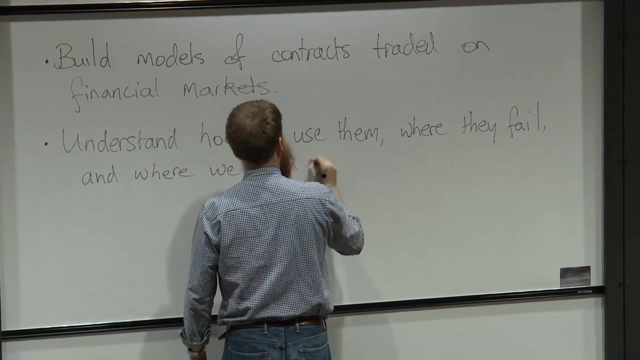 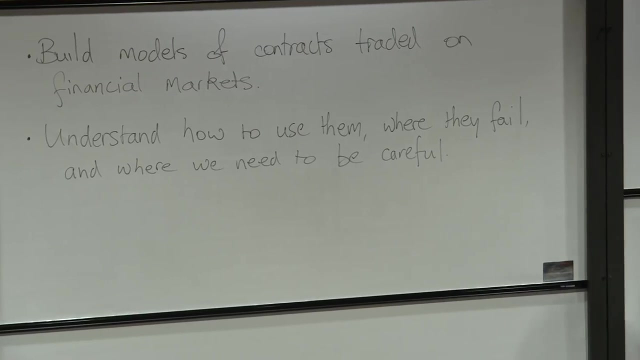 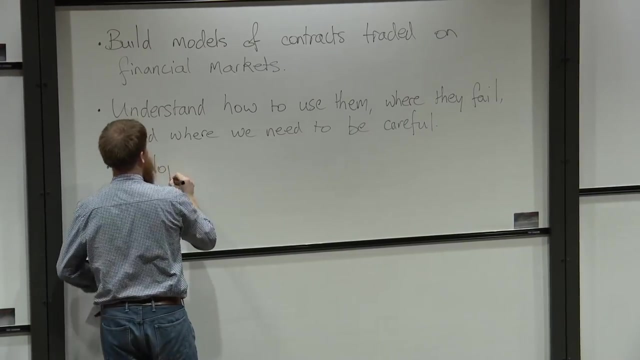 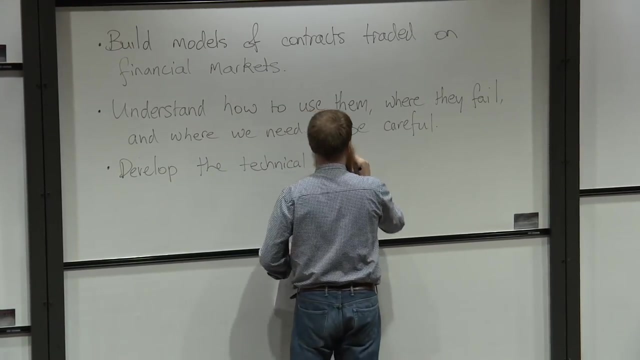 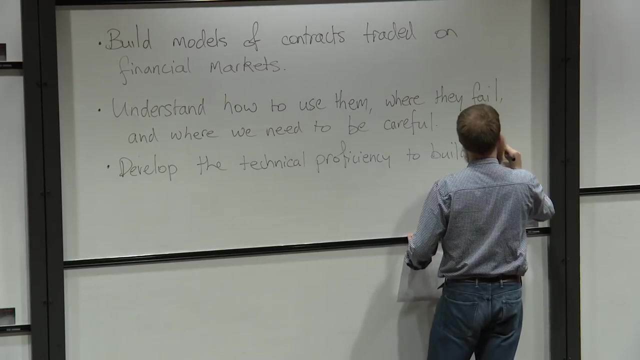 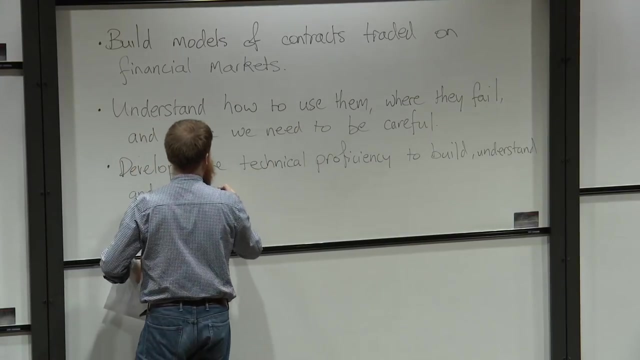 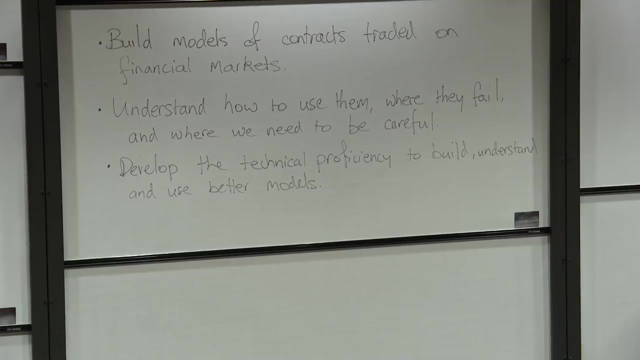 understand where they fail. we want to understand how to use them where they fail and where we need to take particular care. well, we need to be careful. and, as a third point, we want to develop the technical proficiency to build, understand and use better models. so this course is not the end point. we're not going to get 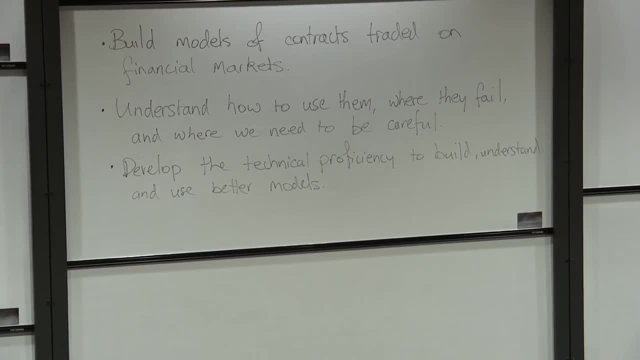 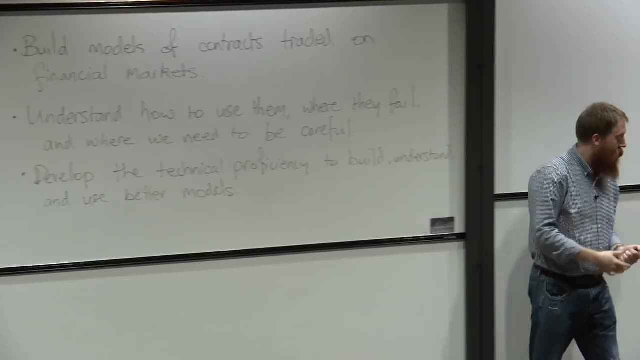 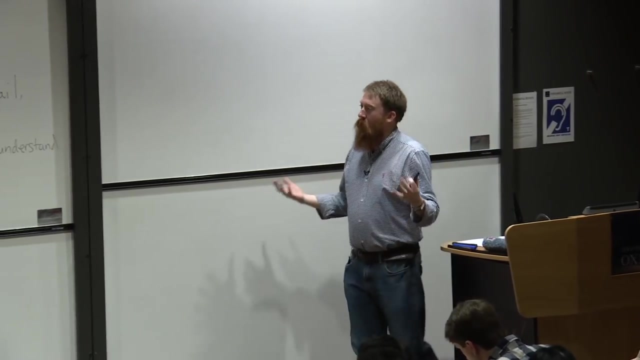 to the advanced things that one can do in the world of mathematical finance. but we're going to try and get enough technical proficiency that we could at least move on to that step at the end of this course. ok, so when we're building a model in finance, what are the key concerns now? 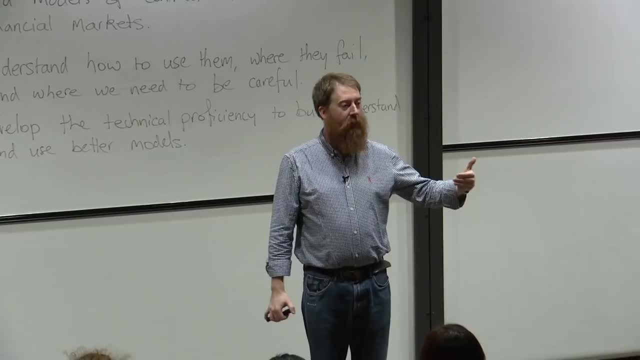 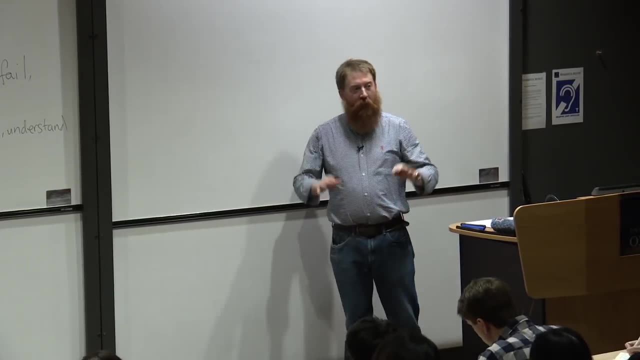 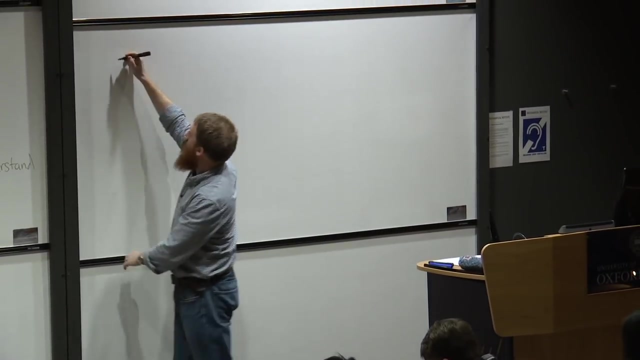 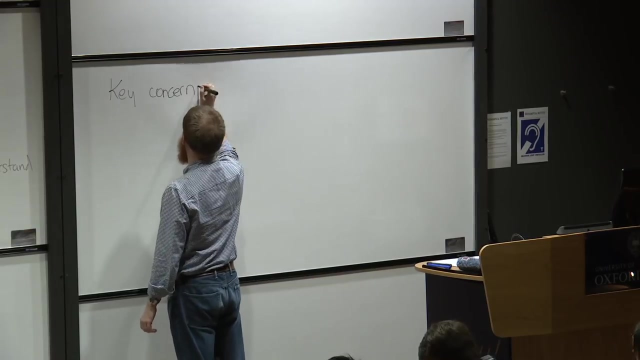 the usual thing people think is that you're trying to build a model so that you make money sounds good. the truth of the matter is that usually making money is not our first concern. usually our key concern in much financial modeling key concern is giving into the wrong people or thinking of people shouldn't give in and 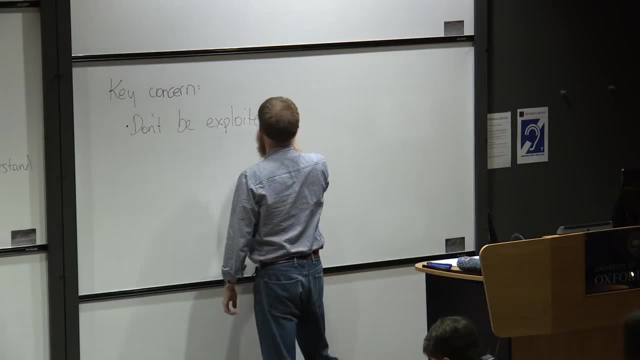 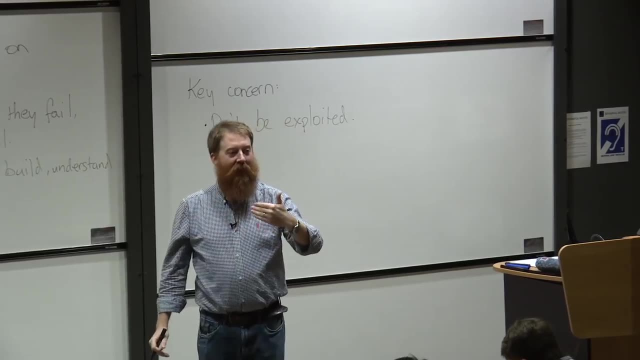 go out and do all kinds of useless work. so generally, Roseanna's question, I ask everyone that maybe has certain problems or other questions, all kinds of useful capabilities, all kinds of financial knowledge, but let's think the other question and you just do it and stuff until you get sort of the 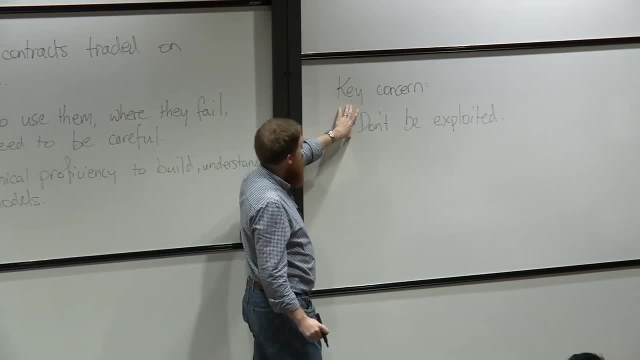 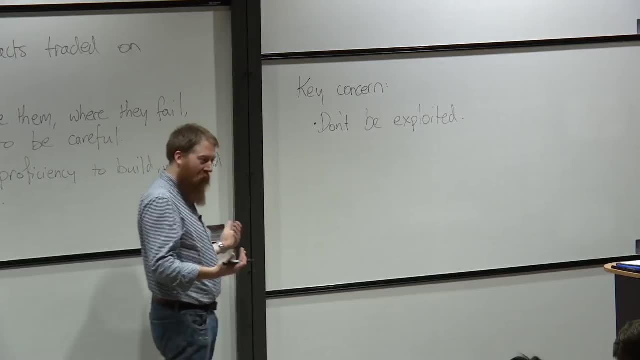 exact Monkey weiter. you want to ayaned it? just a cent range and we have four hundred thousand, 35 million people know a gold slowly, or banner, and each one of them is a hundred. things will be an. then we're not going to do very well, and so this is our first concern. Our second: 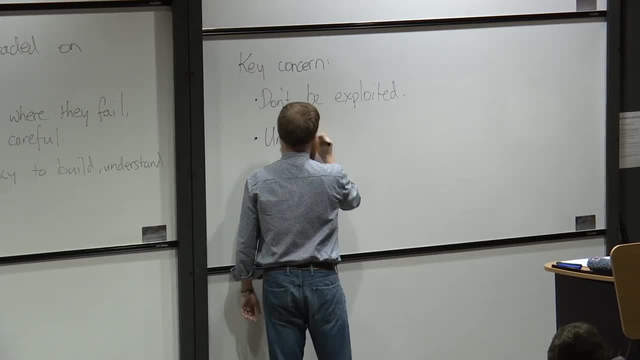 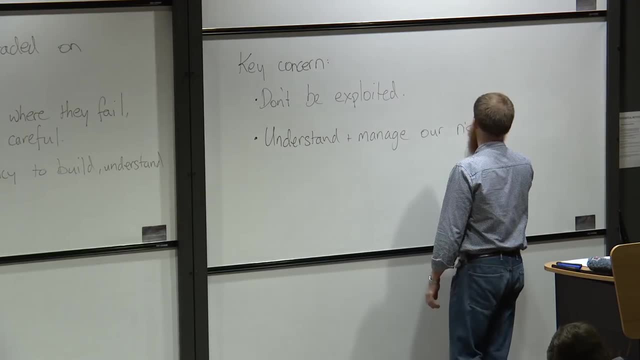 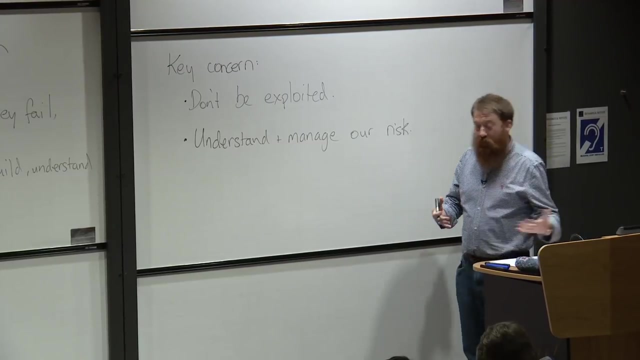 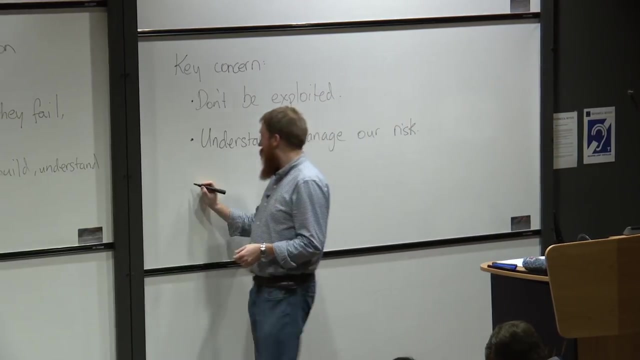 concern is we need to understand and manage our risk. It's not enough to have something which pays off well if it's so risky that we're going to lose before we win, and so we need to understand and manage our risk. and then a third goal is: 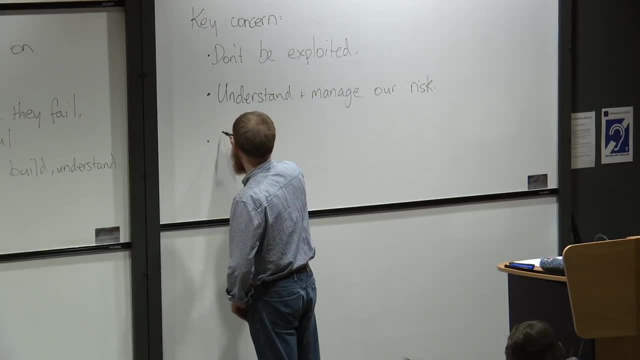 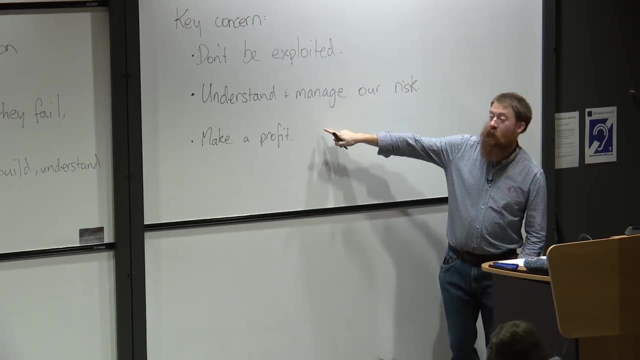 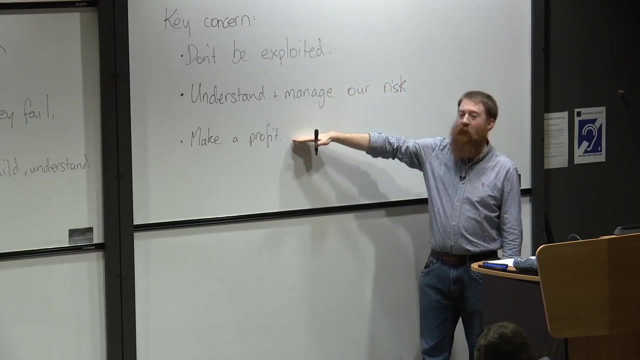 make a profit, but in what we do in this course, this is actually not going to be our key aim. We're going to be trying to understand these steps, because it's only once we've done these that this is even possible to even talk about making profit, unless you can understand your. 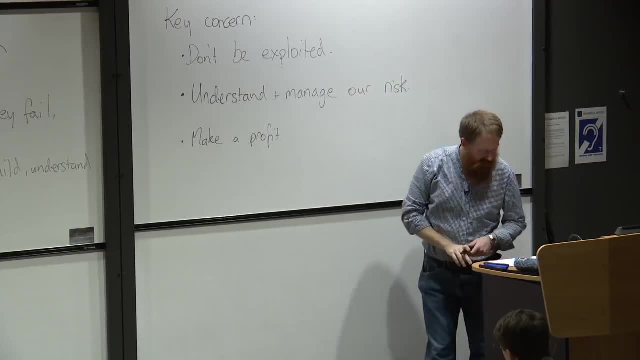 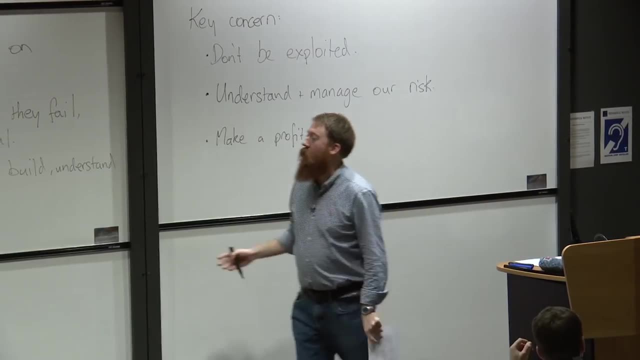 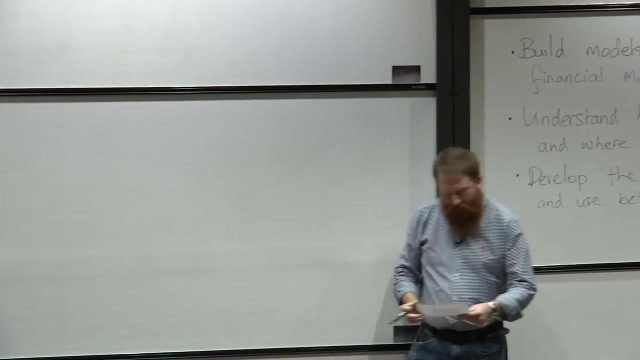 risk and you're sure you're not going to win. You're going to be exploited. There's no way you can turn a profit. Okay, so what are the economic assumptions that underlie most of our modeling? Let's try and start moving towards actually building a model of something. So we'll begin with a fairly simple set. 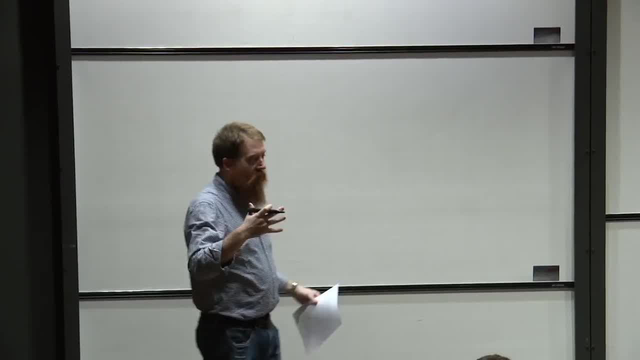 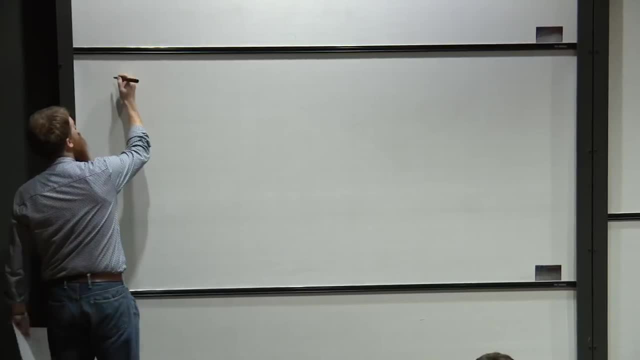 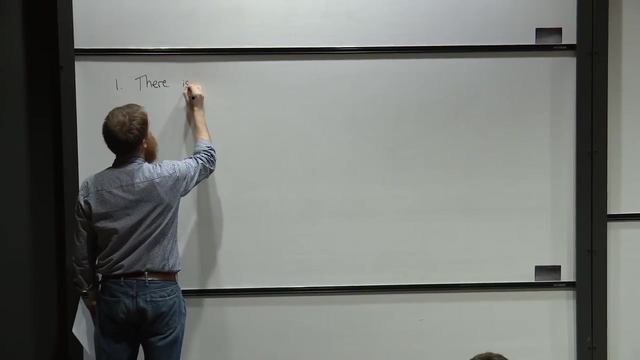 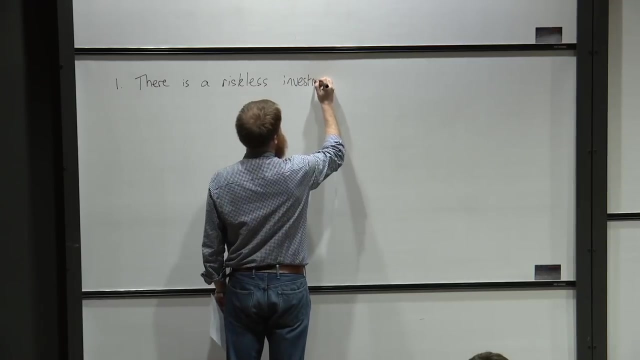 of assumptions about how financial markets work, and these are deliberately simplified, but they allow us to start making some conclusions. So the first assumption that we're going to use in a lot of the models is that there is a riskless investment. Now, what do I mean by? 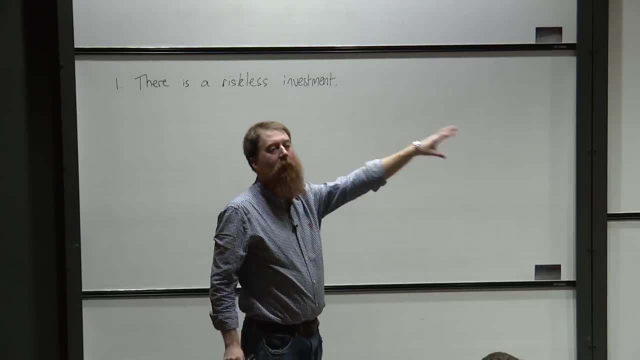 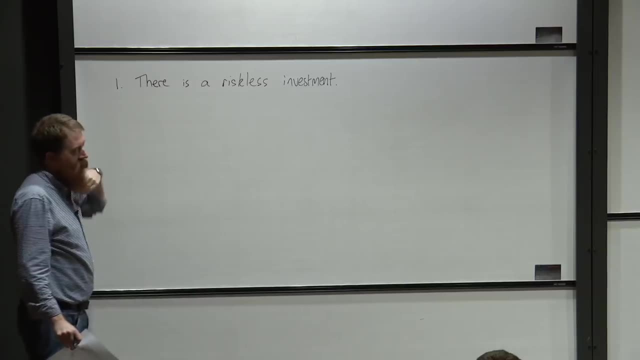 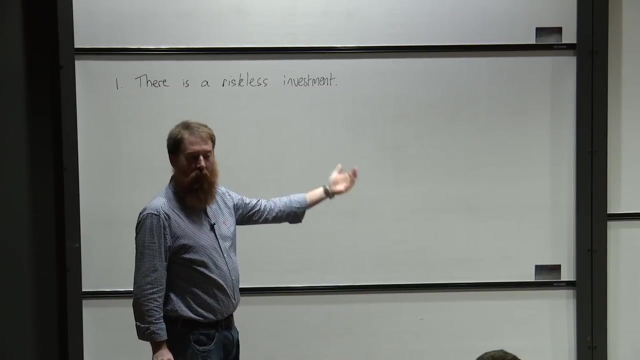 riskless. I mean that if I put money into it now, I know how much money I'm going to have in a year's time. So this is a common assumption. you can think of this as being cash or, more usually, as being a bond or a bank account with a fixed interest rate. I can invest in it today. 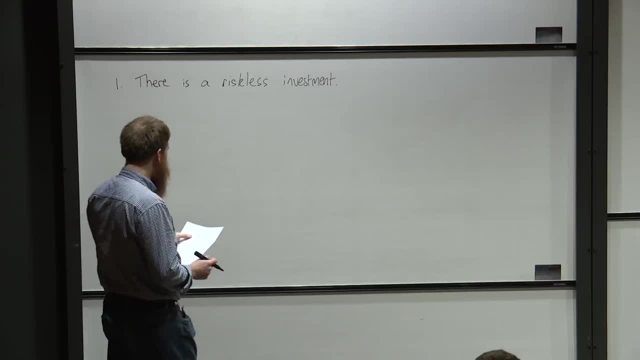 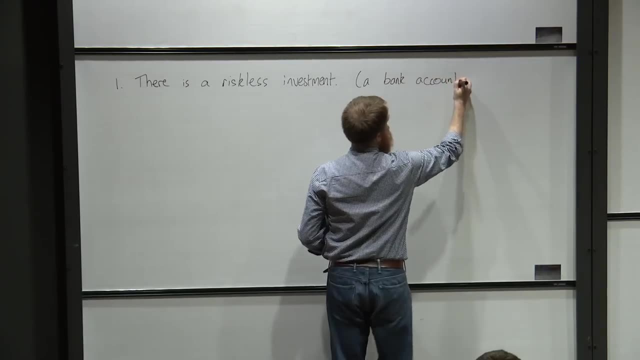 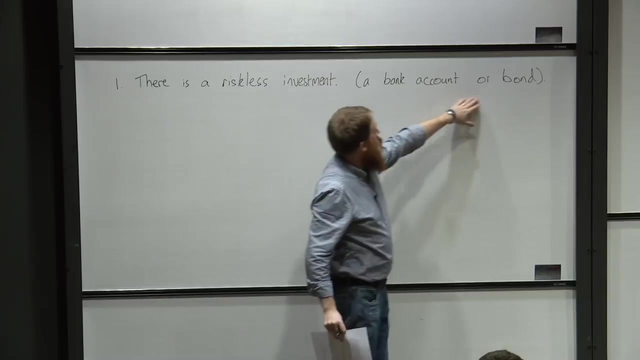 and I know how much money I'm going to have in the future. so we'll often refer to this either as a bank account or a bond. if you're not sure, a bond is just a, an agreement to pay in the future. if I thought of it, I would have. I have one in. 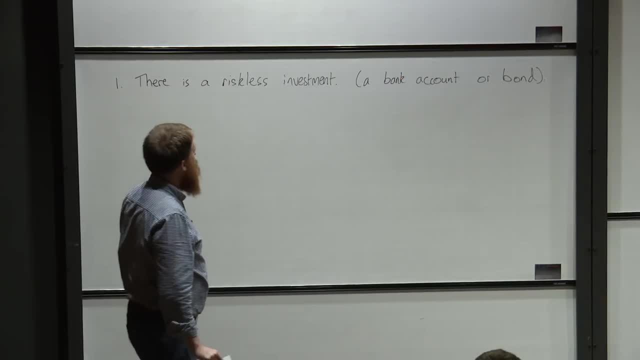 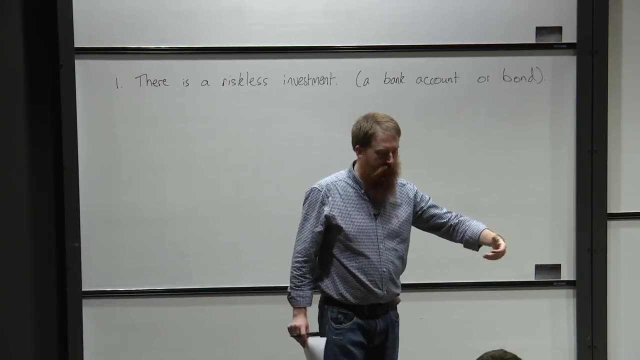 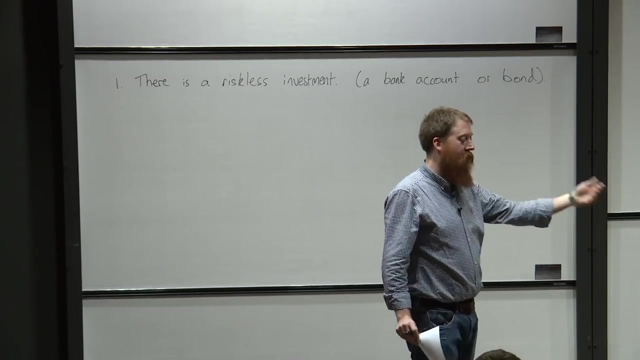 my office an old physical bond. it's a contract where what you do is a company or government will issue bonds, they sell them in the market and they give the holder of the bond the right to certain cash flows. so if you buy a bond, you then can go to the company and every month or however often the payment is, they will. 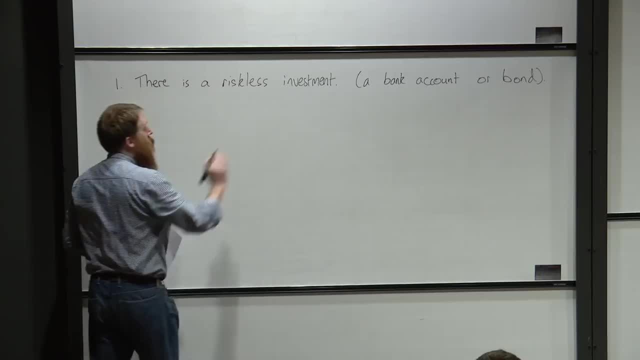 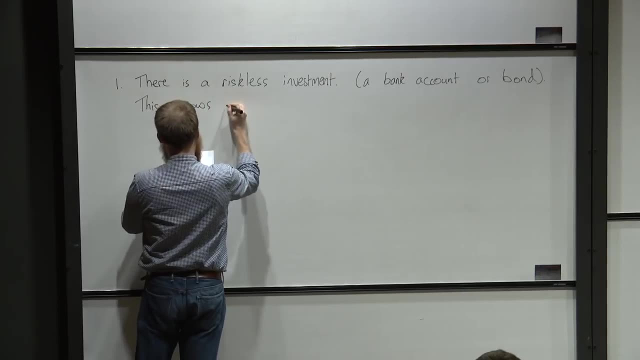 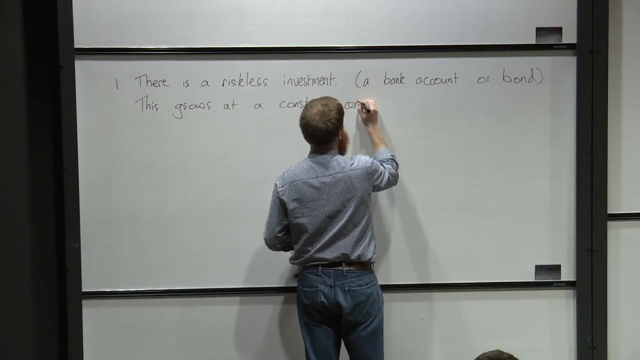 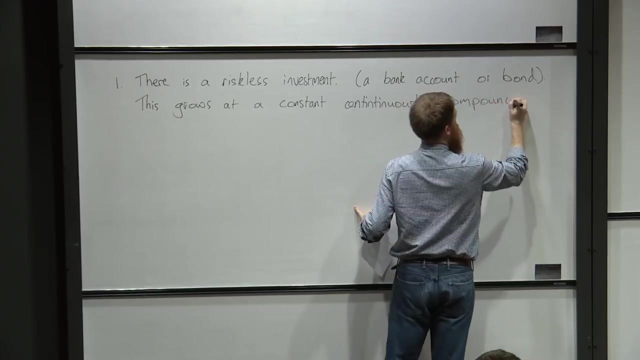 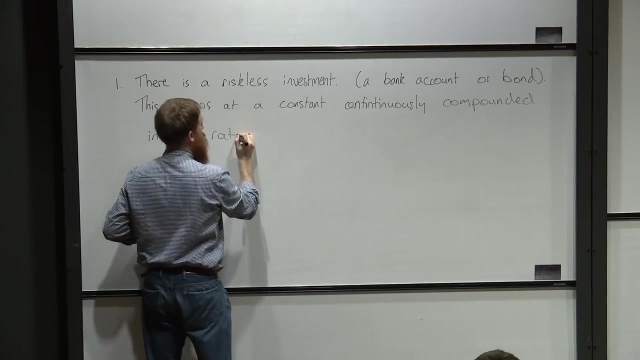 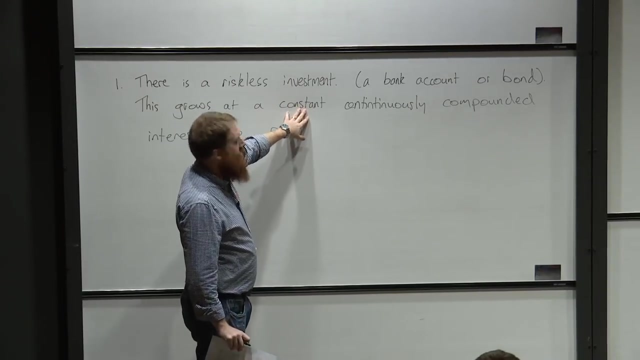 give you money now. to make things simple, this grows at a constant, continuously compounded interest rate, which will denote by a lowercase r. Now the fact it's constant just simplifies things a lot. We'll come back to whether this is a good assumption at various points. 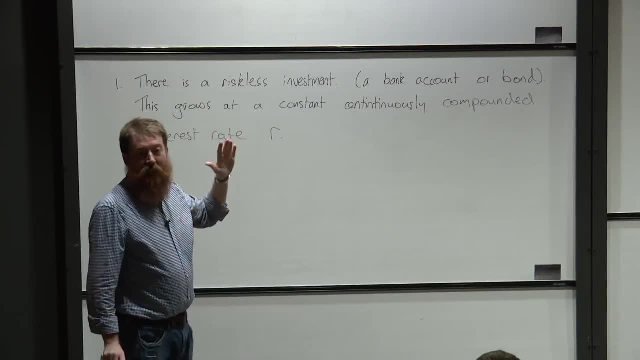 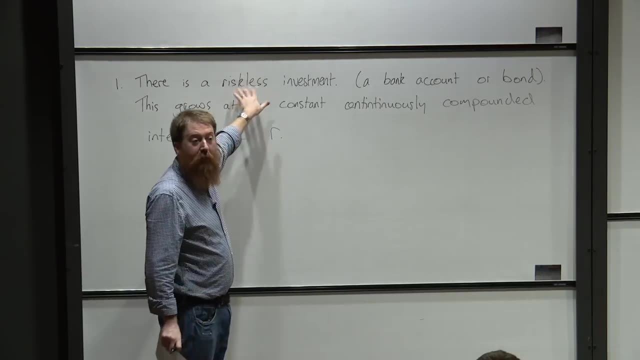 The continuous compounding. that's more of just a technical simplification. The fact that something's compounding continuously means that I can figure out the value of my riskless investment at any point in time, without worrying about when exactly the interest is being determined. 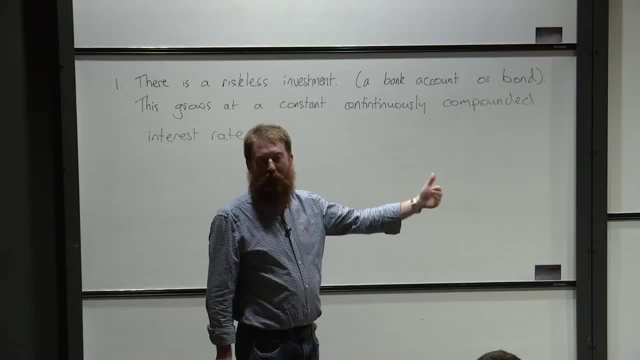 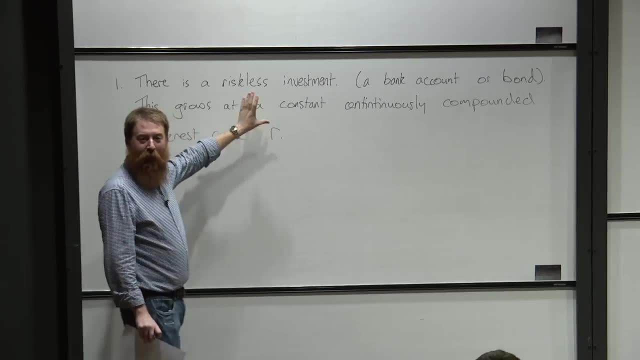 Now, in many cases, interest is calculated on a day-to-day basis, so at the end of the day, And what that means is that this is only an approximation. It's the first point where we've already started making bad assumptions, assumptions that are not. 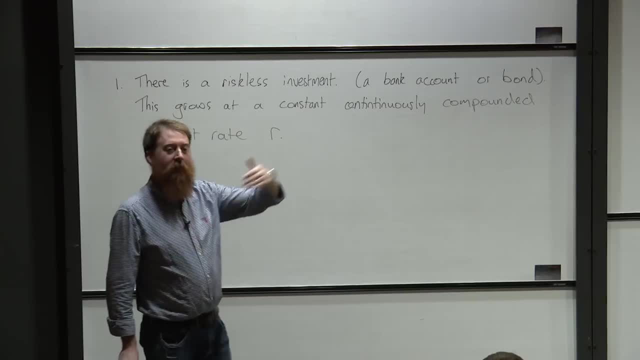 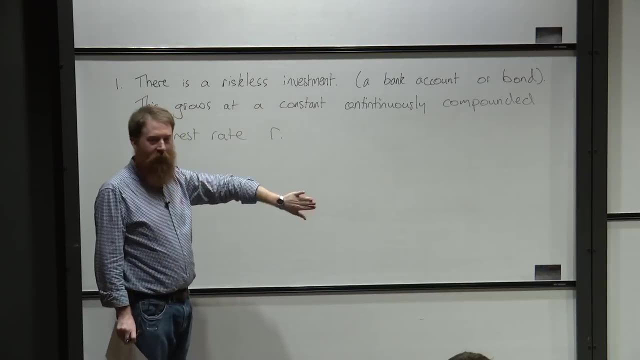 technically true, but they're good enough If I'm pricing something which is a long way in the future, say a few months. the fact that interest is being computed daily rather than continuously makes very, very little difference in most cases. OK. 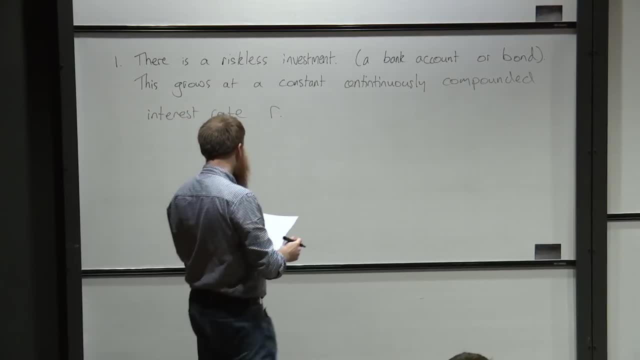 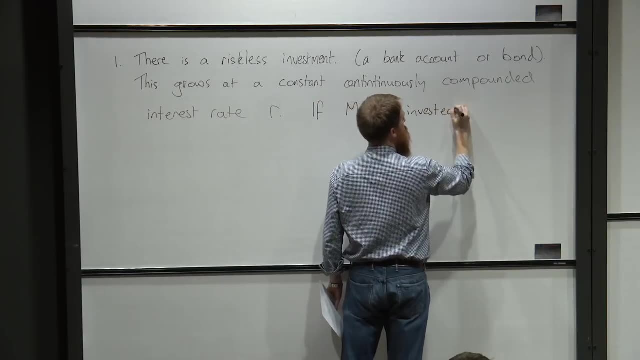 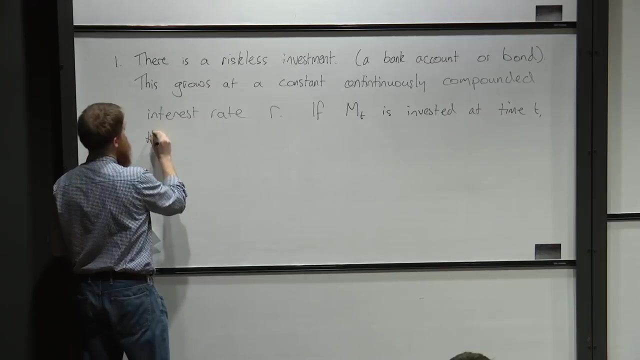 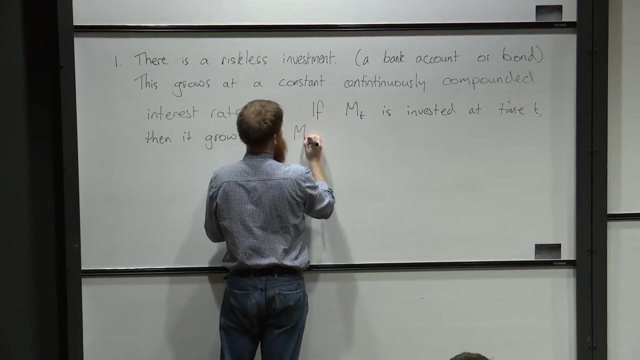 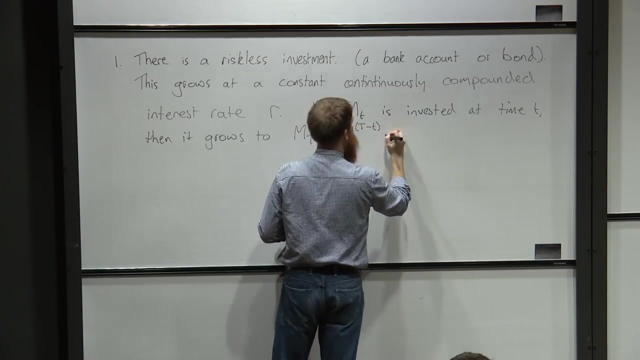 So what is this? Well, it means that if a quantity mt is invested at time t, then it grows to. well, how much m big T, which is e to the r big T minus this Little t mt at time t. 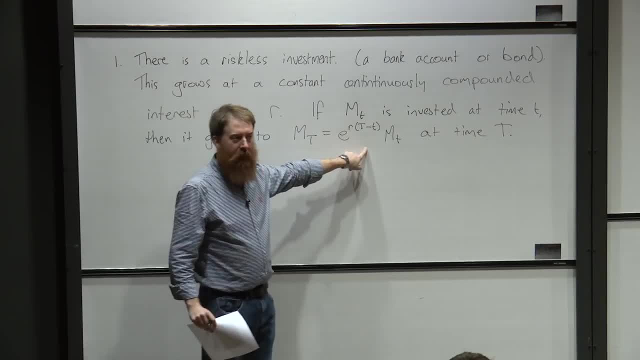 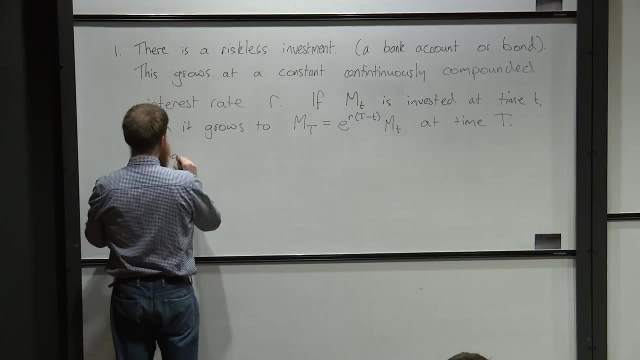 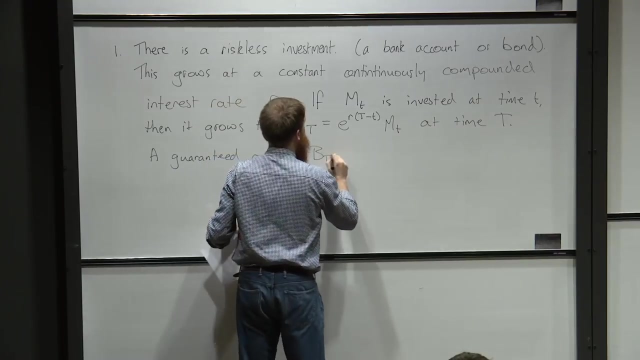 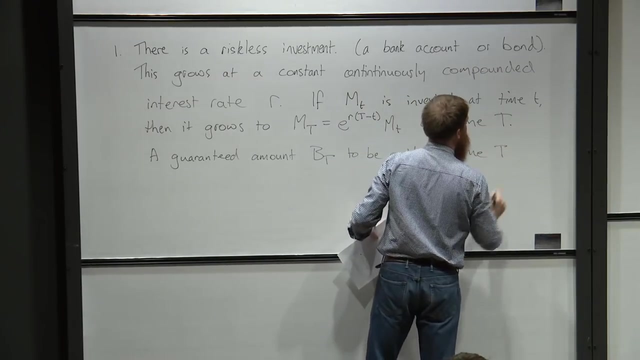 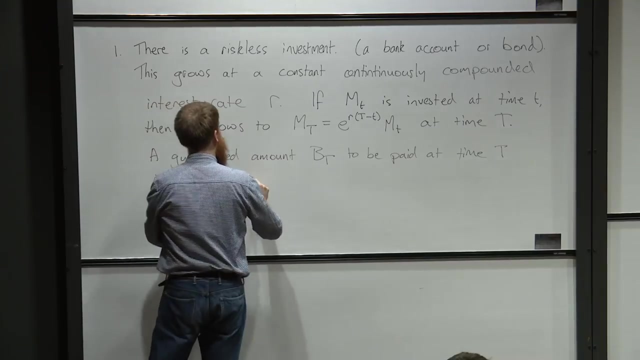 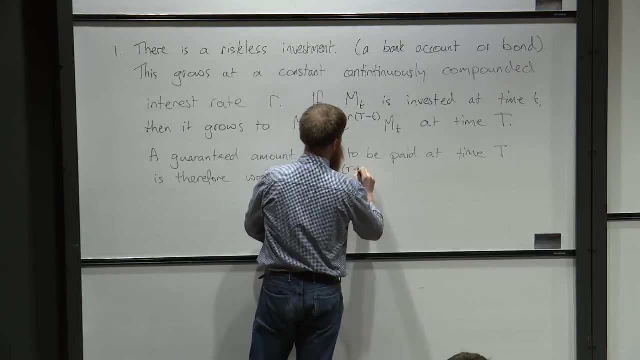 And so this is this continuous compounding. You get an exponential coming in, OK, A guaranteed amount, bt, to be paid at time t, OK, That's it. So you can see that the time t is therefore worth b little t, which is e to the minus r t. 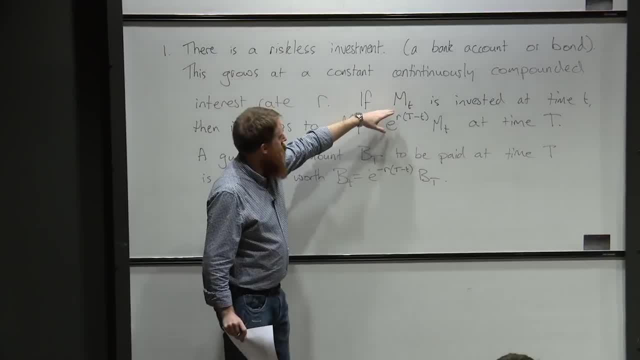 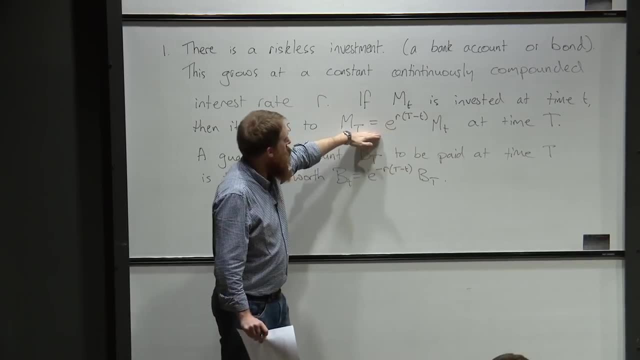 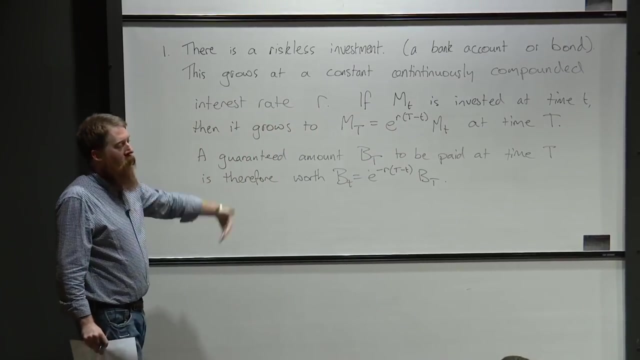 So if this is true, if I can invest at time, little t. so today I invest into the future and my amount that I've invested grows by multiplying by this coefficient e to the r, big T minus little t, the time duration. Well, that means, if I want to get 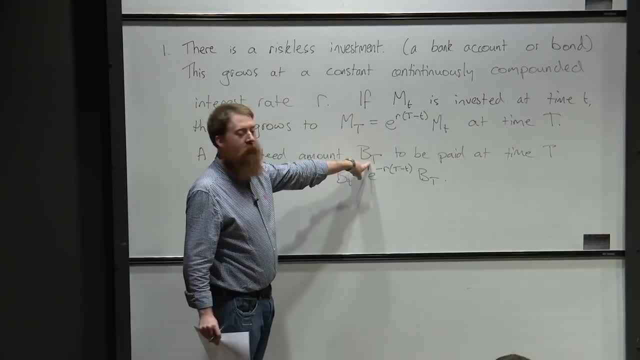 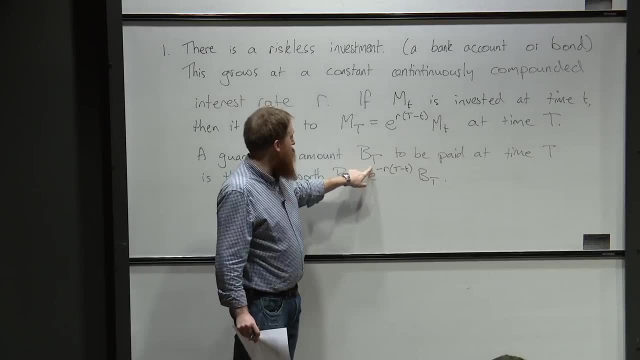 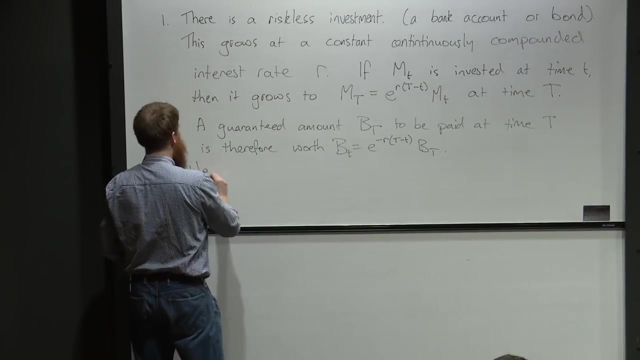 a contract which will pay me in the future a fixed amount, b big T. then how much do I have to invest today? Well, you rearrange this formula and you get it, but with a negative exponent, We assume. So it's not a big deal if I get this now, and I'm still. 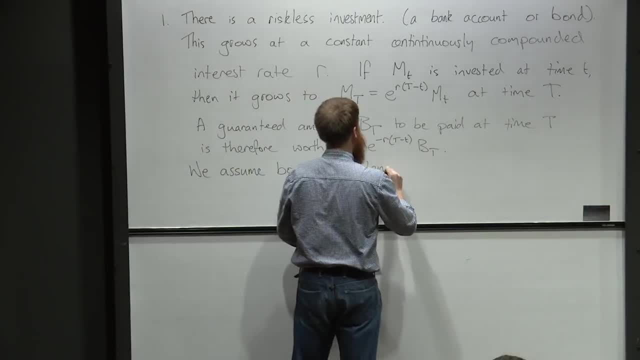 having a great amount of money. I'm having a nice normal life, But at the end of the day, I want it to be good in terms of true, And so the two assumptions are correct, But I want it to be clear that my current borrowing and lending 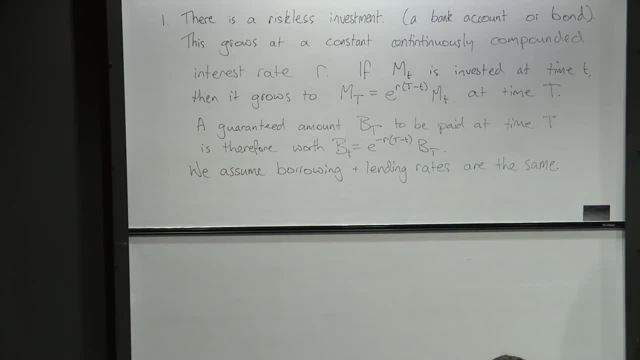 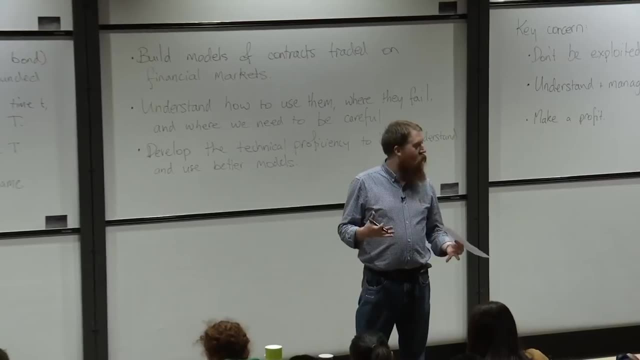 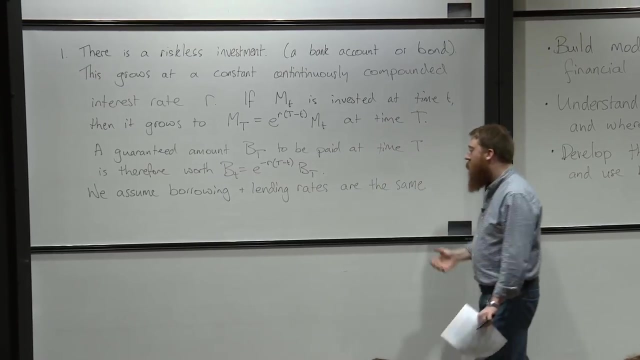 rates are the same. Well, there's an assumption that's clearly not true, But if you're a big financial institution, it gets close to being true that the amount that you're paying to borrow and to lend is very similar, And so we're just going to assume that they're the same. 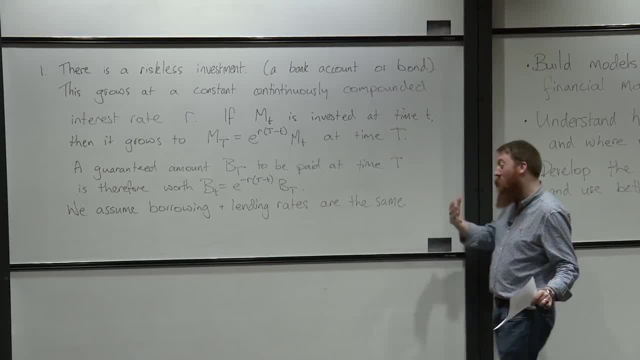 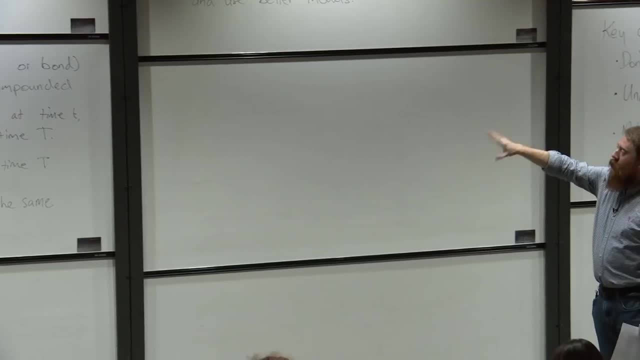 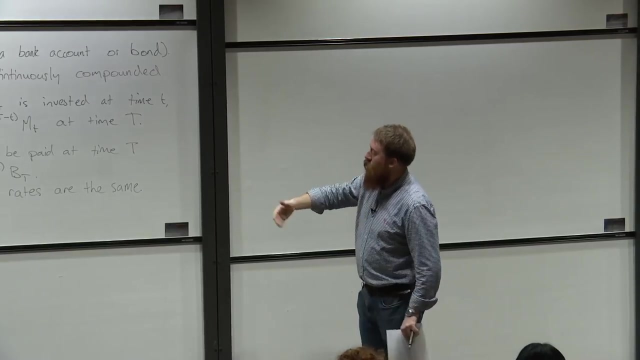 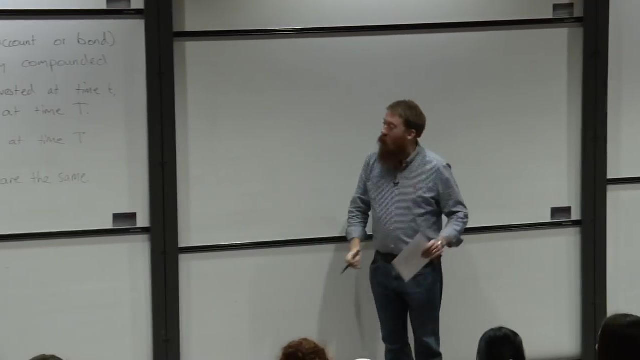 but we are going to remember. that's an assumption which we know is sketchy. okay, so this is the first thing that we've got. we've got this riskless investment in the world where we can invest now for the future, and it's going to grow at a fixed rate that we know beforehand. okay, what are the? 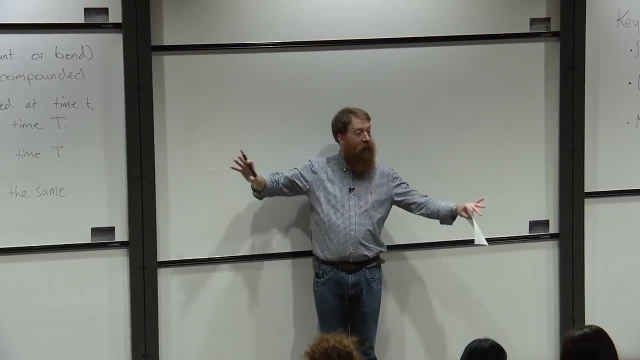 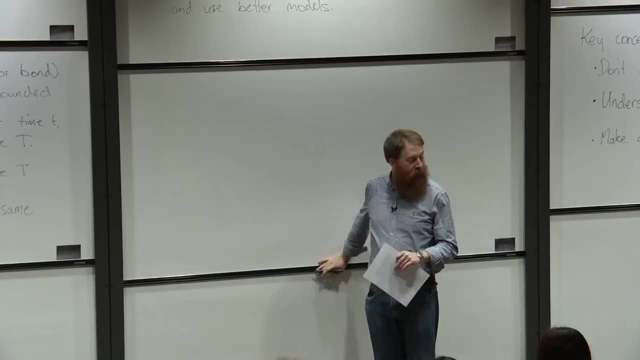 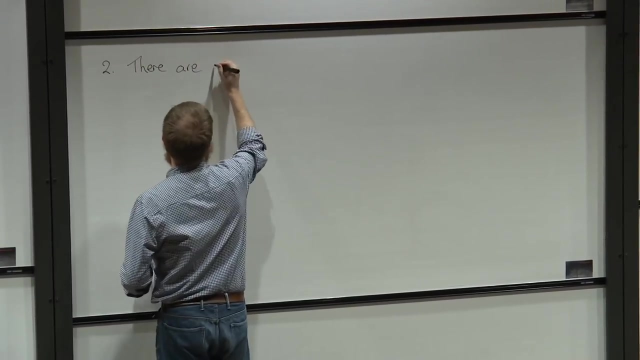 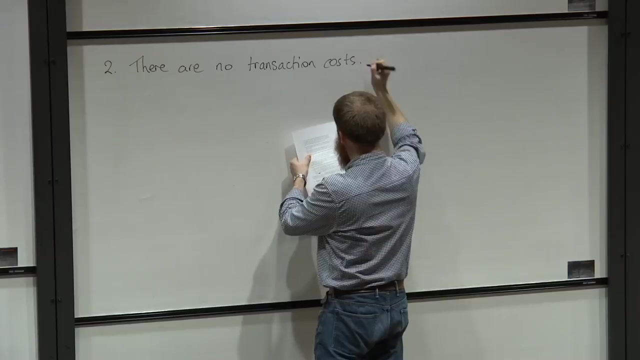 assumptions about the market, because so far we've said nothing about a market. we've just said there is an investment. so we're going to make two assumptions which are sort of our basic modeling assumptions about financial markets. so there are no transaction costs. so what does that mean it? 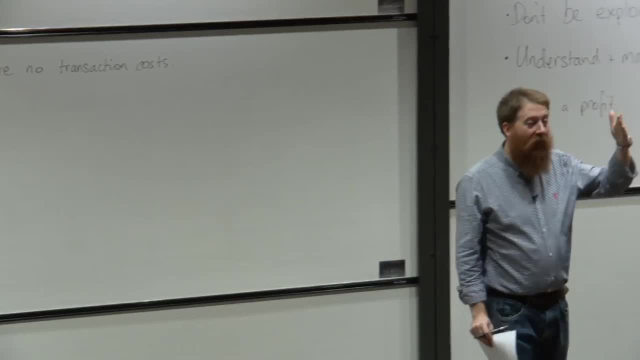 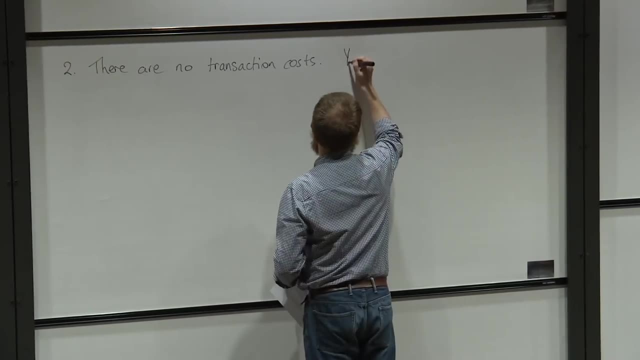 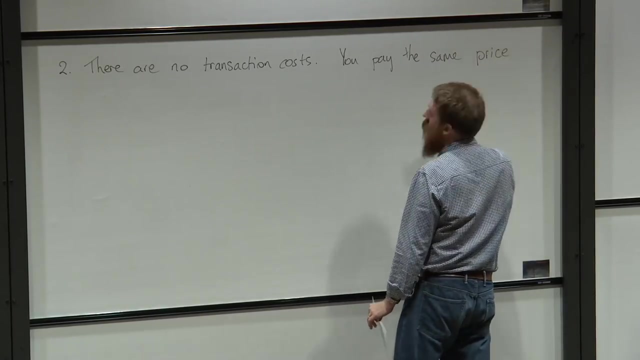 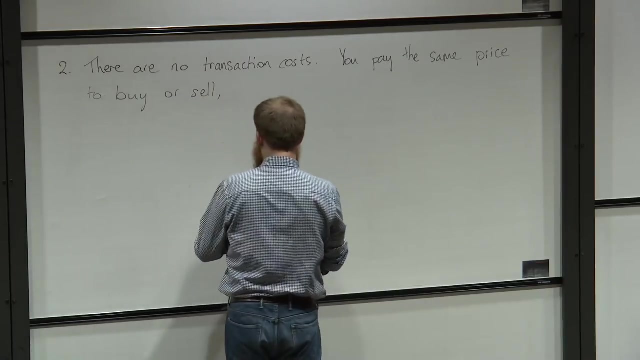 means that if you want to buy something or if you want to sell it, you're going to pay the same price as you're going to pay the same price as you're going to pay the same price as you're going to make either side of the trade. so you pay the same price. you pay the same price to buy or sell, okay. 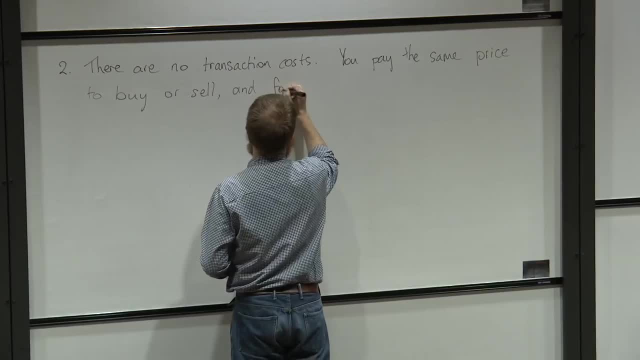 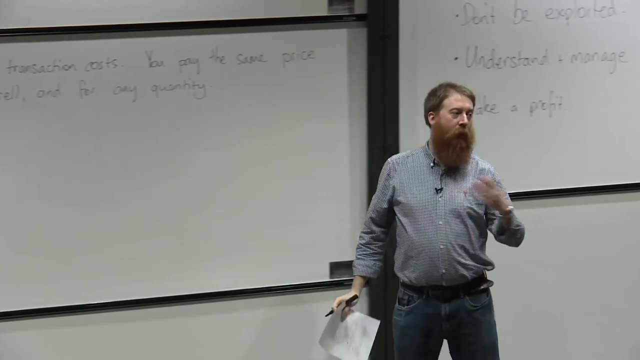 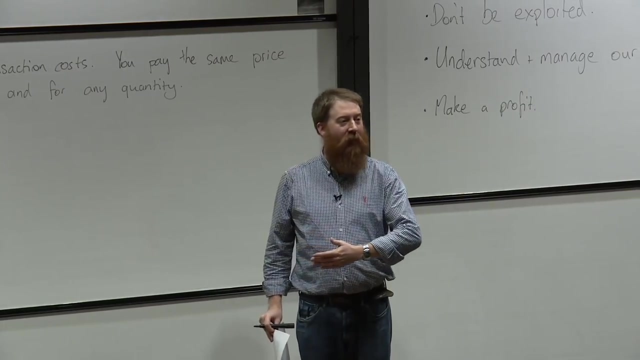 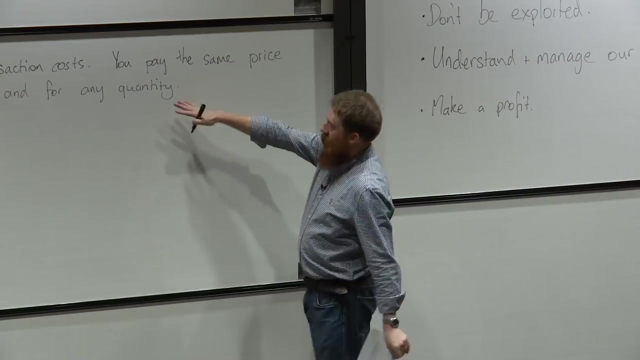 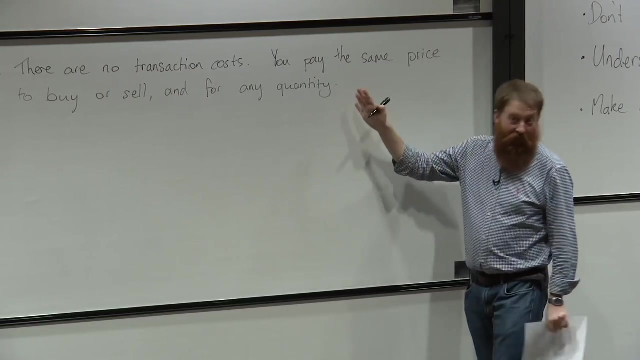 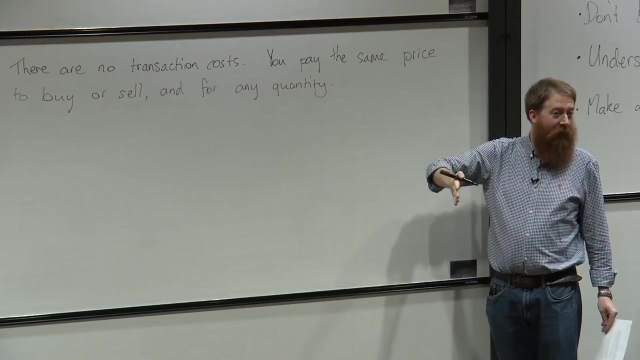 and for any quantity. so the price that you would pay and for any quantity. so the price that you would pay for buying one. брос the ugly, form and then be. i'll go back to that forces. okay, what now? you would probably want to pay for the, because there are certain bits. so, um, let's. 'm only talking about these two- fits right, and there might be some of theری for that. so let's look at today's statement, which is to say it's going to be a reasonableılanーン, And if I said I'd like to sell you 1,000 TVs. 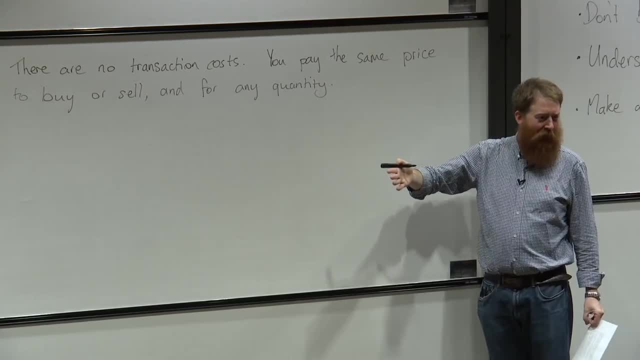 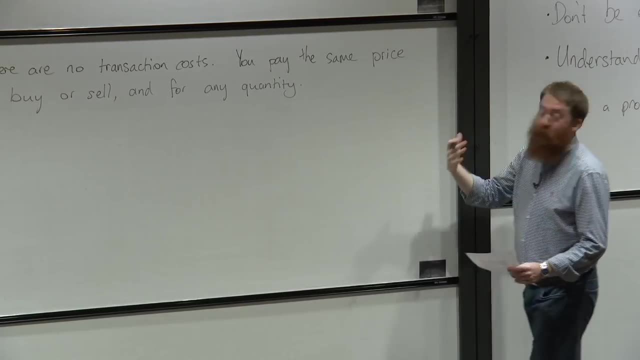 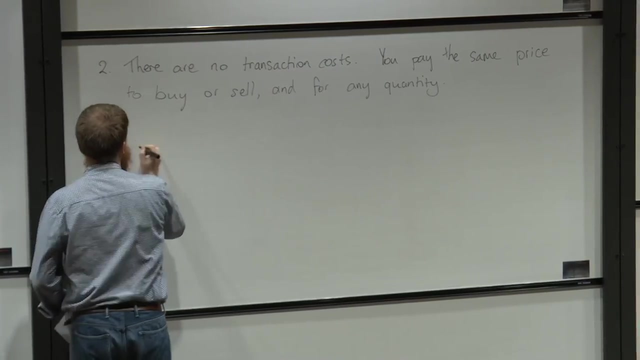 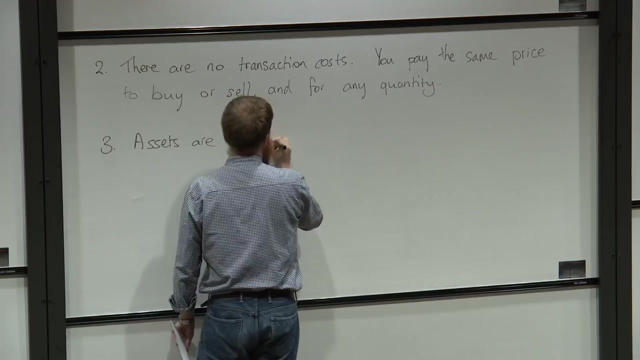 you'd look at me strangely and ask: where have I gotten 1,000 TVs from and why am I trying to sell them? So the quantity effects are important, but we're just going to ignore them as a first approximation. OK, a related assumption is that assets are infinitely. 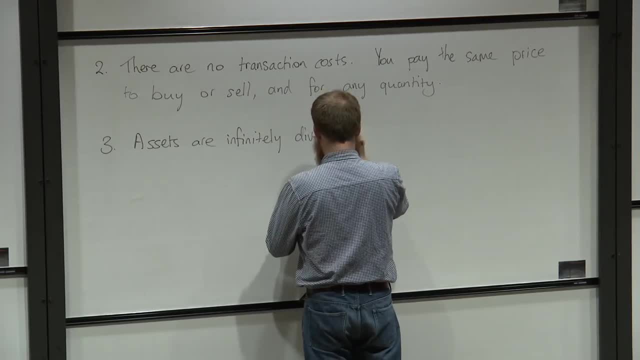 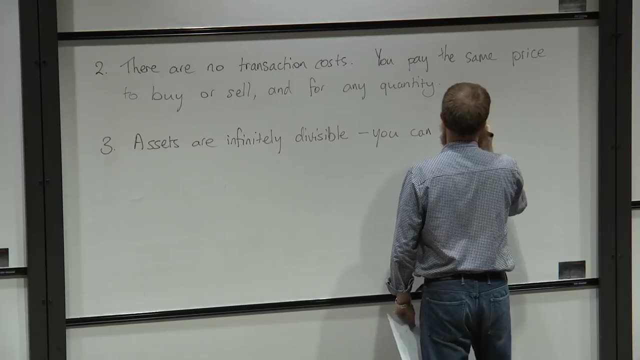 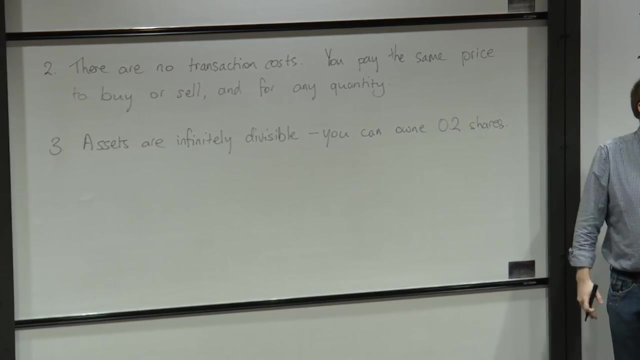 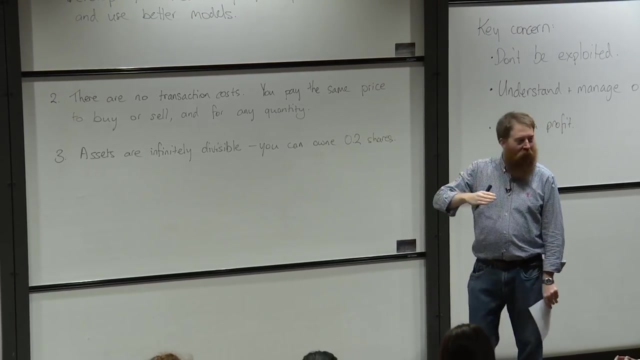 divisible. OK, you can own 0.2 shares. This is more a technical assumption than anything else. It means that we don't have to worry about discrete numbers of shares, that you've got to buy one share or two shares. You can't buy 1 and 1 half shares. 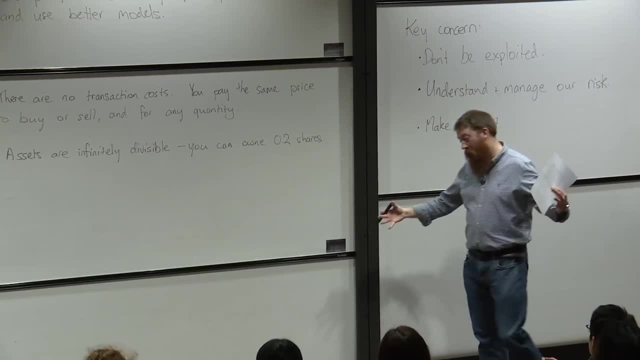 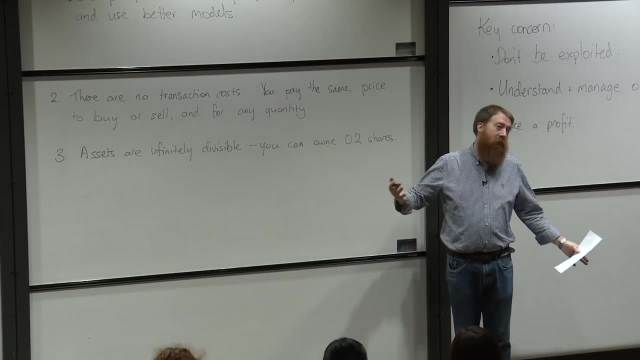 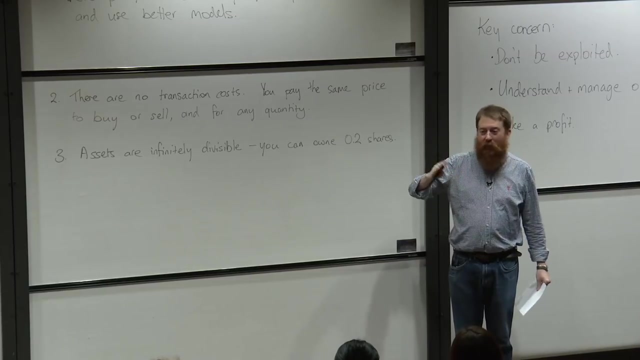 Practically it doesn't matter, Because once you're working on a large scale, if you're working on a deal for 10,000 shares, the difference between buying 8,000 and 8,001 shares is pretty small. It's a discretization error, but it's small enough. 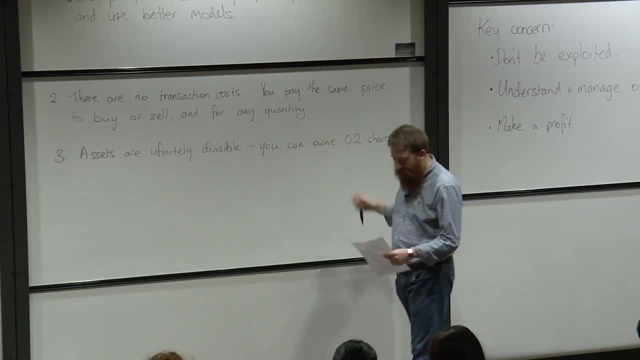 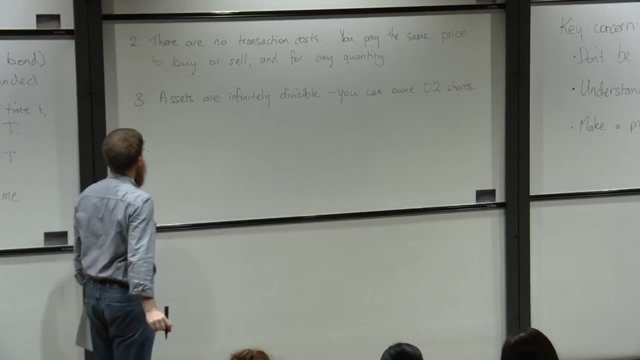 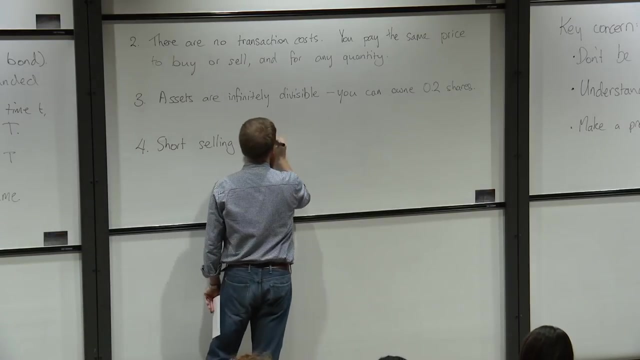 that we don't need to worry about that as a first approximation. OK, something a bit more controversial than those is that we're usually going to build models where short selling or long selling is allowed. OK, a little bit of terminology whenever I say short. 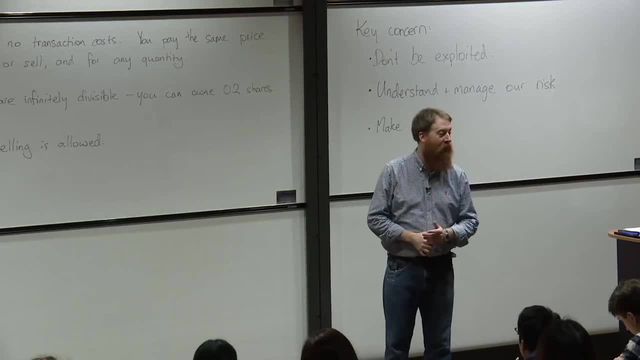 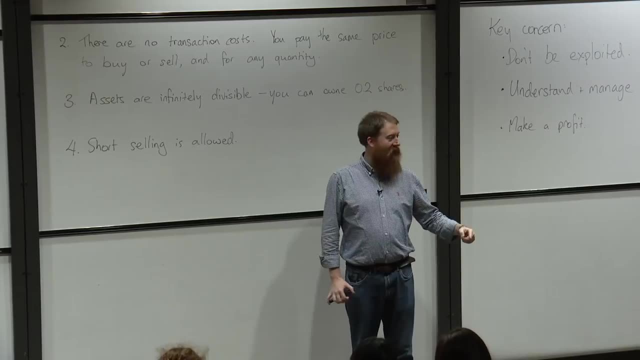 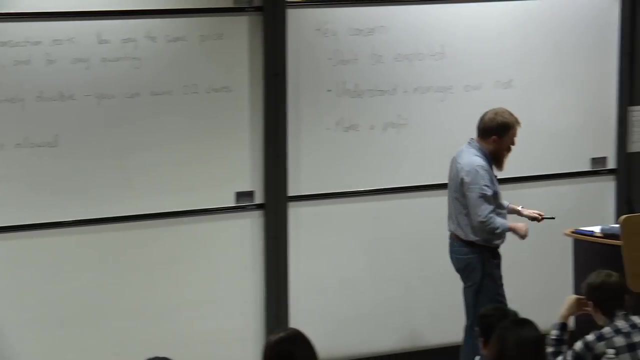 I mean selling something. Whenever I say long, I mean owning something. So what's a short sale? That's where I own a negative quantity of an asset. Now, is this possible? Well, it depends on what you mean. Now, it's certainly true that in many markets, what you can do 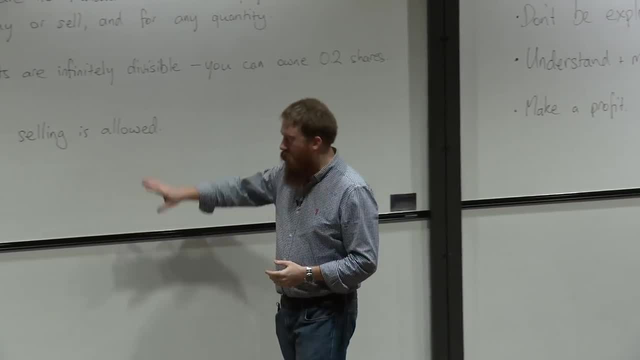 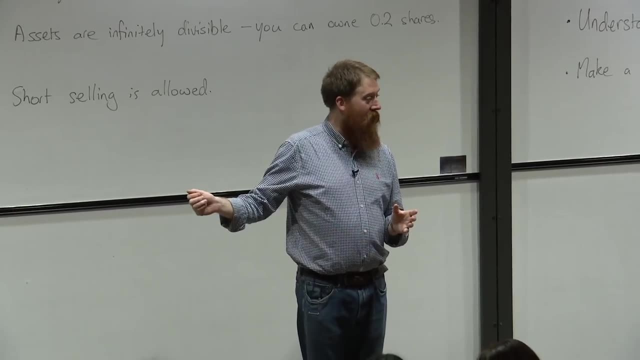 say, in the equity market for big stocks. if I want to hold a negative amount of some big stock, what can I do? I can go and I can borrow that stock from someone else. I pay a fee. We'll ignore the fee. 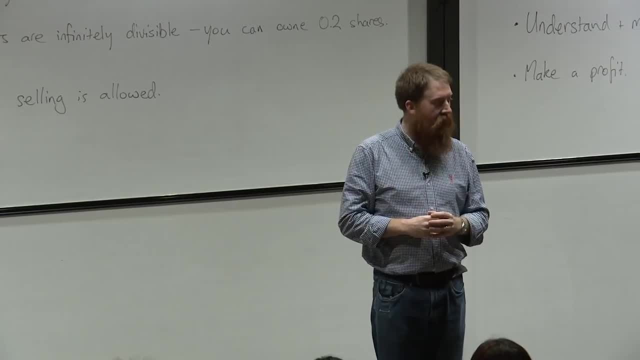 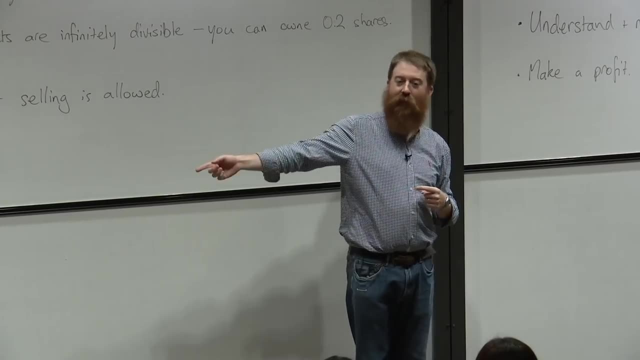 But I pay a fee to borrow the stock. I then hold the stock. I can sell the stock. Now what that means is I have an obligation in the future to buy the stock again and return it to the person I borrowed it from. But in the meantime I hold a negative quantity of stock. Why is that? If the stock goes up in price, I lose. If the stock goes down, I win, because I'm going to have to buy it in the future. Now that is what's called a covered short sale. 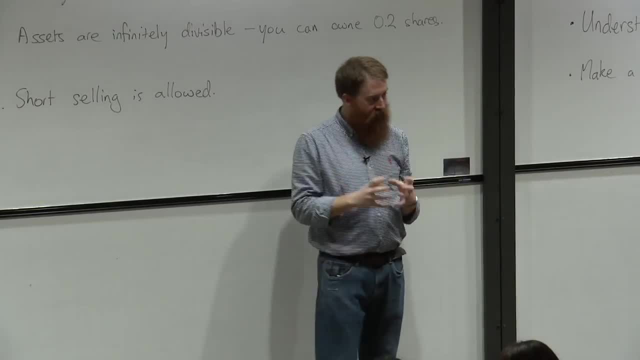 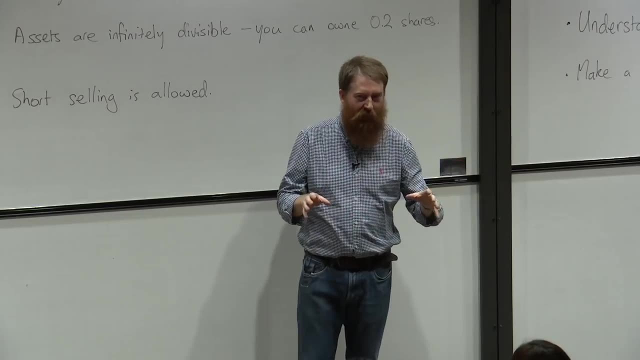 I have gone, I have borrowed the stock from someone, so the stock is physically there and I'm able to sell it on. When I say physically, I mean I'm able to sell it on, I don't mean physically. Pretty much everything's done electronically these days. 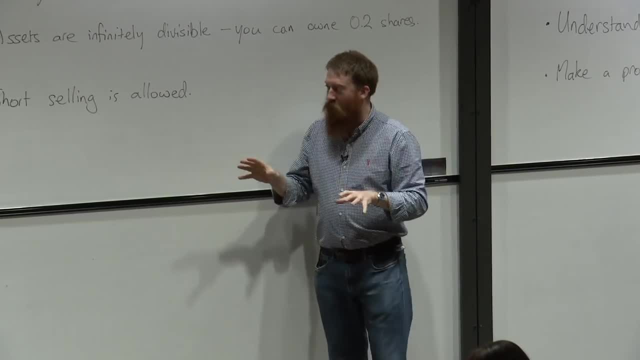 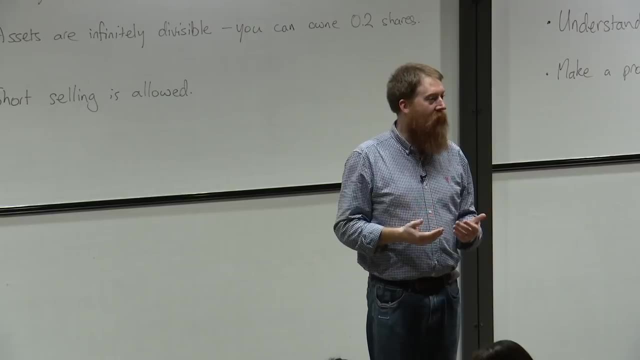 but don't let that worry you. There is also what's called a naked short sale. A naked short sale is basically where I go into the market and say I'll sell you some stocks And you say, all right, I'll buy them. 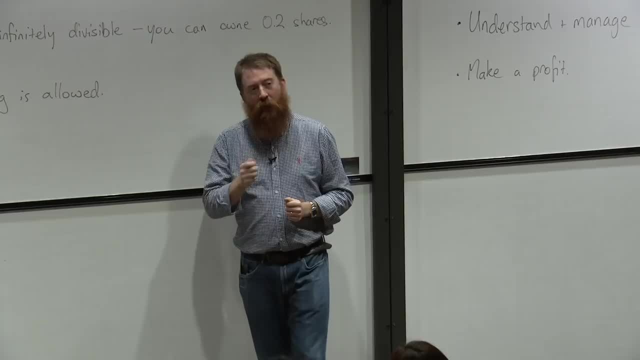 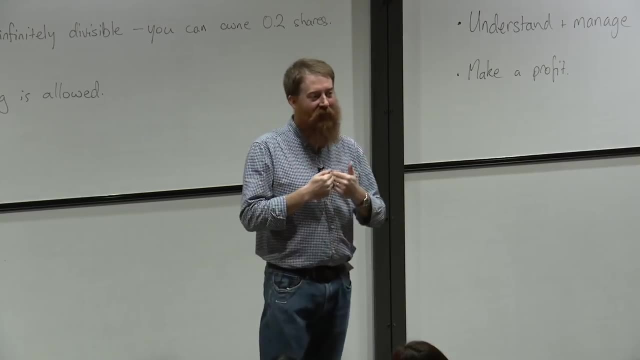 And I go great. And I know that the contract gives me two days to make good on the deal. So if you've bought stock from me, I know that I have two days in which I, in two days' time, well, by two days' time. 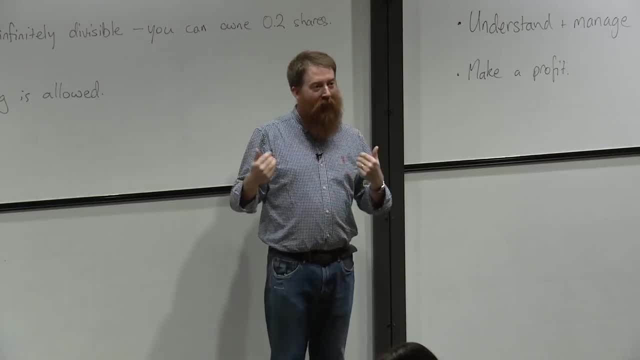 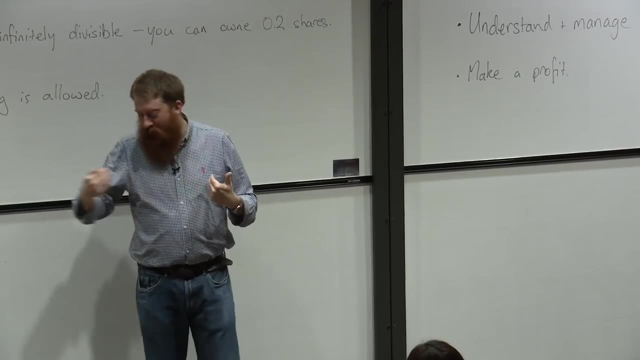 I have to deliver the stock. So I am now currently short the stock because the stock goes up in value. I'm in trouble. But there's the idea that I could go and if I do this, if I make a naked short sale, I say I'm going to sell it. 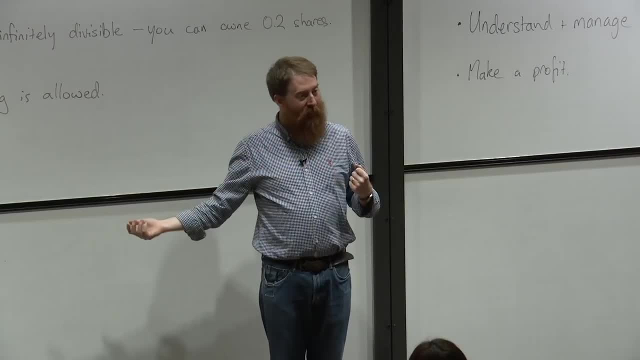 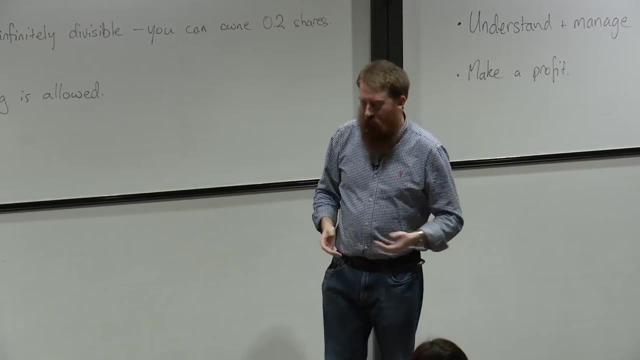 I could then go and buy it in the market or borrow it from someone after I've made the deal. This is a naked short sale. This has been very controversial in the past few years. Why is it? Because, if I haven't already identified the stock, 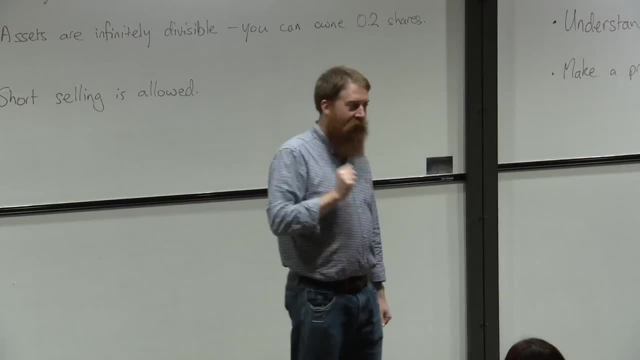 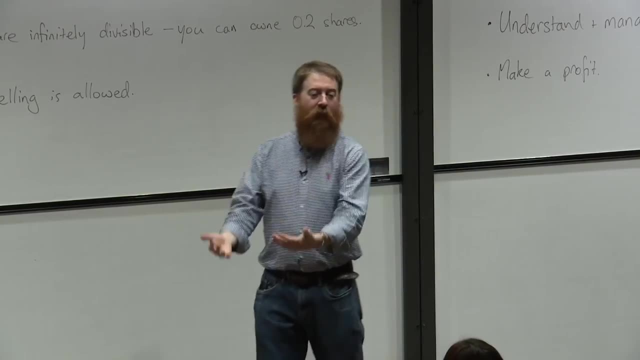 that I'm going to be borrowing or if I haven't already borrowed it. it's very easy for me to start selling things I don't own. It's very easy, if I'm allowed to do that, for me to go and say: 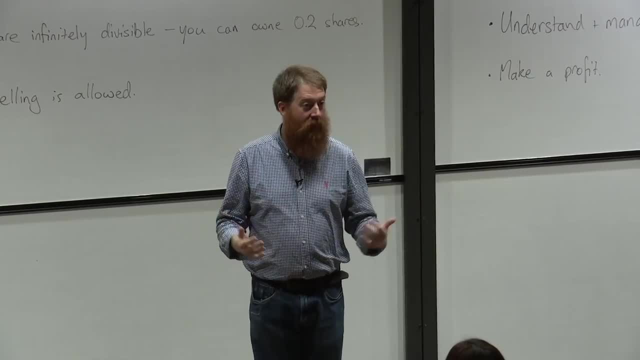 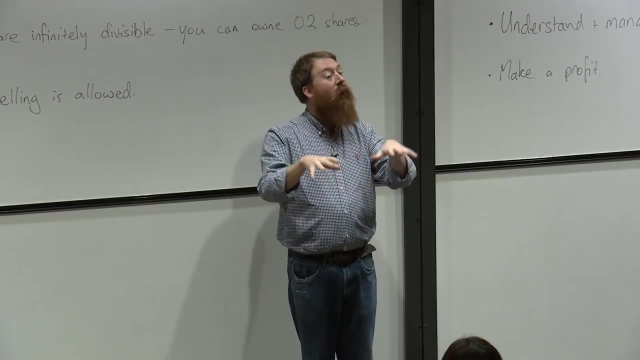 I'm going to sell 10,000, 10 million, however many stocks I want, And that looks like lots of people are trying to sell a lot of stock even though I don't own it, And so that's been linked to the idea. 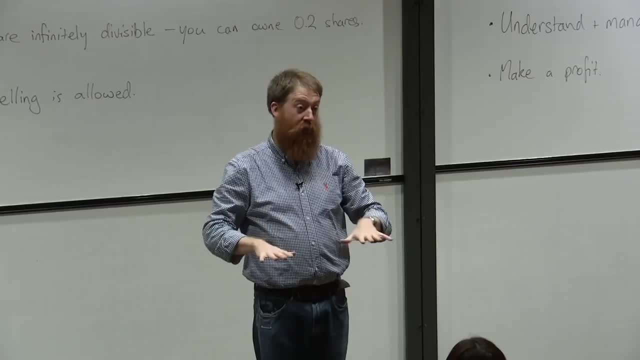 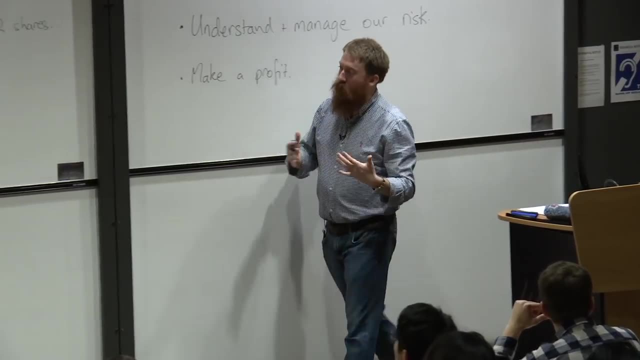 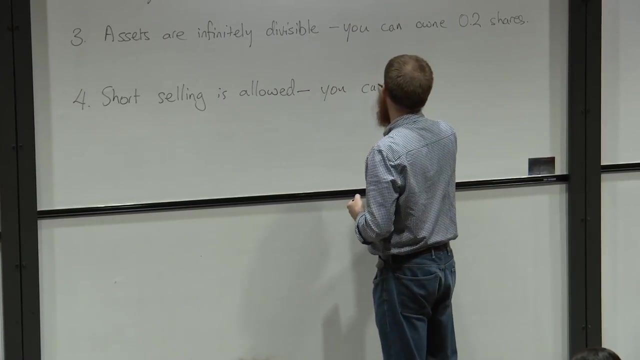 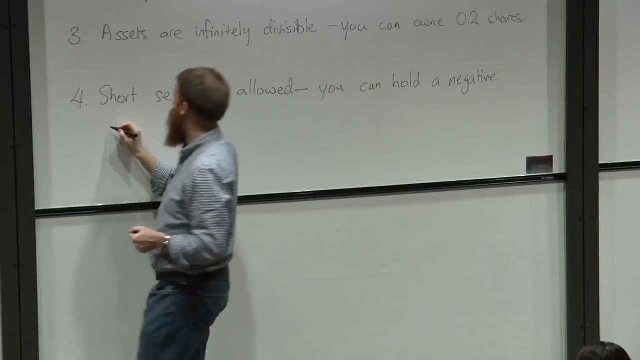 that it's going to push prices down, and so it's been quite controversial. We're going to assume that it's allowed. We're not going to go into the details of how short selling is actually manipulated, but we're just going to say you can hold a negative quantity of. 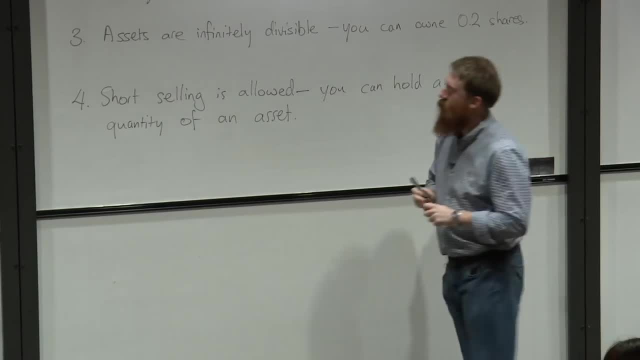 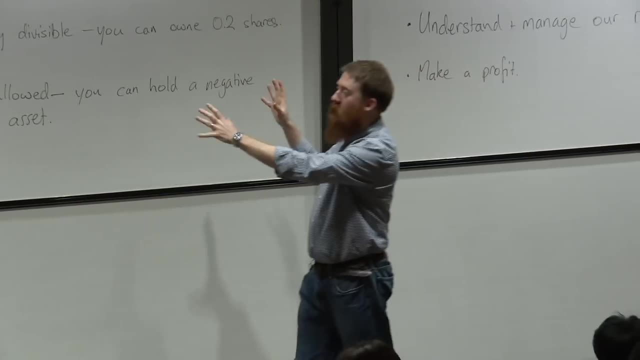 say $1,000, $1,000, $1,000,, $1,000, $1,000, $1,000.. And then we're going to say, OK, so this is the basic assumption of how we are going to model markets. 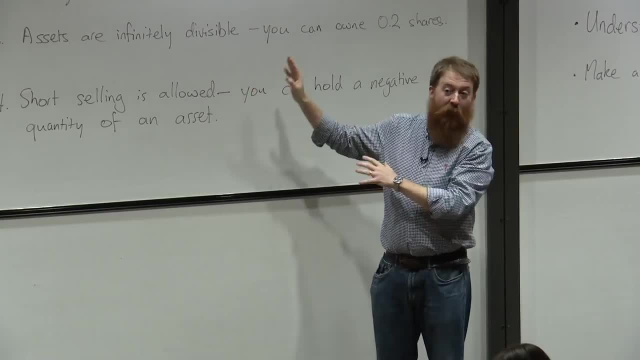 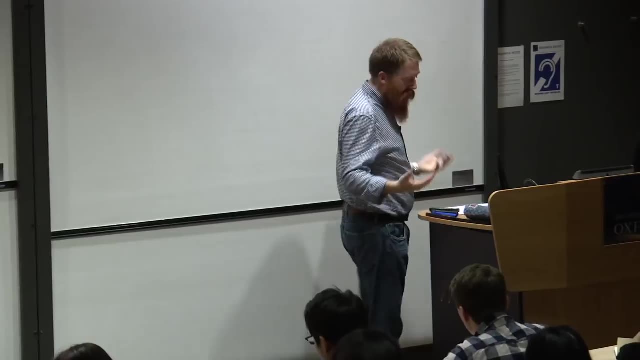 unless I say otherwise, we're going to take these as given, even though we know that most of them are sort of not true. But this is true in most mathematical modeling. We have to abstract, we approximate and we hope that we've captured the key features of what 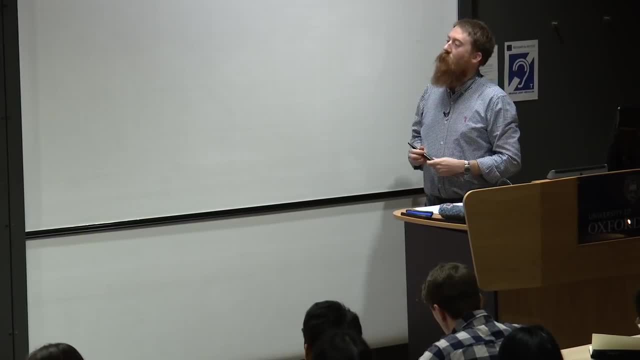 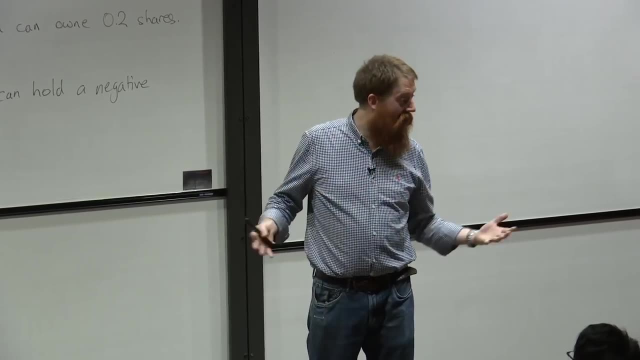 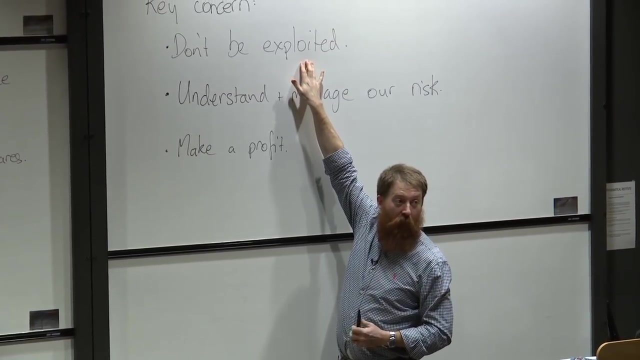 we're trying to understand. OK, So how do we proceed? Well, we haven't yet given any principles which will allow us to find a price of anything, But we have said one thing earlier here: that we're going to avoid being exploited. 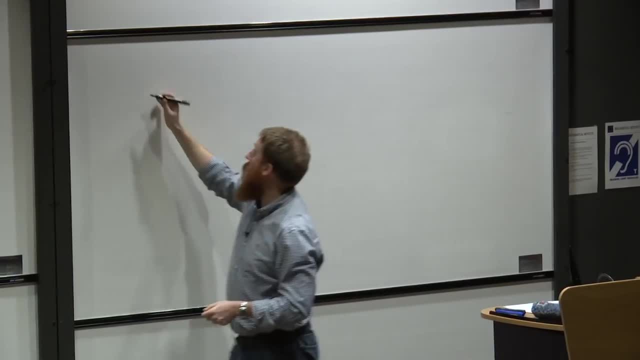 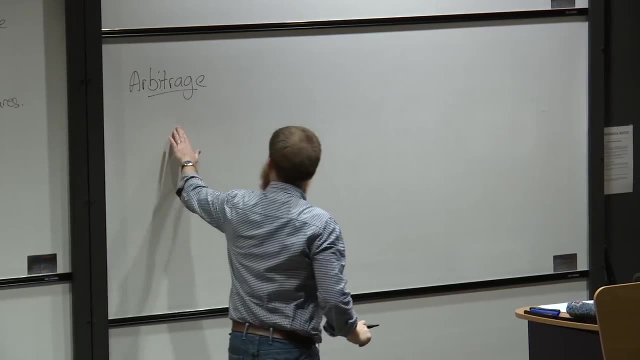 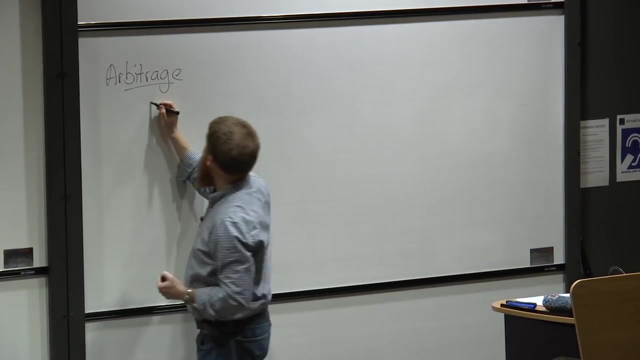 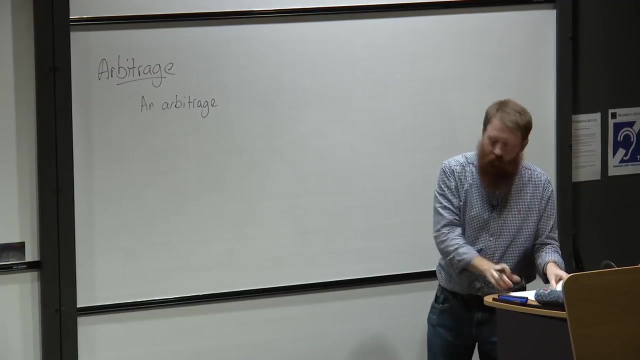 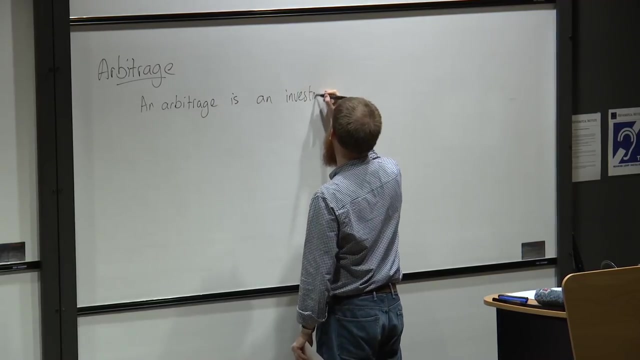 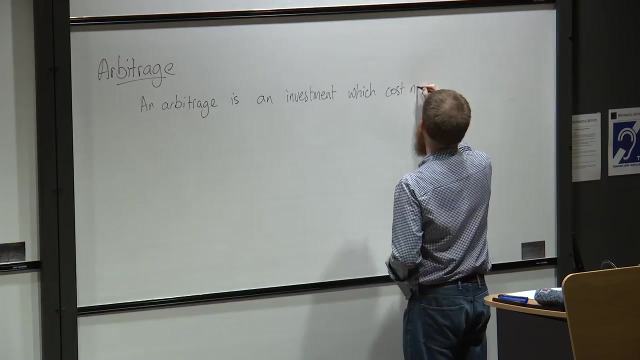 And the most basic form of exploitation is arbitrage. So what's an arbitrage? An arbitrage? An arbitrage is a deal that is too good to be true. So an arbitrage, let's get the definition right. so it is an investment which costs nothing. 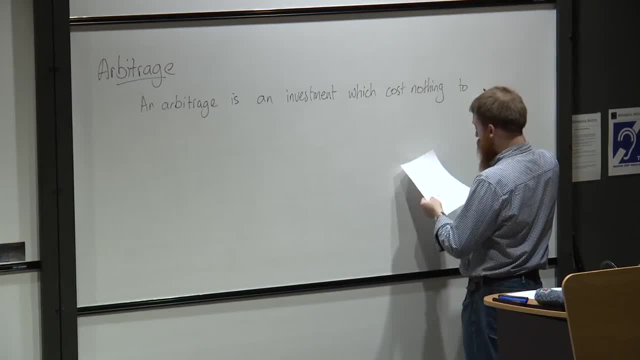 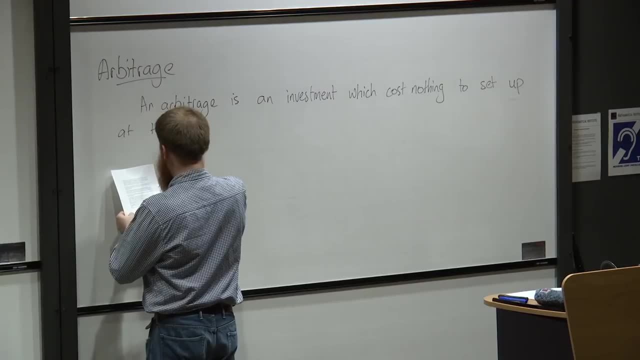 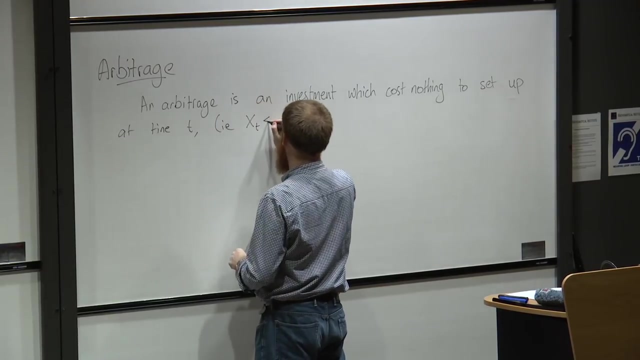 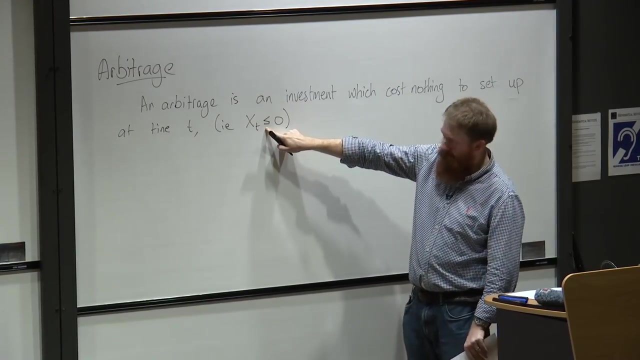 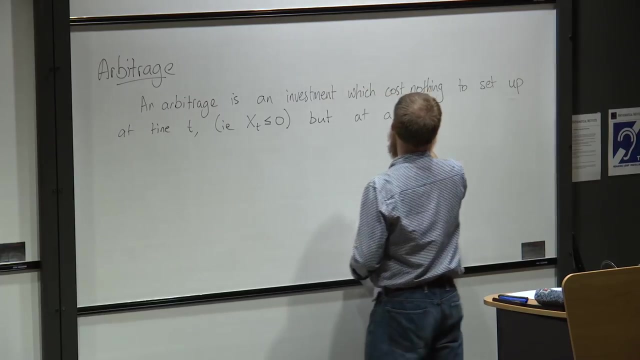 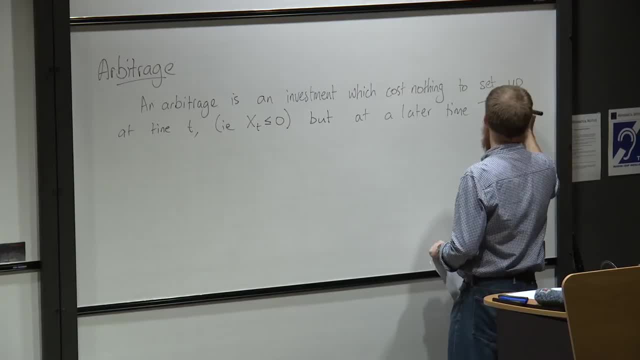 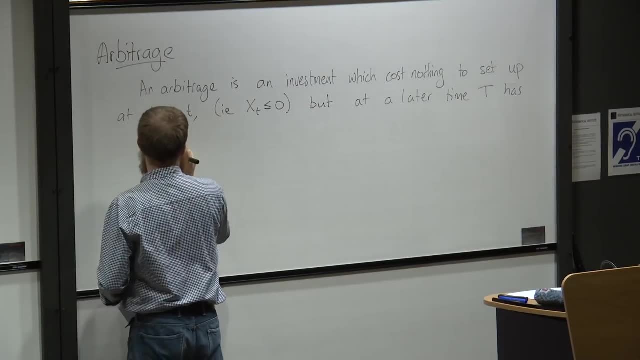 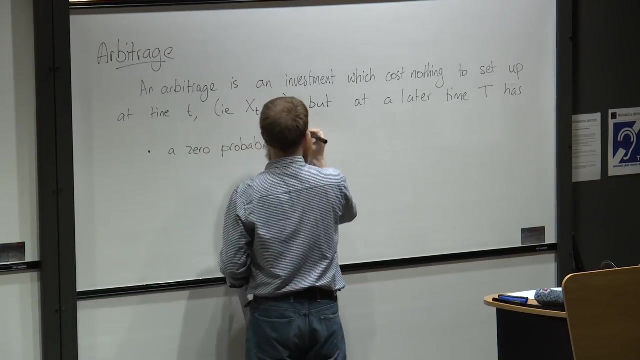 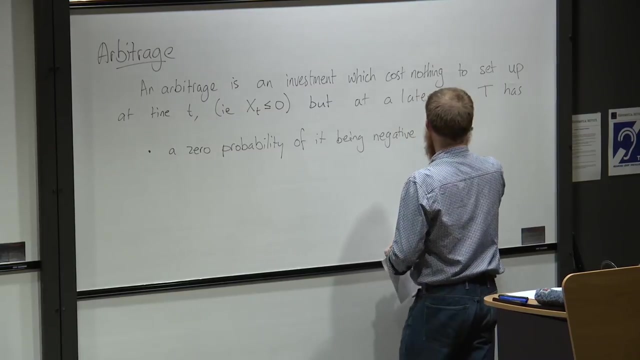 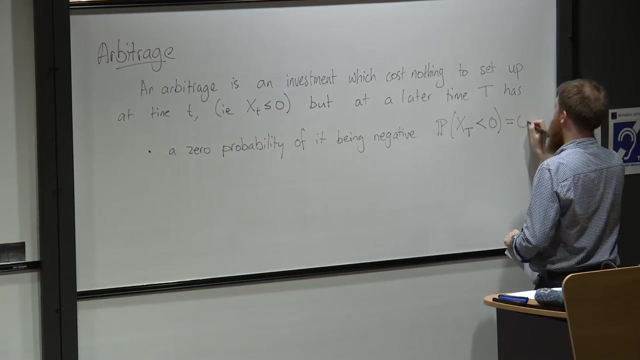 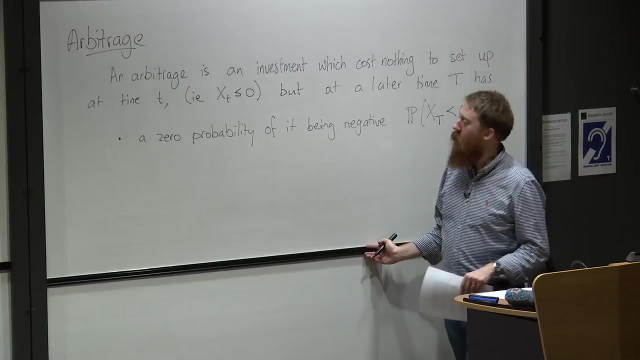 At a later time. big T, we have a zero probability of it being negative. so the probability that X at big T is less than zero is zero because if it was worth a negative amount that would be costly for me in the future, I'd have to pay it. 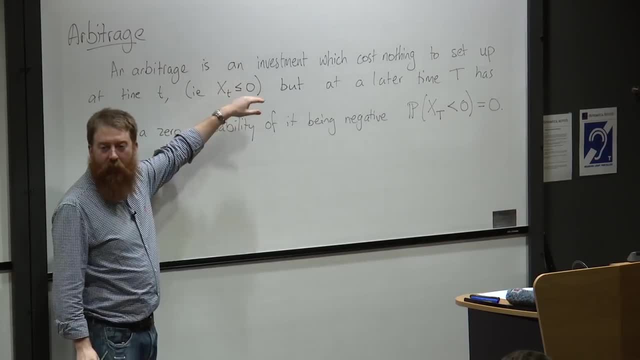 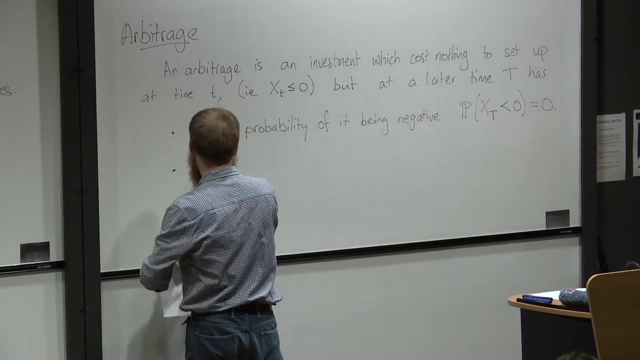 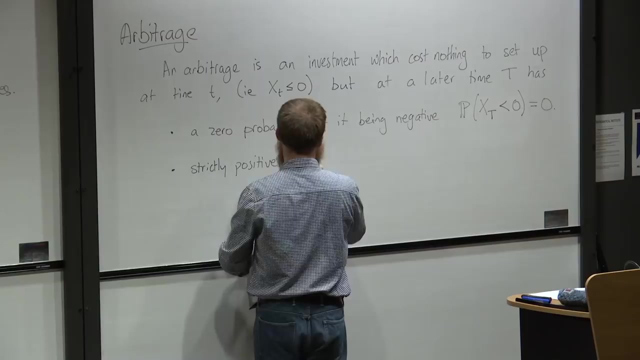 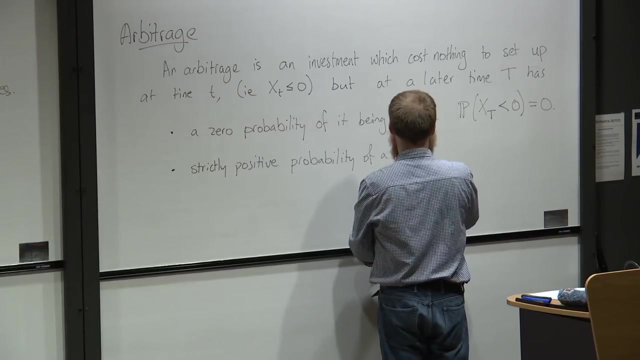 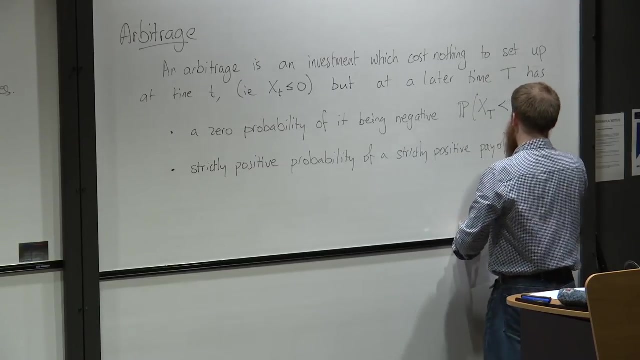 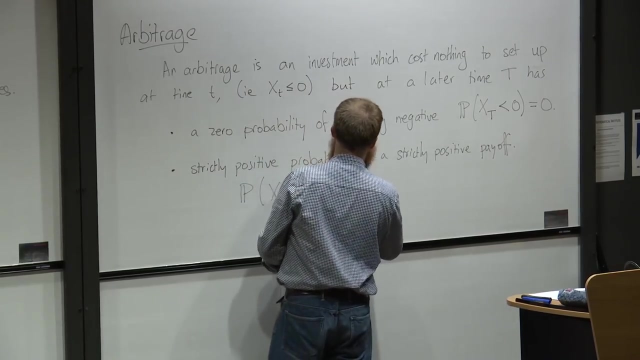 So this is a deal which costs me nothing to set up in the future. I can't lose. the probability of me losing is zero and it has a strictly positive probability. So I mean that the probability that XT is greater than zero should be positive. 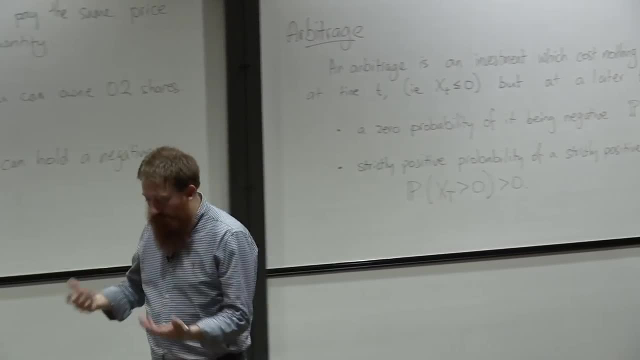 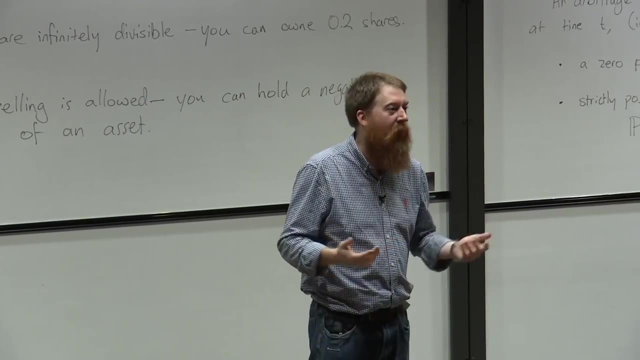 So an arbitrage, if we think of simple games, is something like the game where we flip a coin: if it's heads, I'll give you a pound, if it's the tails, nothing happens. Now, if that doesn't cost you anything to enter into, it's a very good game to play because 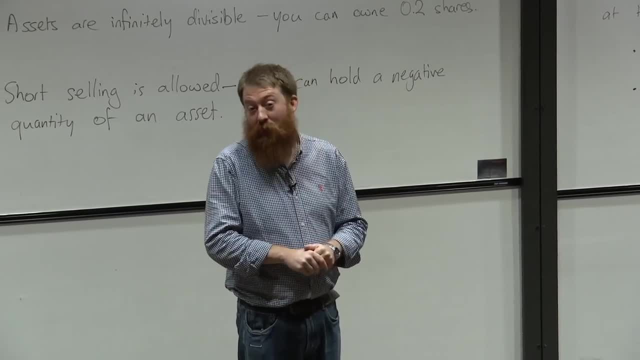 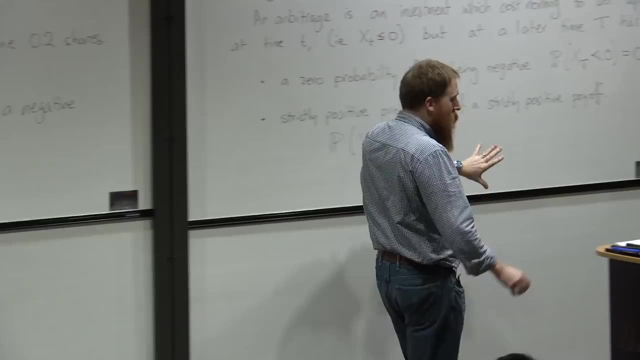 well, maybe you win something, maybe you don't, but you're never going to lose. So that is an arbitrage, and we are going to basically assume that arbitrages shouldn't exist. So the way we're going to build models, 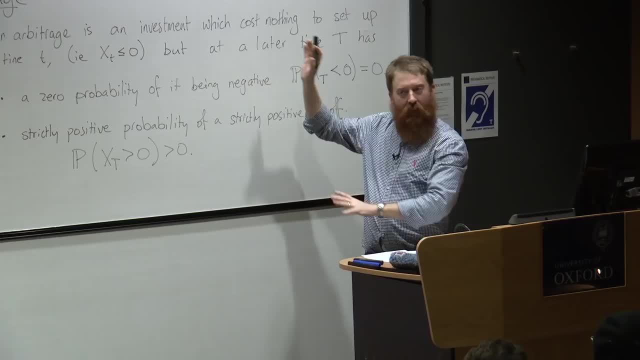 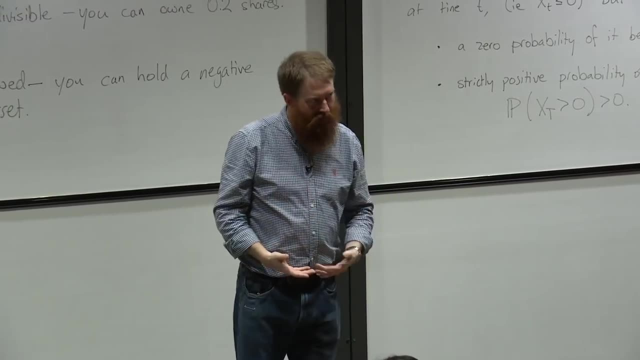 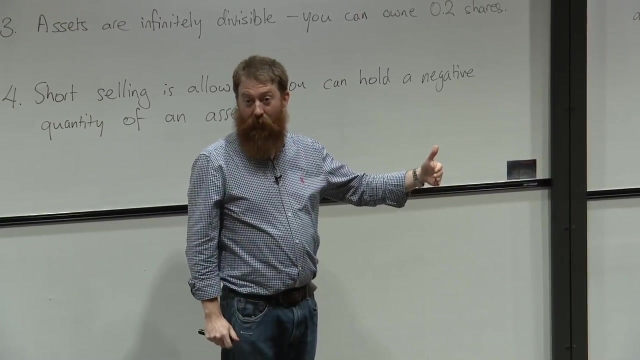 is based on the principle of no arbitrage. Now, does that mean arbitrages actually don't exist? Well, no, they do exist, But on well functioning markets with lots of players. whenever an arbitrage exists, someone will exploit it, And someone will exploit it quickly. And if someone exploits it, they start changing prices. And when they change prices they do so in a way which gets rid of the arbitrage. They sort of eat up all of the money that can be made out of the arbitrage by changing. 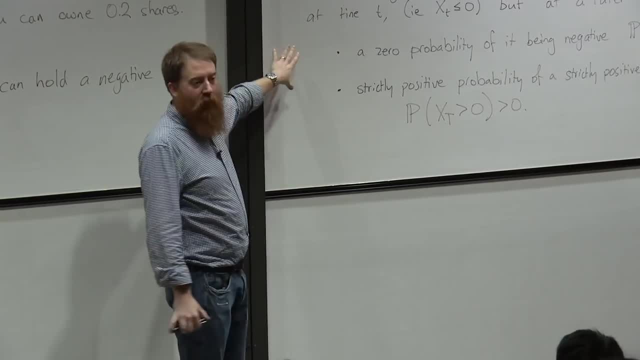 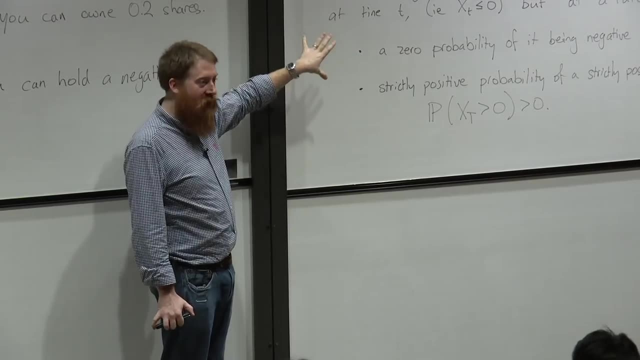 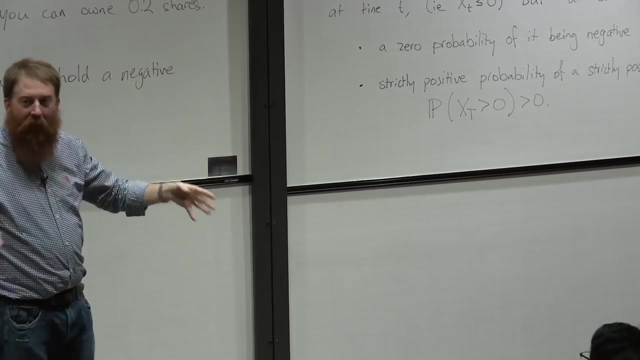 the price. So we're going to assume there are no arbitrages when we build models. What does that mean? It means we're not building a model to try and detect and exploit arbitrage. We're going to be building models which say: let's assume we're not fast enough, we're. 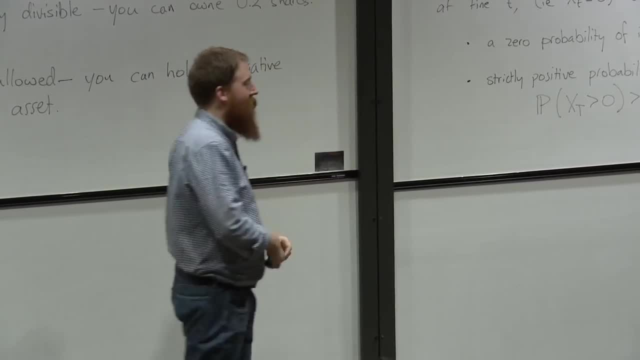 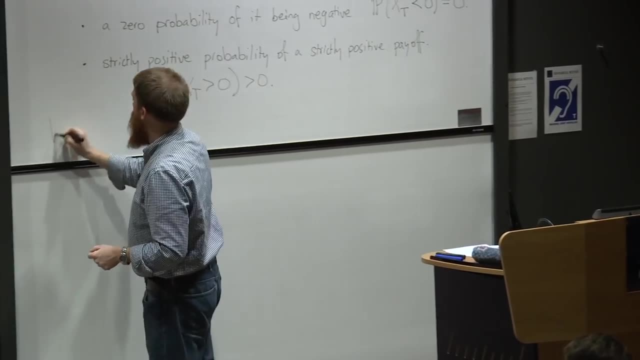 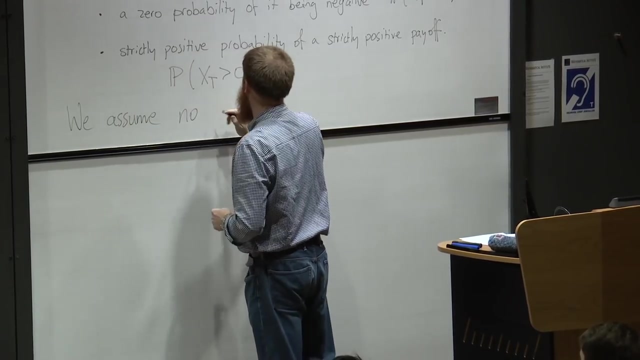 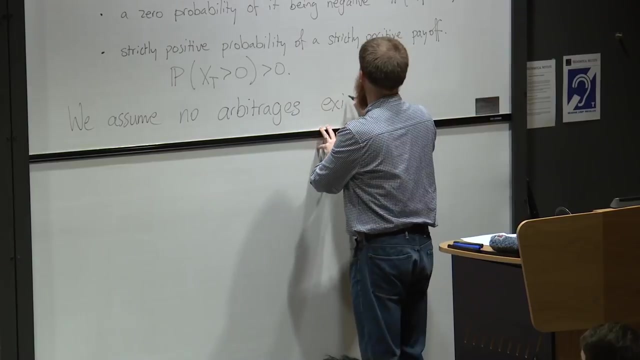 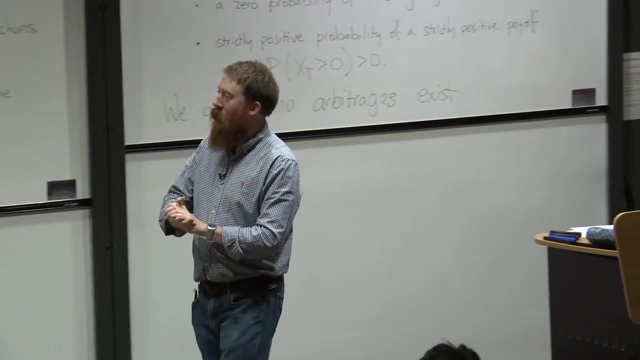 not aiming to exploit this. what can we then say about the market? Okay So, So we assume no arbitrages. no arbitrages exist. Okay So, we've got some basic assumptions about markets and how they work, but we haven't. 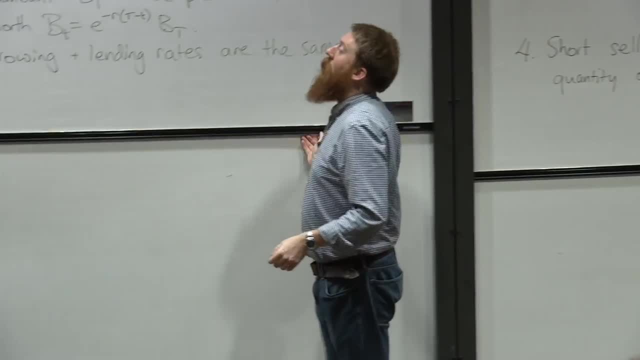 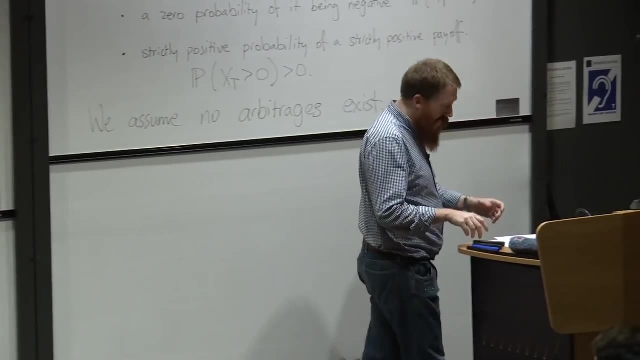 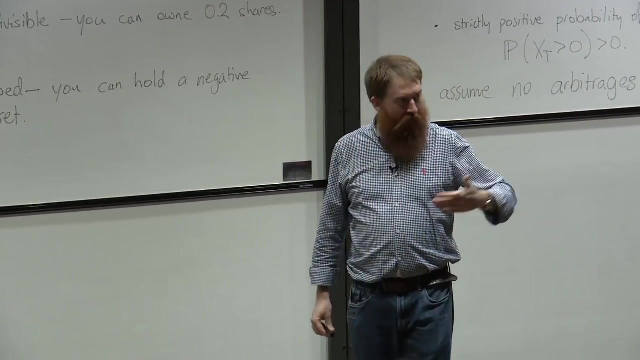 actually considered any contracts yet. So where we'll begin is with probably the oldest form of financial contract. This is what's called a forward, And what it is. I'll give you a simple example. Imagine for a moment that you are an exporter. 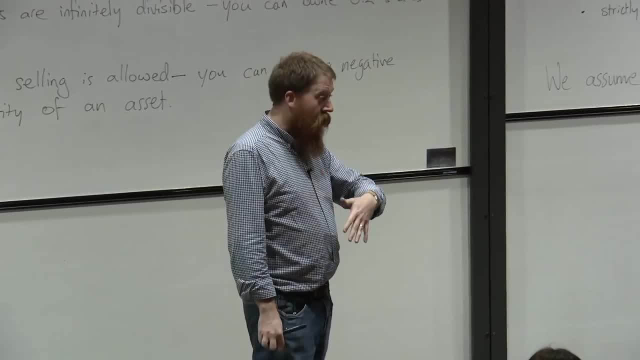 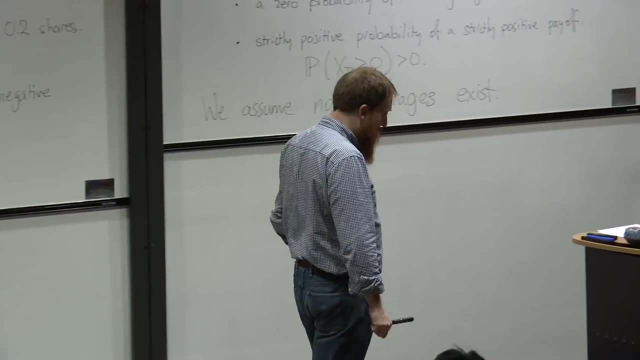 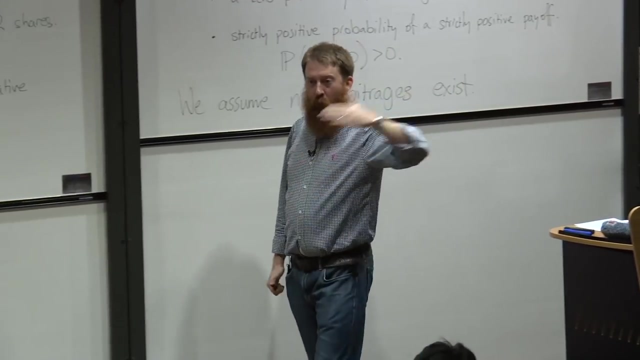 So you are based here in the UK. You are selling things in the US, for example. So in one year's time, Okay, You will make a sale. You've already signed the deal today to make a sale in the US and you will receive some. 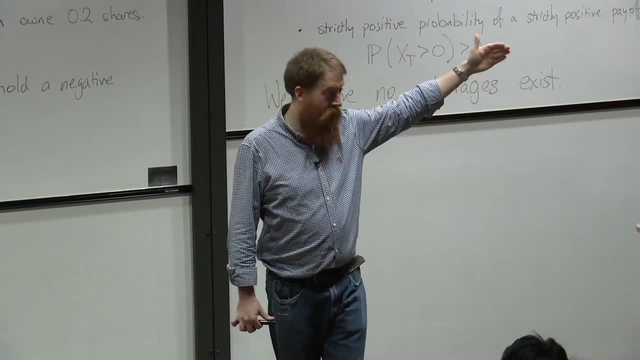 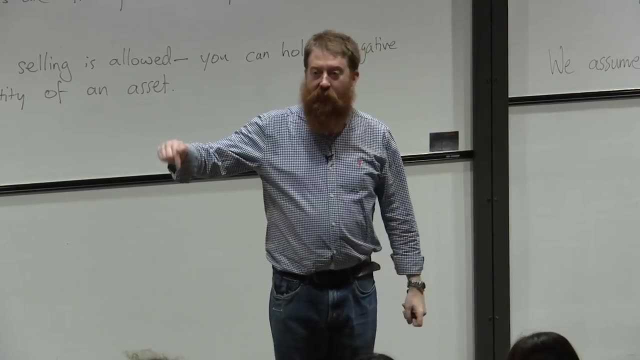 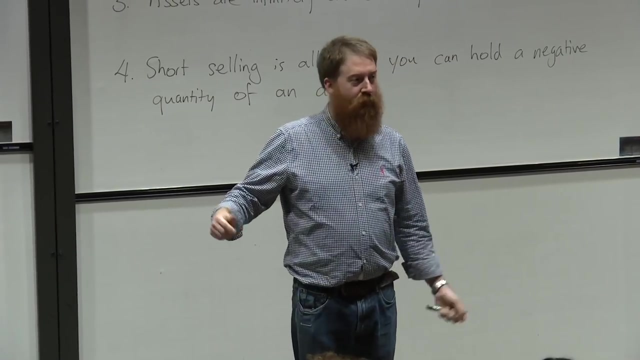 quantity of US dollars. You know that you're going to receive them. On that day, you will have to pay all your costs in the UK. All those costs have to be paid in pound sterling. Okay, You have calculated that, Okay. 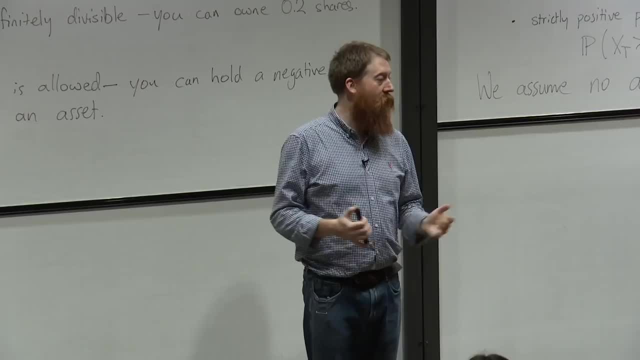 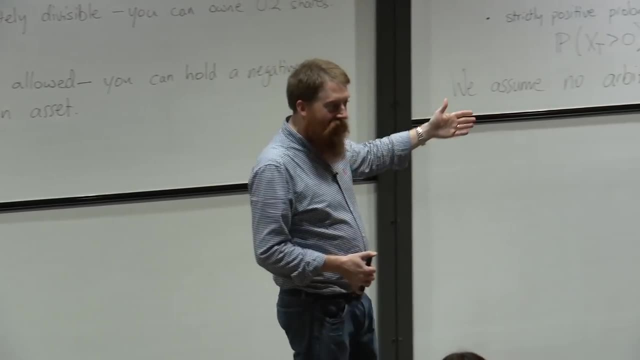 If the exchange rate is as it is today, then this is a good deal. You will make money, But you're worried. You've looked at the last couple of years and the price of pound sterling versus the US dollars has fluctuated quite a lot. And you're worried that in one year's time, when you receive a whole lot of US dollars but have a whole lot of expenses in pounds, that you won't have the money to cover it and you might lose, even though you think today this is a good deal. 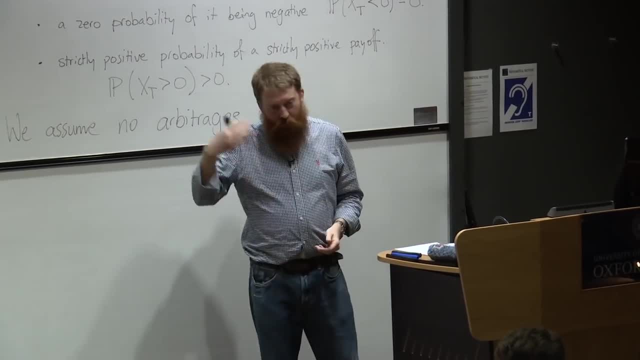 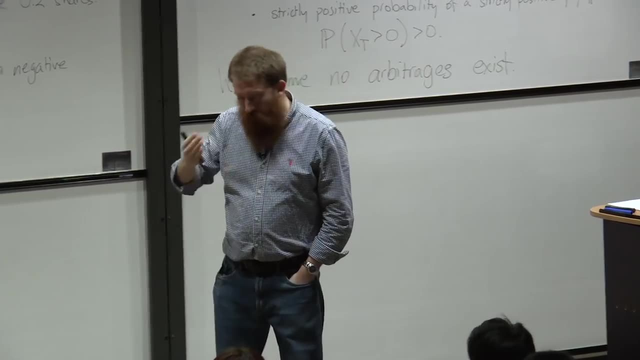 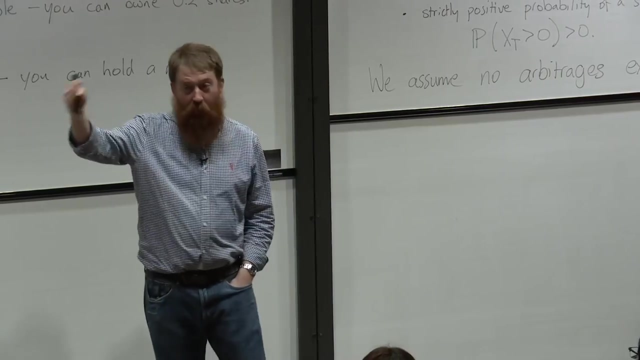 Okay, So what could you do? Well, what you do is you can go to a bank and you say to them: look, this is my situation. I would like an agreement with you to sell US dollars into pound sterling in one year's. 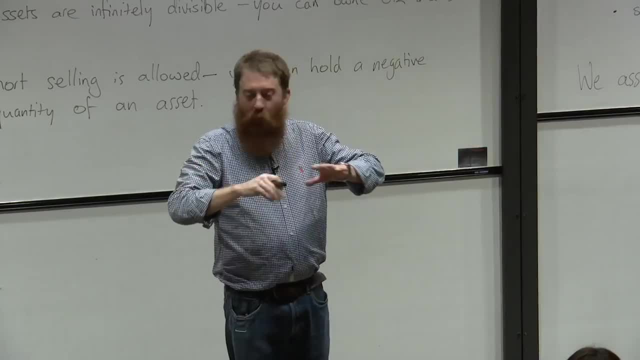 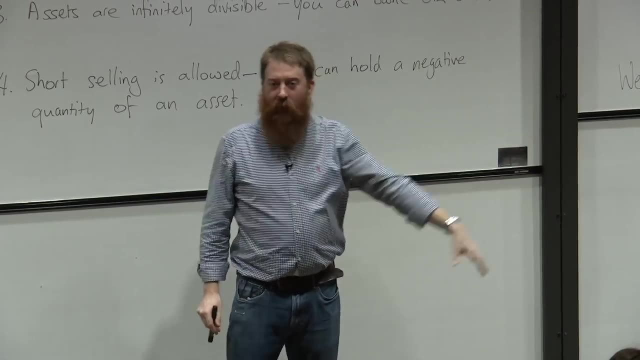 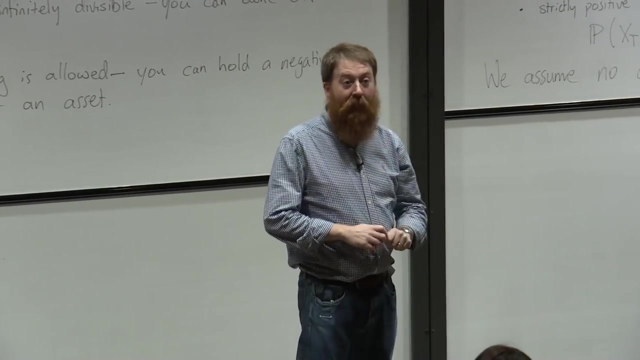 time. Now, there's nothing strange about this contract. All it is is: in one year, I will be giving you, say, one million US dollars, and I would like you to give me however many. it is Okay, Pound sterling. And what you try and do is you go to the bank and say: could we please agree today on the? 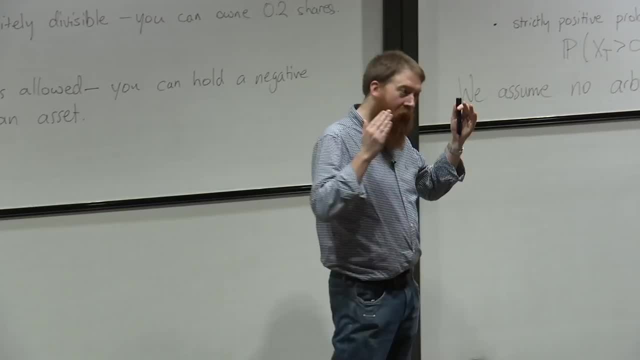 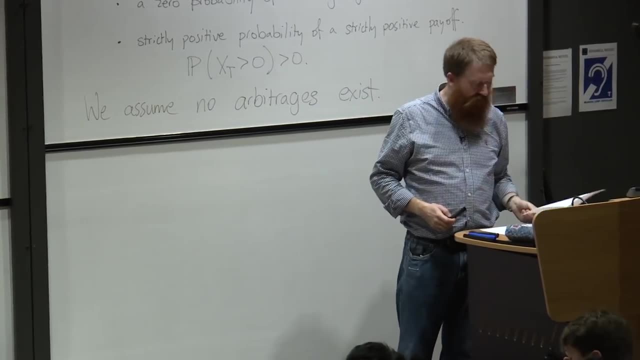 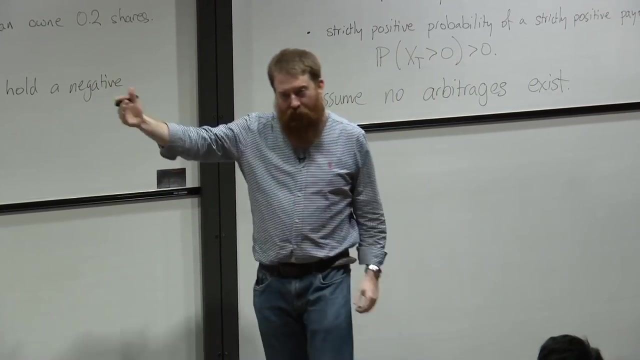 price at which we'll do this deal. Okay, So we're going to agree today on the exchange rate at which we will trade in one year's time, And that's the basic idea of a forward. It's about taking a price today at which we will trade in the future. 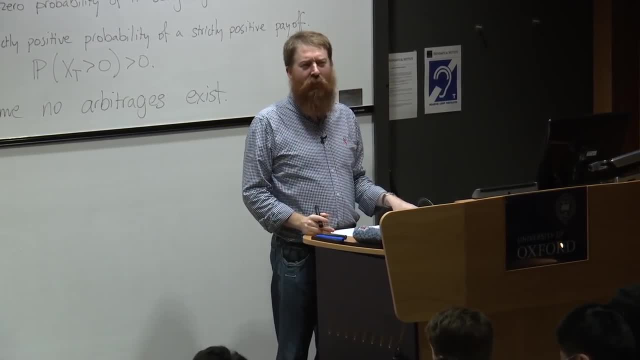 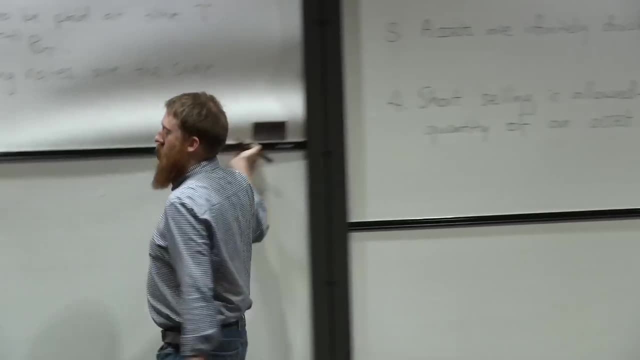 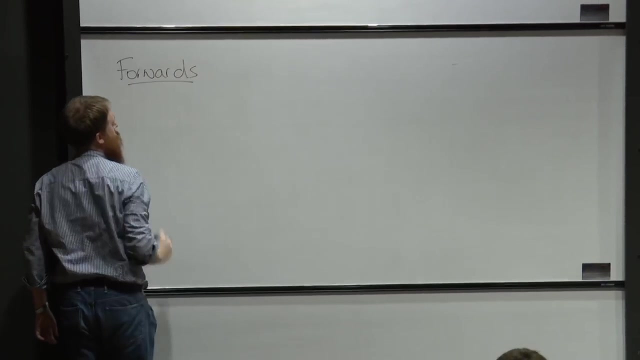 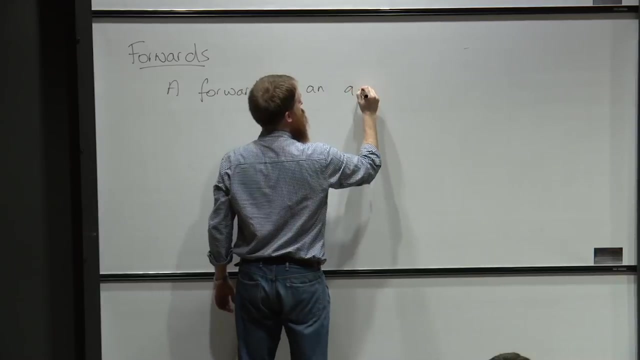 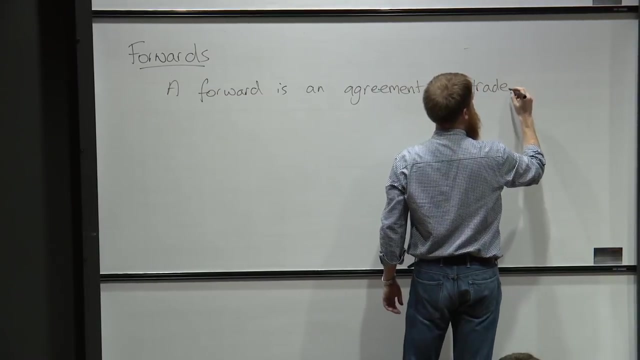 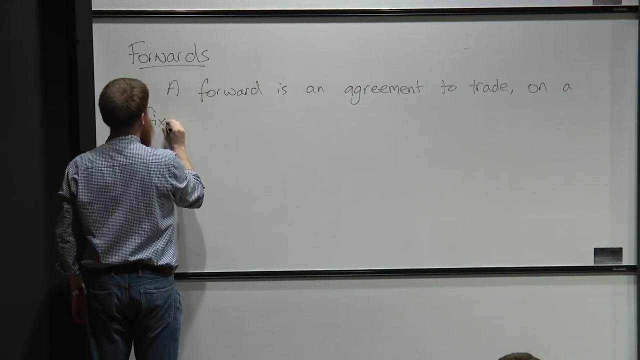 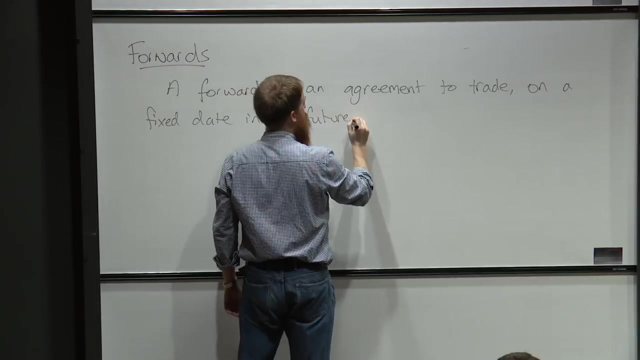 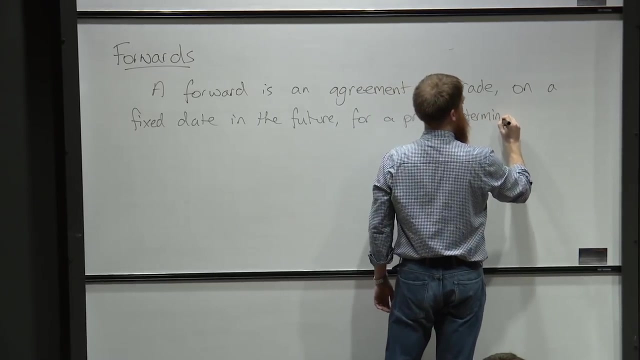 The question is: what price? What should we trade at? So how do we determine the price today? Okay, so let's try and write this out: Okay, A forward is an agreement to trade on a fixed date in the future for a price determined today. 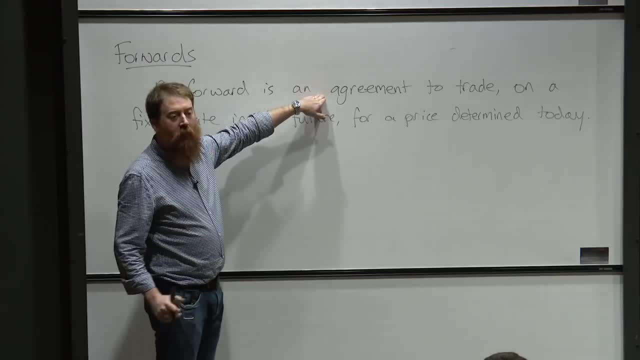 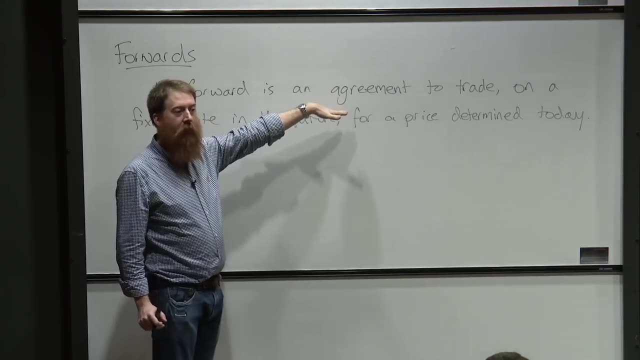 Now one thing to notice. this is an agreement to trade. All parties must trade on that date. There's no way I can get out of this. Once I've signed the contract with the bank, I am legally bound to deliver US dollars in one year's time. 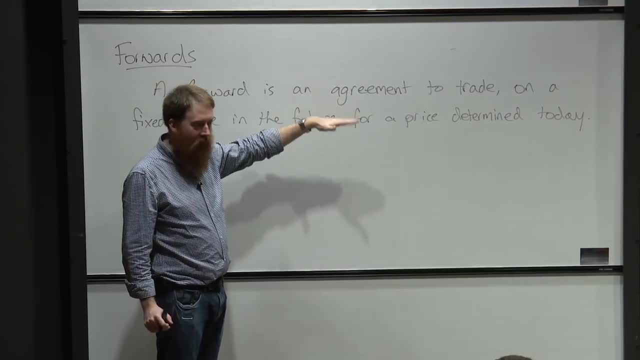 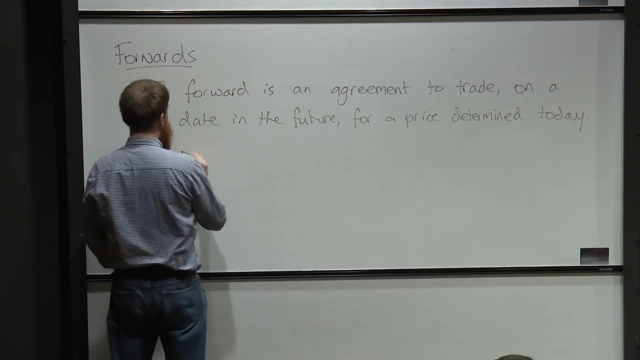 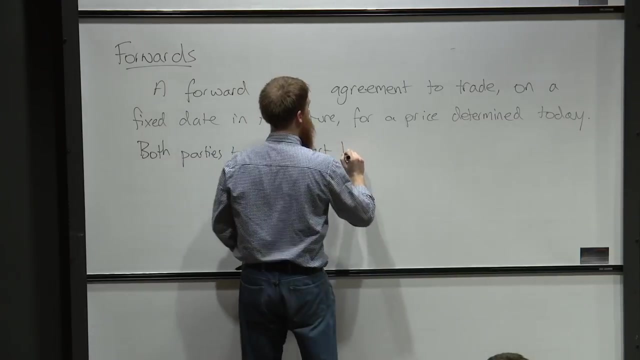 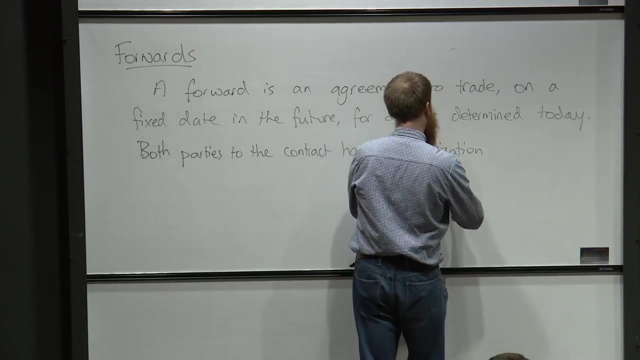 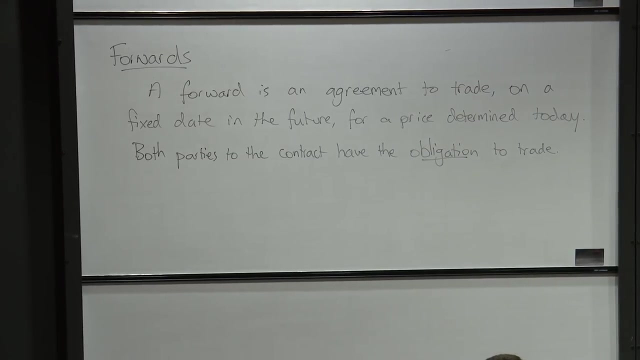 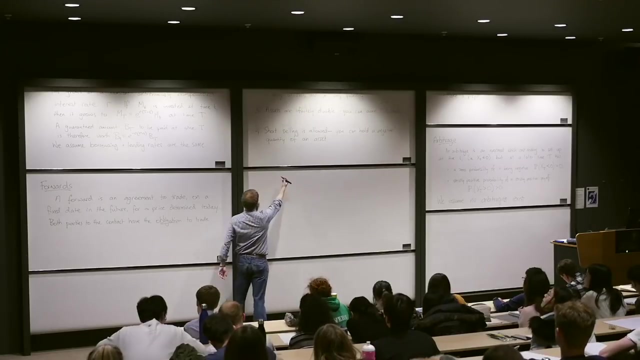 And they are legally bound to deliver pound sterling in one year's time. No one is allowed to back out of the deal. Both parties to the contract have the obligation to trade. So how are we going to find a price for this? OK, let's think about this. 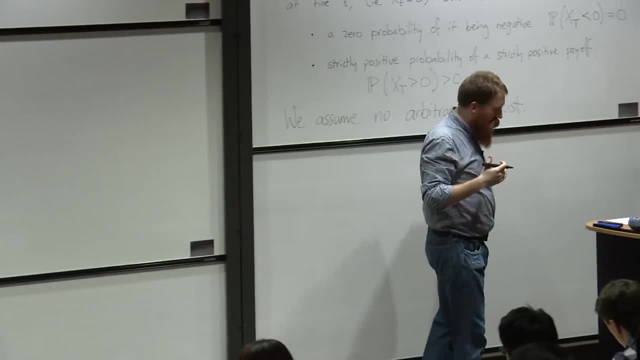 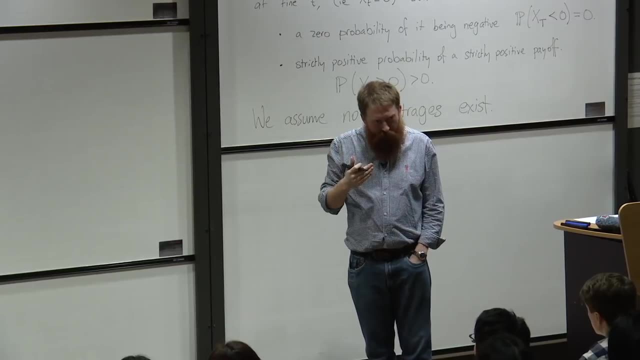 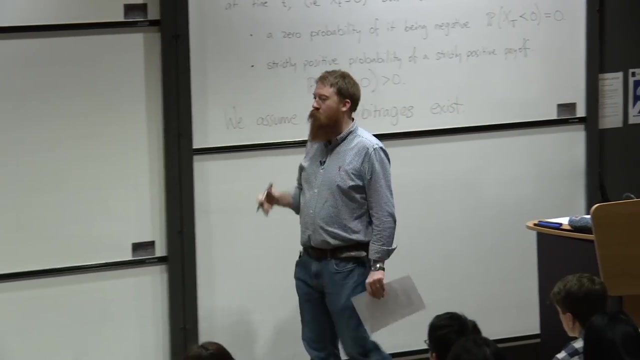 What other options could I do? Well, I know that I'm going to have to sell US dollars in one year. I'm going to have to sell US dollars in one year to get pound sterling. So what I could do- this is called the short position- 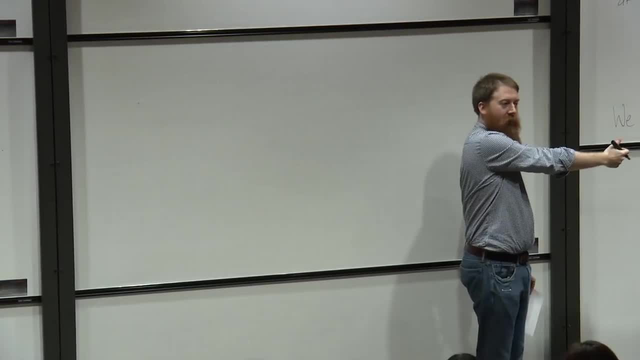 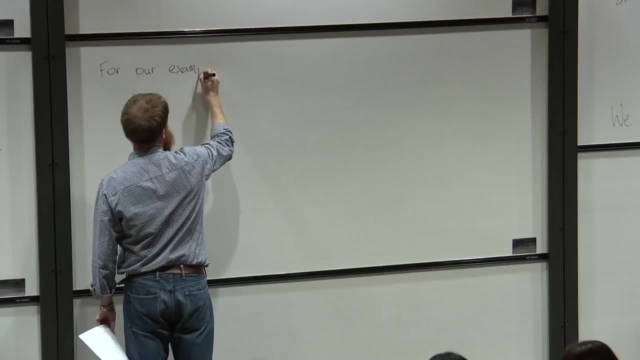 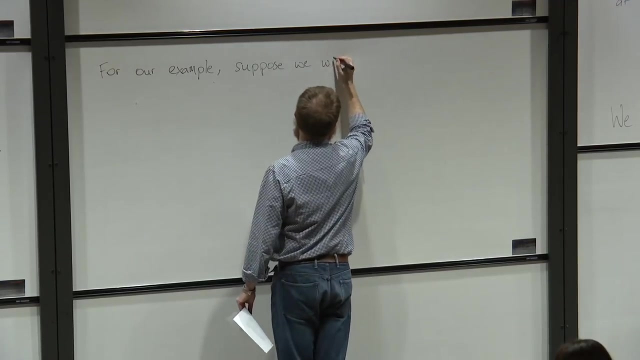 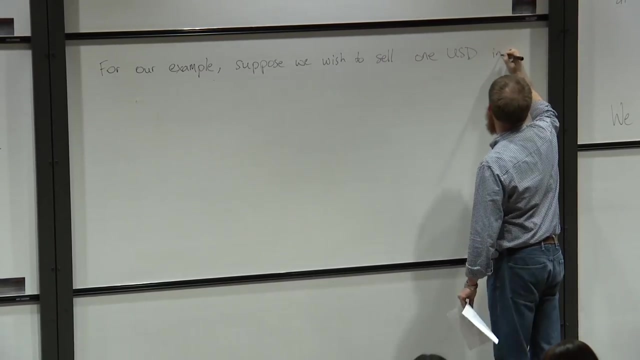 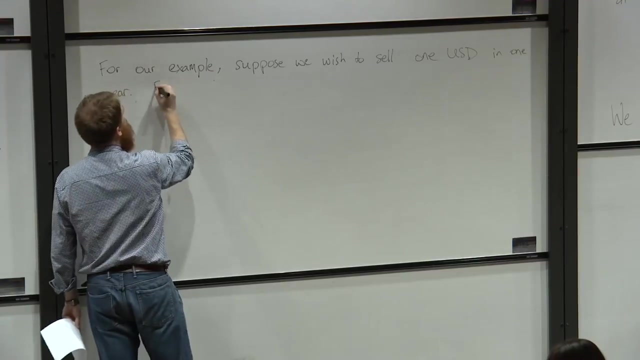 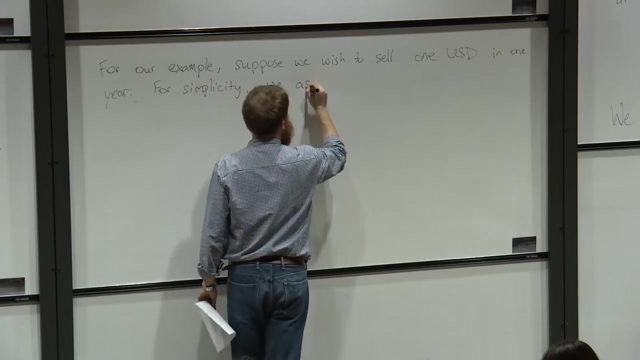 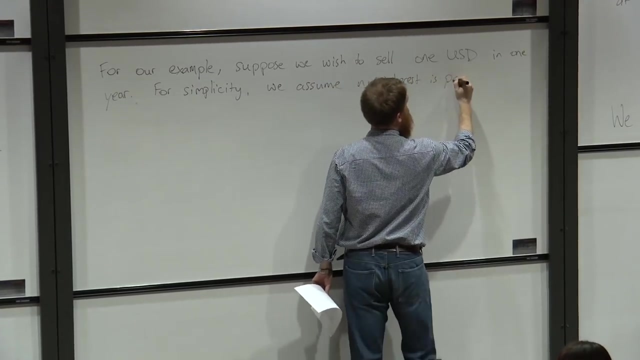 from the UK's perspective, because I am selling the asset. The asset is US dollars. So, for our example, I suppose we wish to sell 1 USD in one year. For simplicity, we assume no interest is paid for holdings. We assume no interest is paid for holding US dollars. 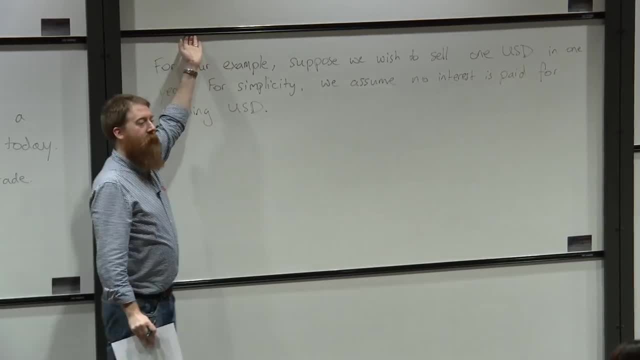 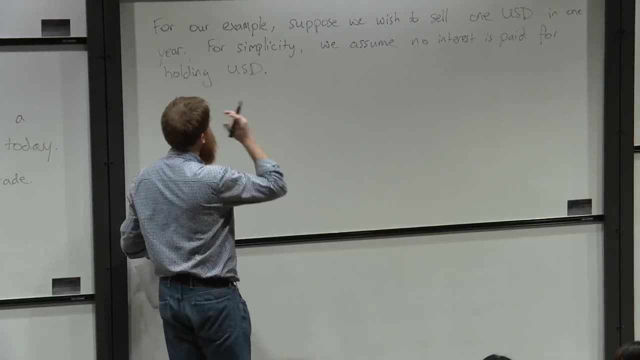 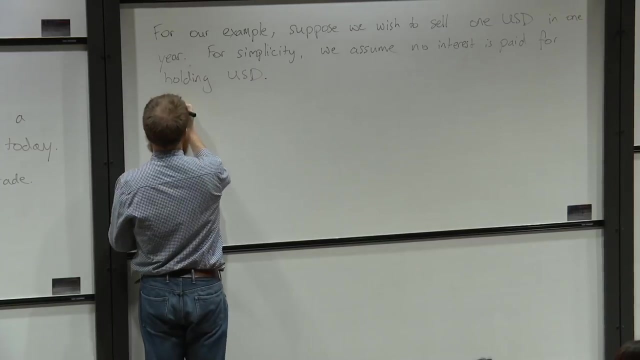 Although we'll come back to that assumption. So let's begin as soon as you hold any US dollars. there's no interest being paid on that. So what could I do? Well, one thing I could say is I could. let's. 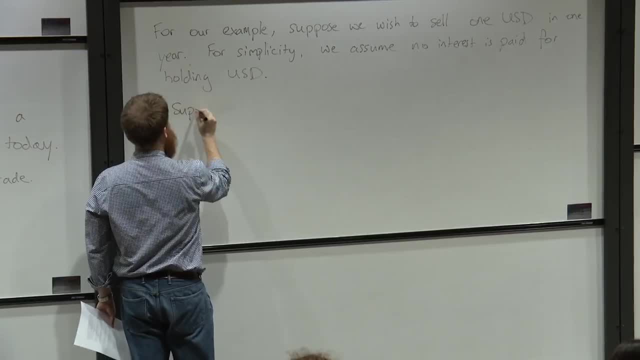 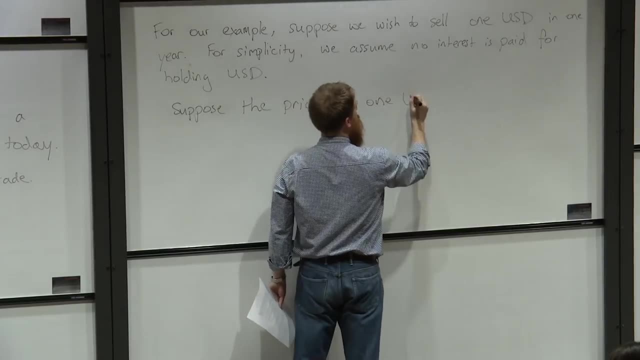 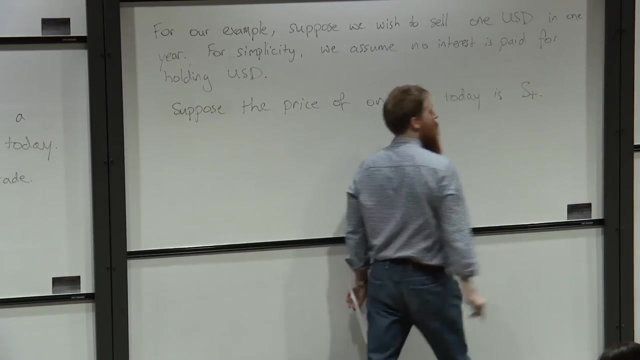 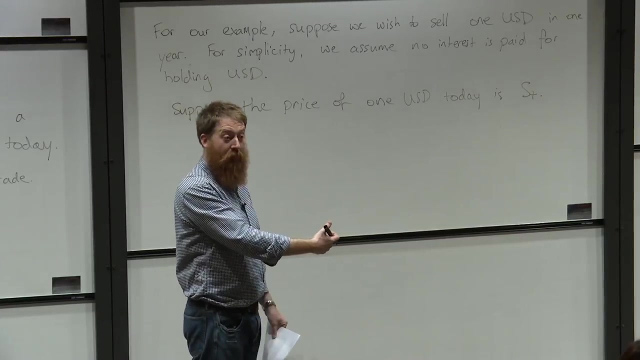 we could do that with the price, but let's assume the price was 1.. Now suppose the price of 1 US dollar today is s little t, So that's the price at which I can buy 1 US dollar in pounds right now. 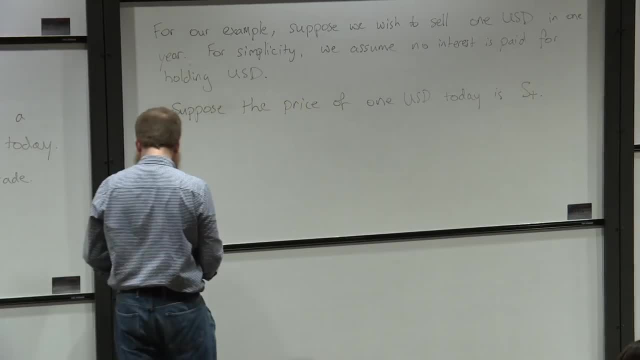 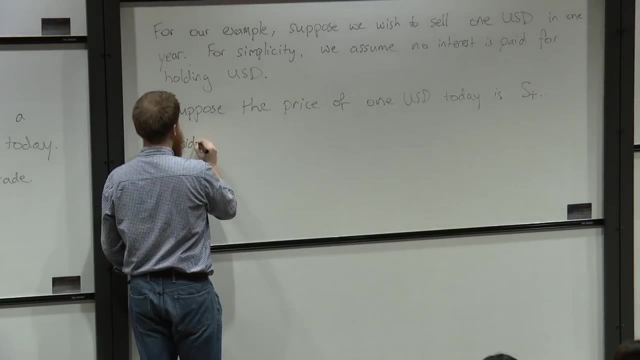 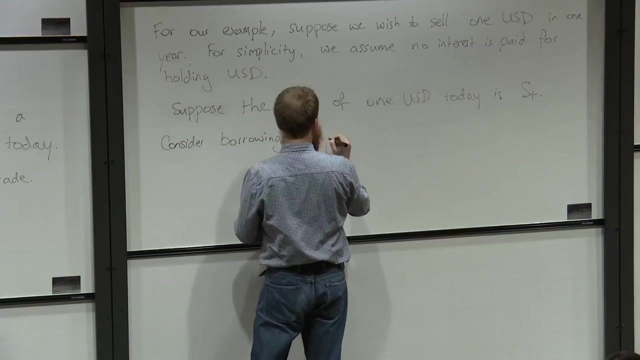 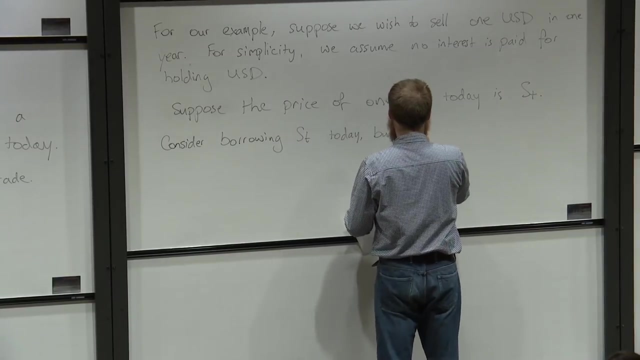 And we've assumed no transaction cost, so I could buy or sell at the same price. OK, we've got the price. We've got the price of 1 US dollar today. So what could I do? Well, I could consider borrowing ST today, buying one US dollar and 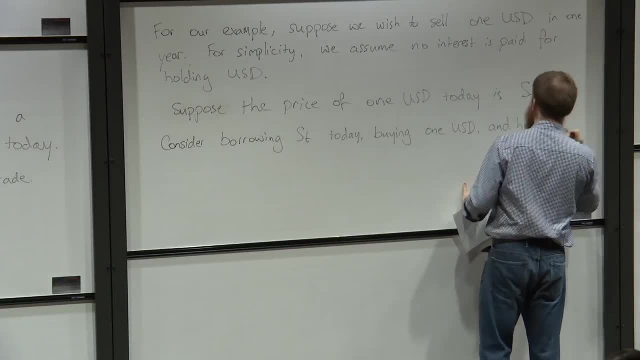 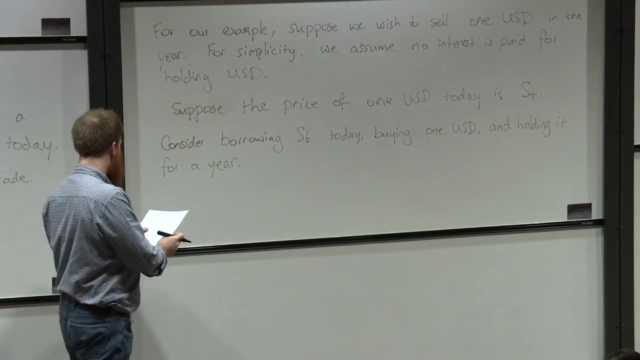 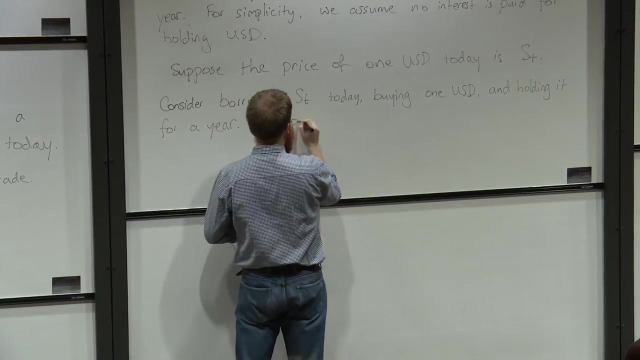 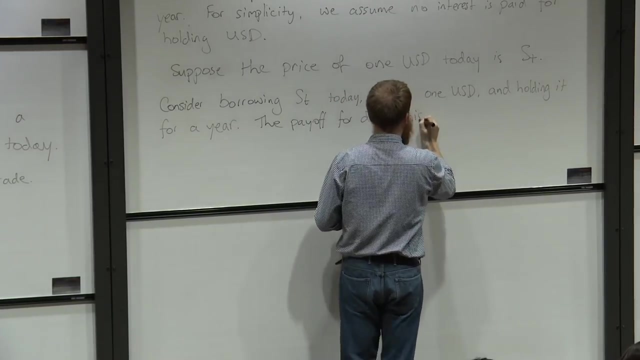 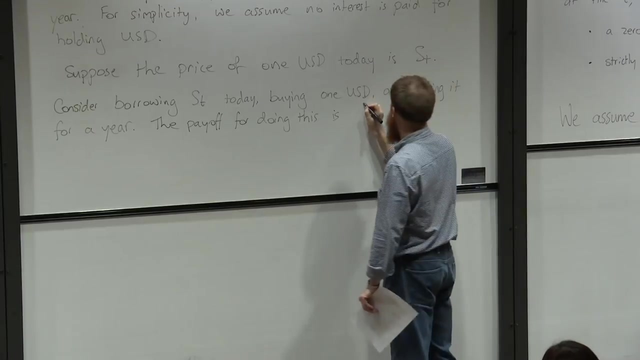 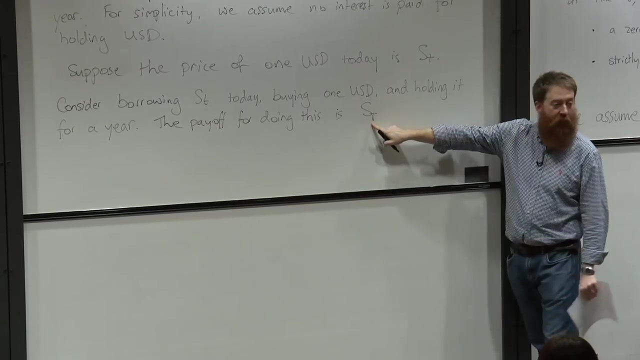 holding it for a year. The payoff for doing this is well. what's the value of my US dollar that I've bought in one year? In one year's time it's ST. That's the future value of one US dollar. I don't know its value. 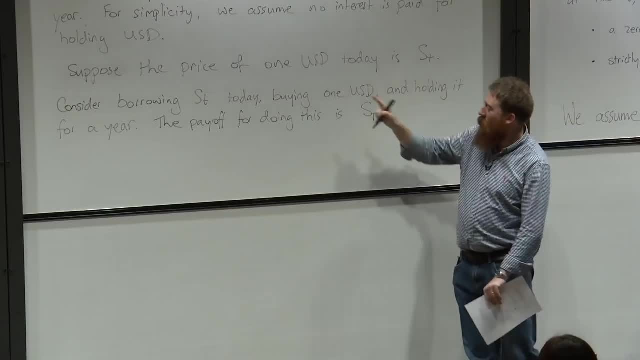 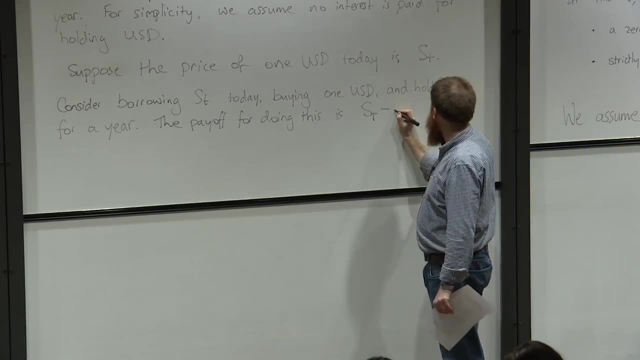 now, I'll only know that at time big T. But I've also had to borrow money and we remember by borrowing ST. today I've had to pay interest on that. So I've got E to the R T minus T. 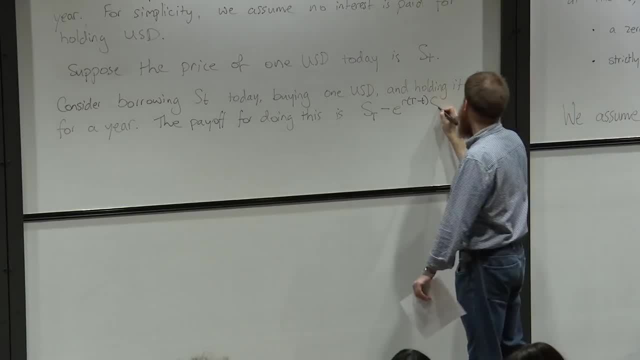 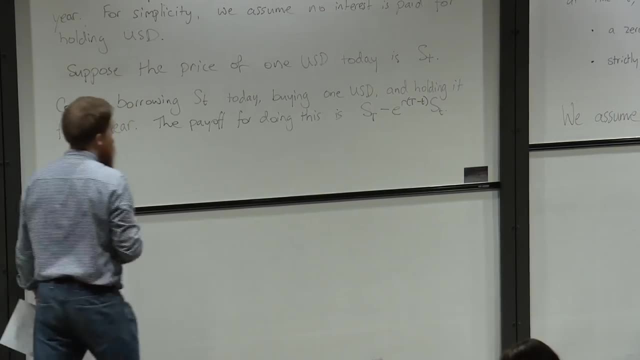 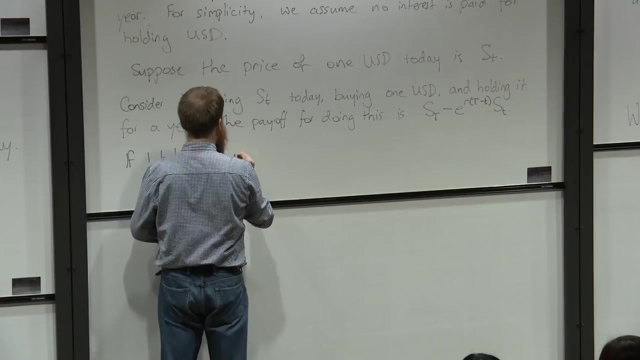 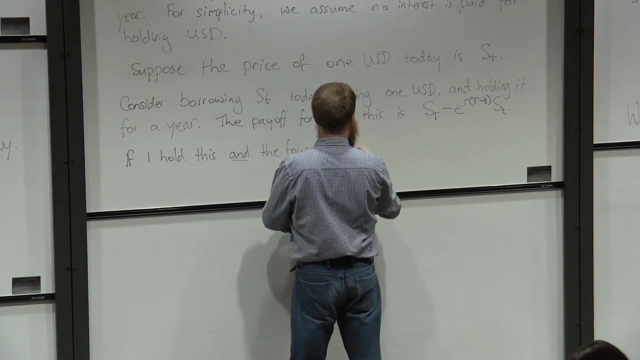 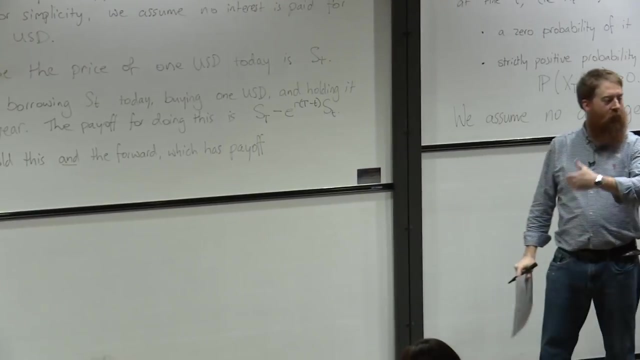 This is my interest rate on the money that I've borrowed in pounds: times the amount that I borrowed, which is ST. Okay If I hold this, and the forward, which has payoff. Well, let's think about this. What's the forward contract worth If I have agreed a price today? 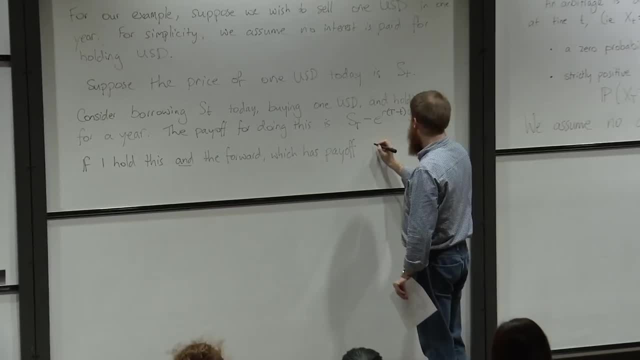 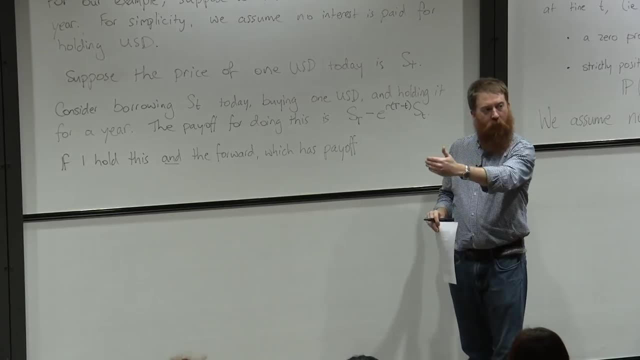 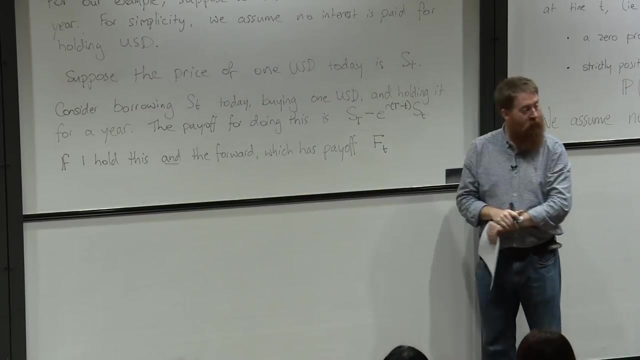 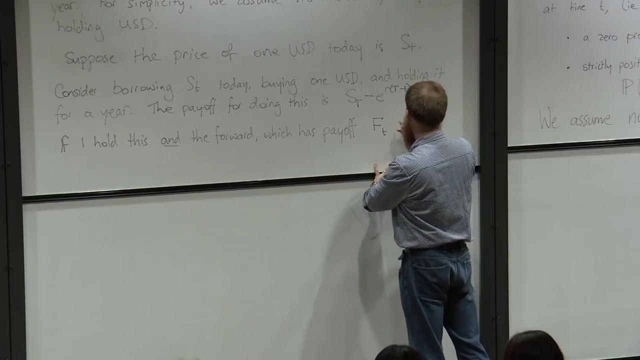 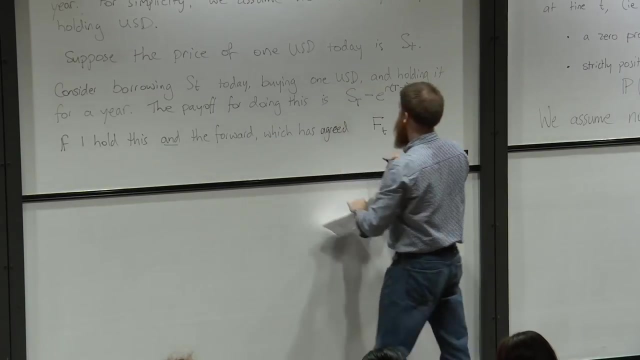 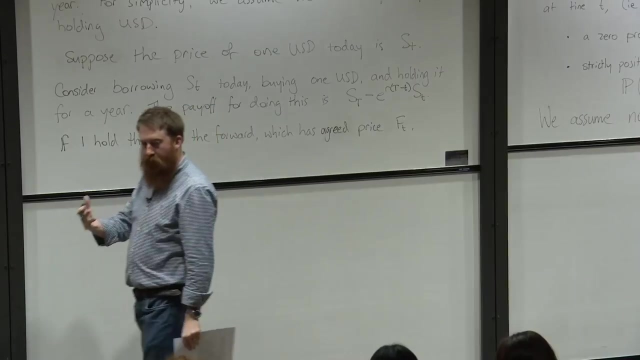 Okay, Then I've got, Well, my US dollar. in one year's time, I can sell it for some amount, Okay, Which is the forward price? Okay, Okay, So agreed, ST, Okay, ST, Okay, So agreed price, FT. So, if I've agreed that price, what's the value of this contract? 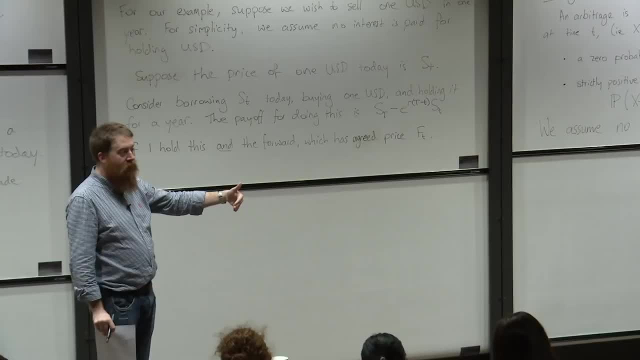 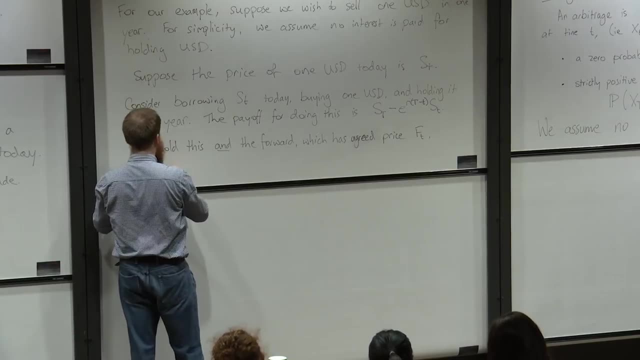 Well, in one year I have agreed to trade at F little t The asset. the US dollar is worth S big T, So I have a payoff which is F little t, which is what I want to trade, Okay. 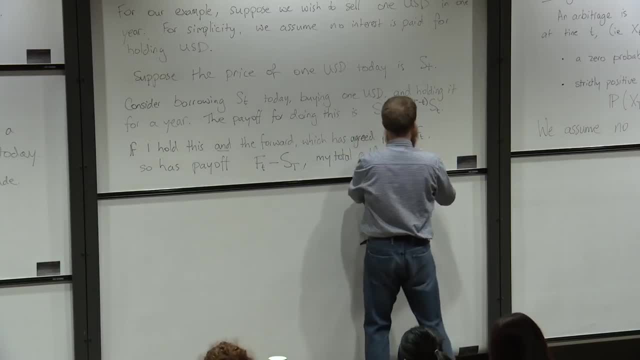 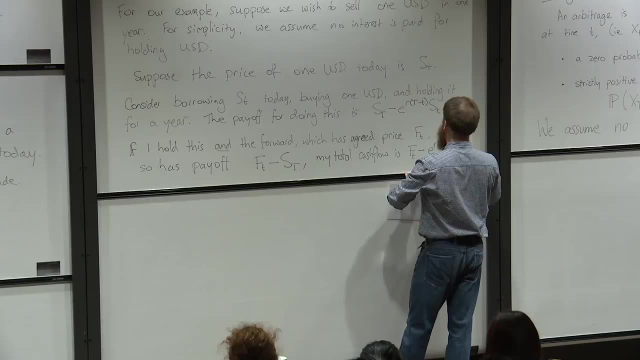 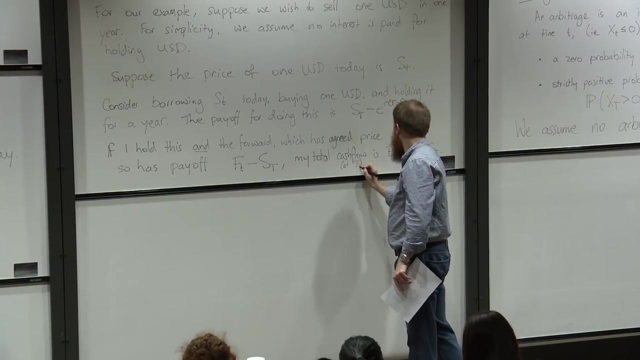 So let's see how this figures out. Okay, St Okay, You have all three options. ST Okay, ST Okay, Wow. FT minus e to the r? AST. So this is my cash flow, sorry, total profit. 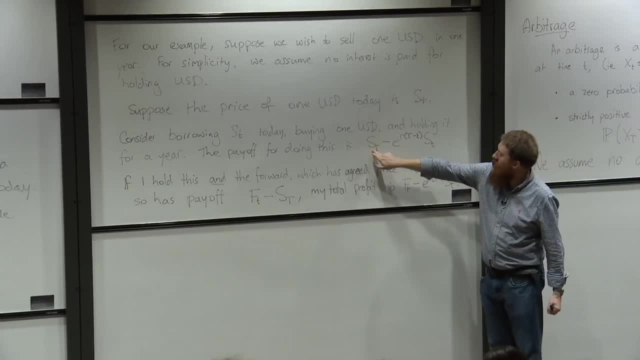 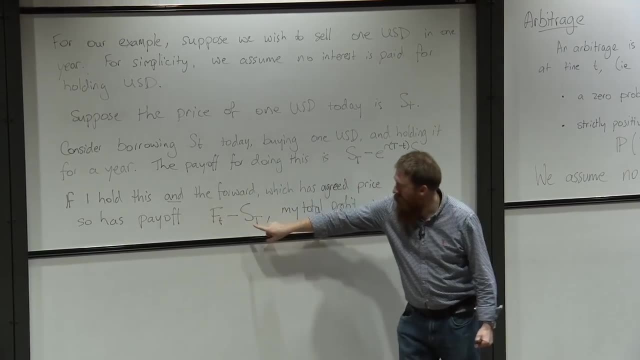 Everyone see where I've got that from. So I've got my terminal payoff. This is what I paid for the amount that I borrowed. I've got my forward contract, which I agree a price on today, But I'm effectively losing out because I'm not getting the value of the stock in the future. 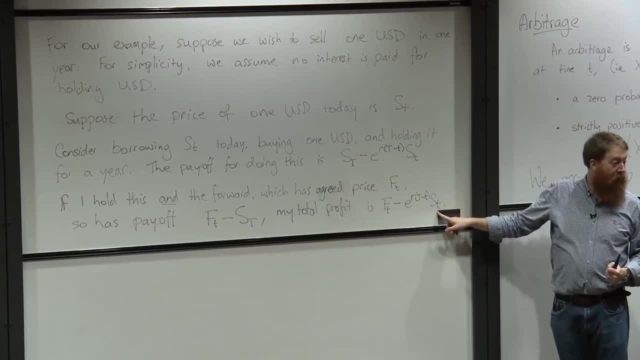 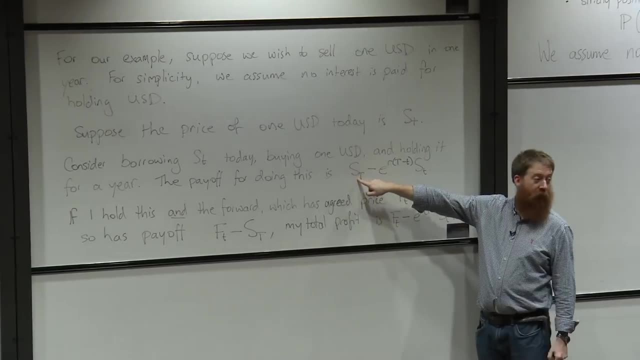 But if I add these two together, I just get this payoff here. The interesting thing is- well, the problem of figuring out the value of this- was that I don't know the value of ST yet. That I'll only know in one year's time, at the terminal point of my contracts. 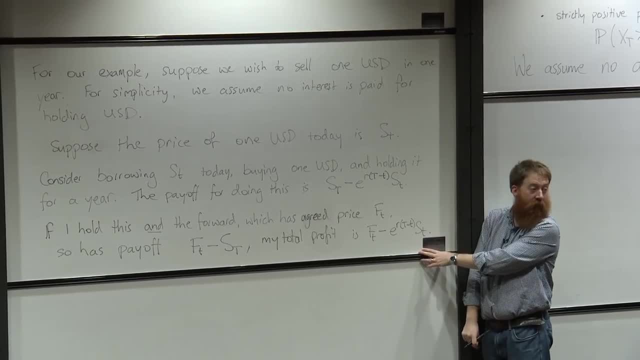 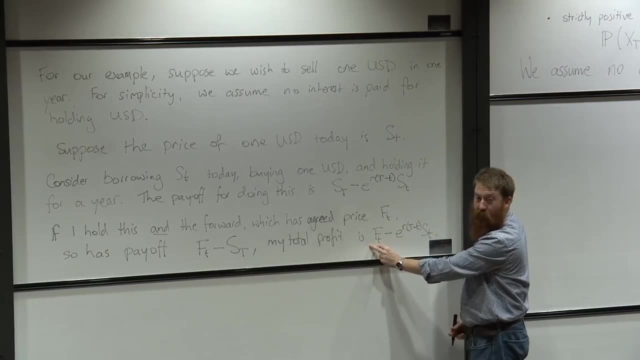 But this depends on things that I know today. There's nothing risky in here. I've got. this is the amount that I've borrowed. I know what I'm going to pay for that. This is the price I'm agreeing on today. 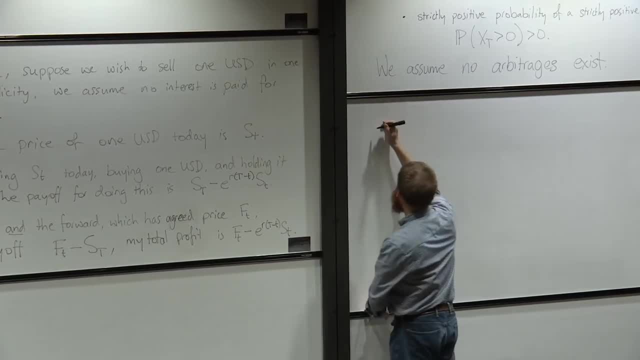 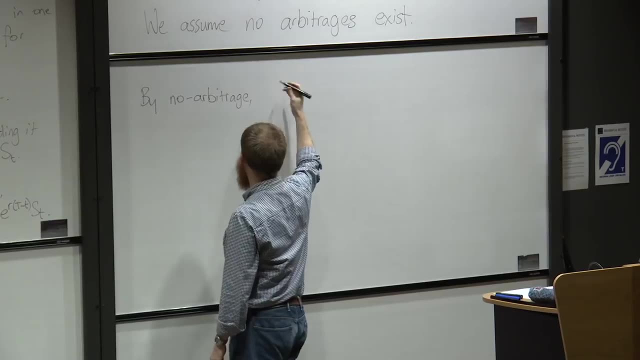 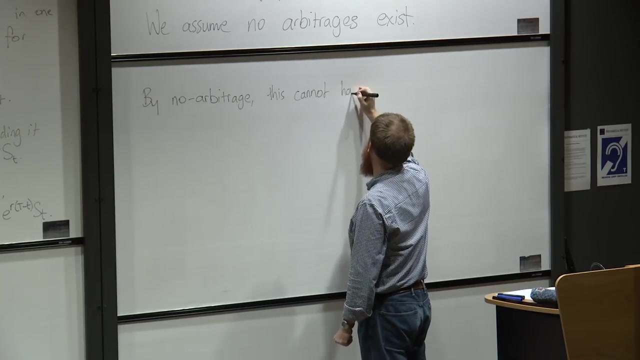 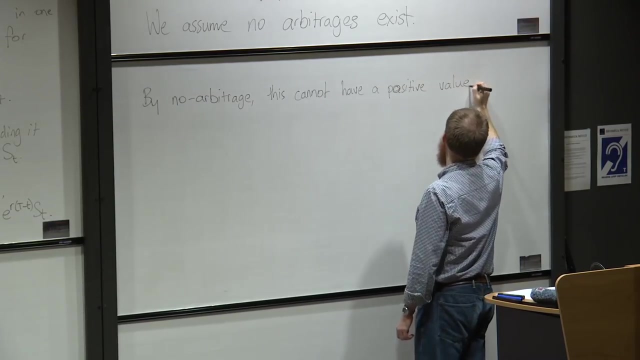 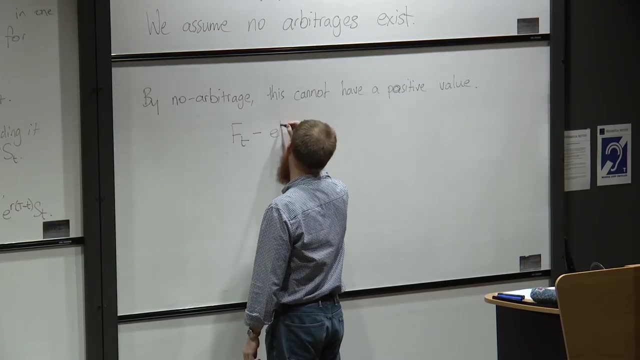 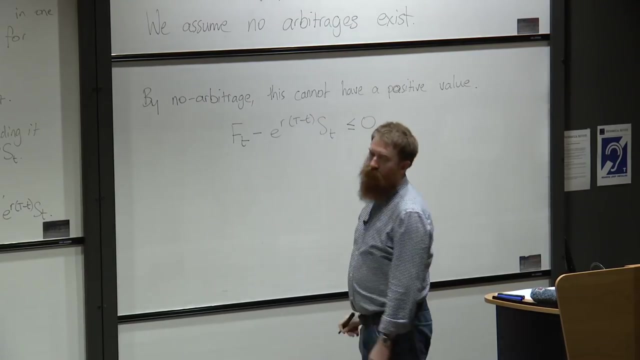 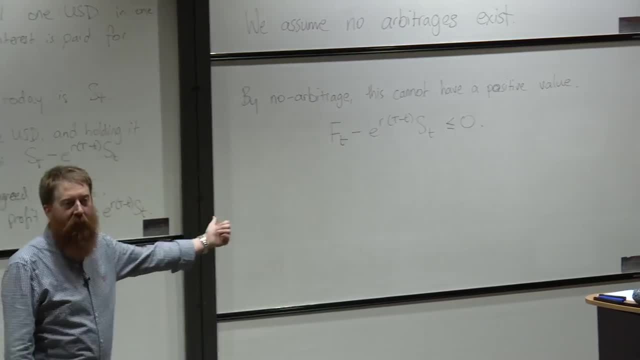 I don't know what the price of my current contract is. That has to be negative, Because if that was positive, this would be free money. I'd go and do this deal, I'd enter into the forward contract, I would borrow money. 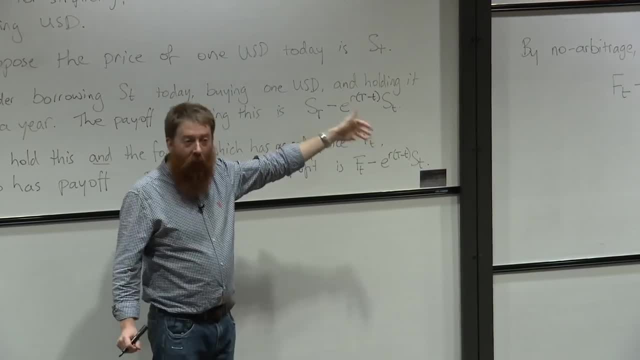 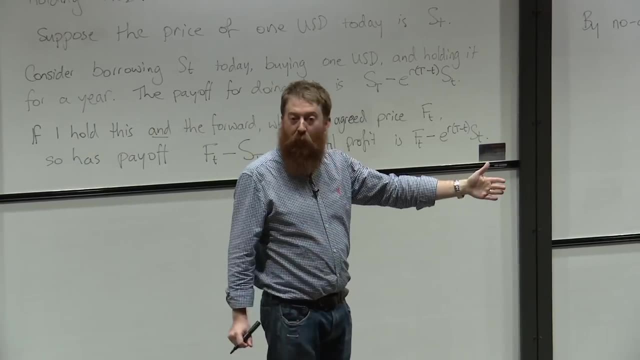 I would buy US dollars And in one year's time I would have money. It costs me nothing today. Forward contracts, I'm not paying you anything today. We're just agreeing a price- No cash exchange today, And so if this were a positive amount, 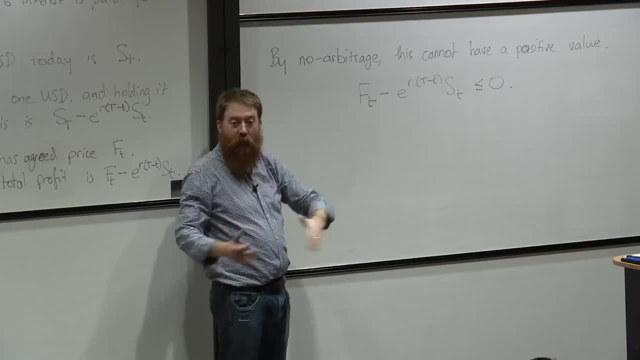 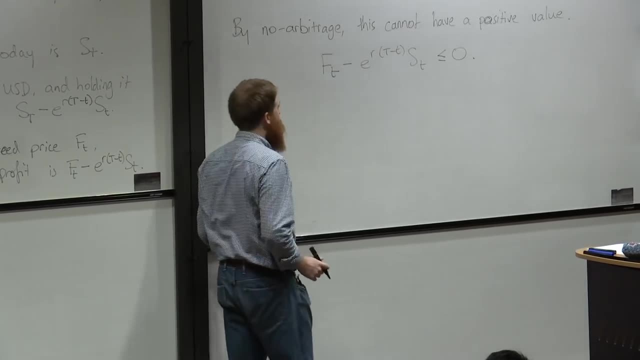 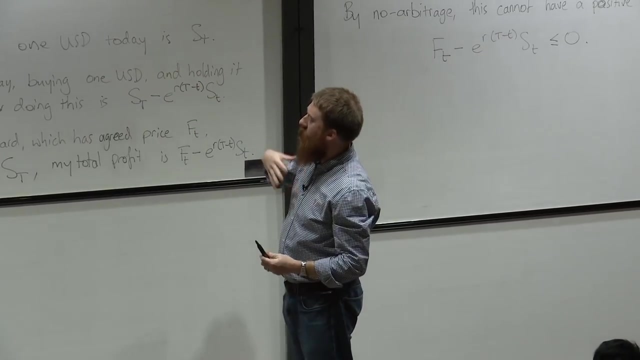 then I'd be able to make money for nothing. So that's an arbitrage which we've excluded from our models. So we certainly know that this quantity must be negative. Well, what about the other side? So this was, if I was thinking as myself. 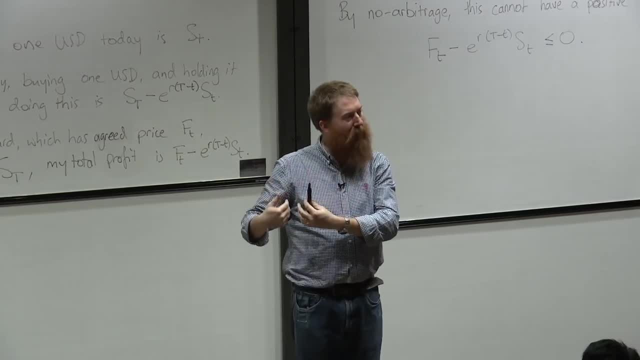 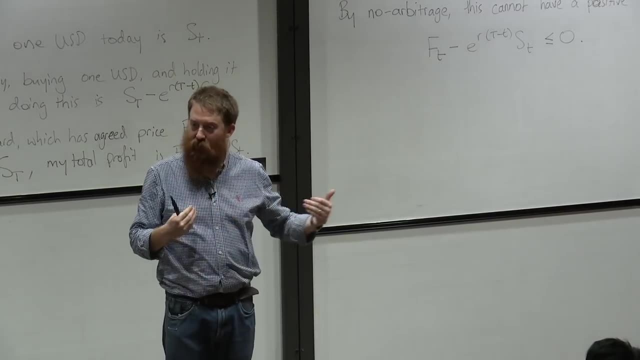 But what I could do is I could instead think: what if I was my bank? So what's my bank's position? They're doing everything opposite to me, So they're selling me. they're agreeing the price to do the trade the other way. 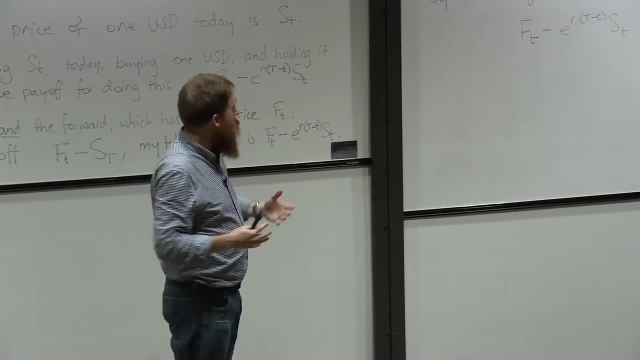 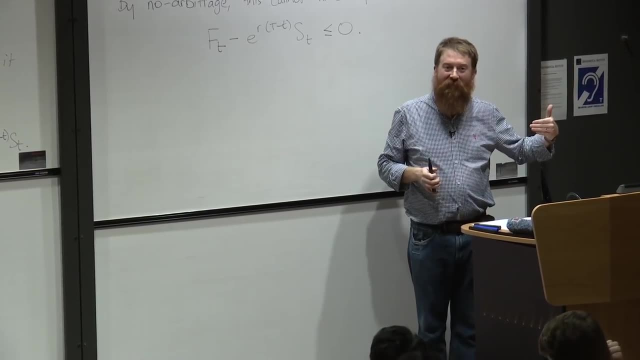 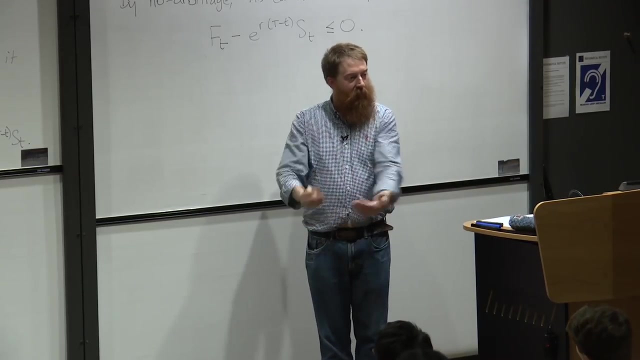 And they could borrow money. They could effectively take money invested and sell US dollars. OK, So instead of buying a US dollar, they short sell a US dollar. Instead of borrowing money, they invest money. So they do everything with the opposite sign to me. 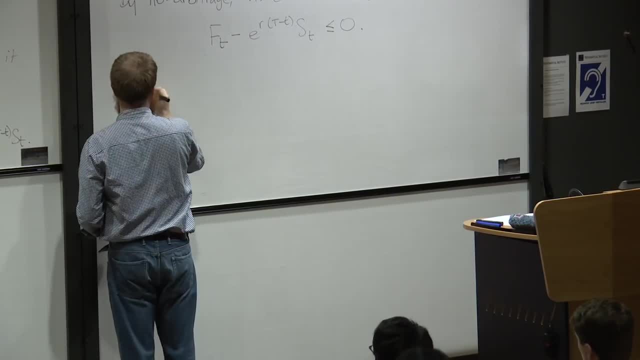 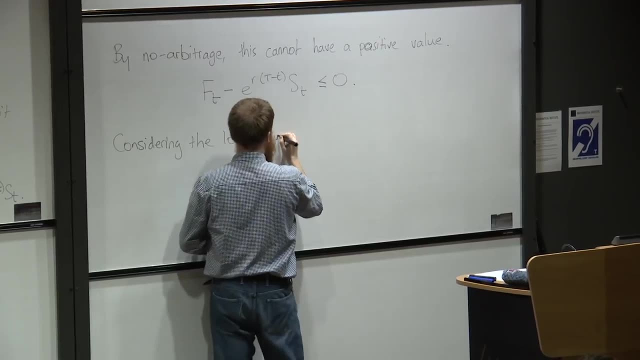 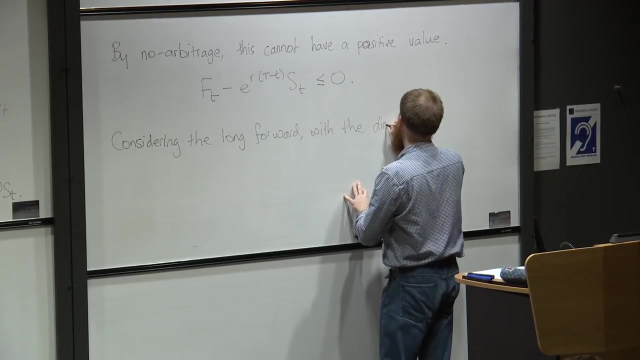 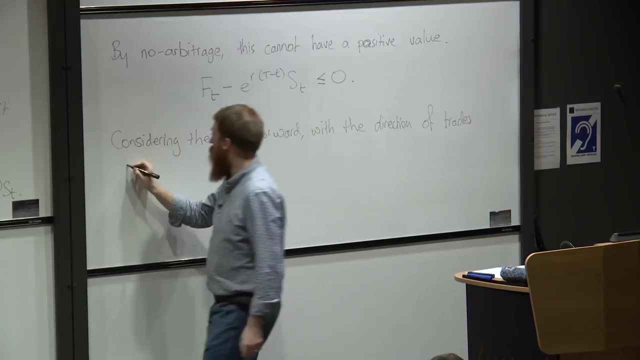 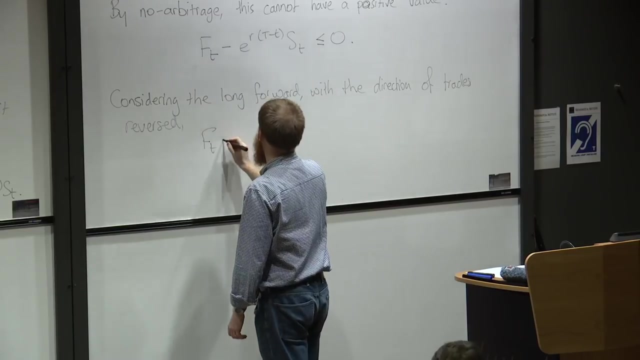 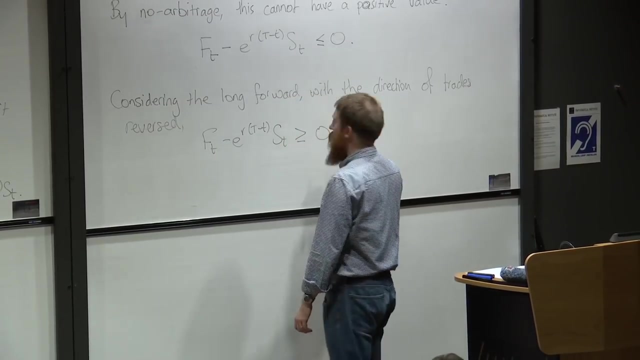 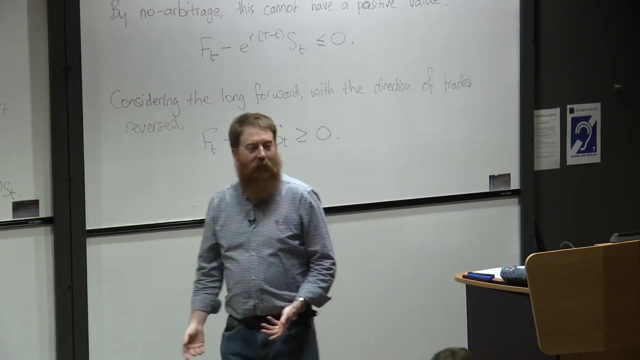 So, considering the long forward with the direction of trades, we get reversed. We get that Because if it was possible for my bank to just go and make money, then that's an arbitrage for them And in fact, if they're offering me a deal. 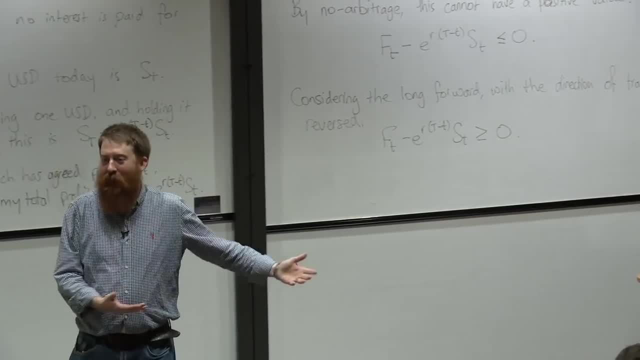 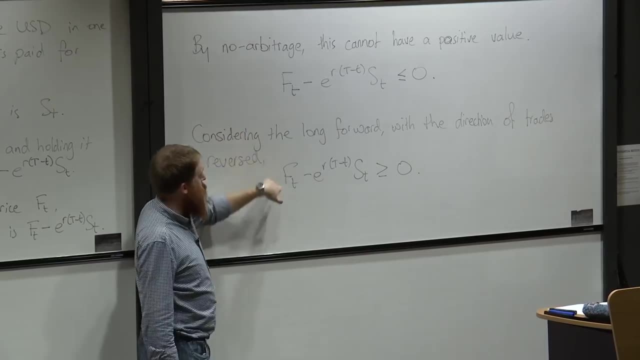 which, OK, there's money on the table, I can make money for doing nothing. Well, we do this. That's an arbitrage, So we're going to assume this can't happen either. But now we put those two together. 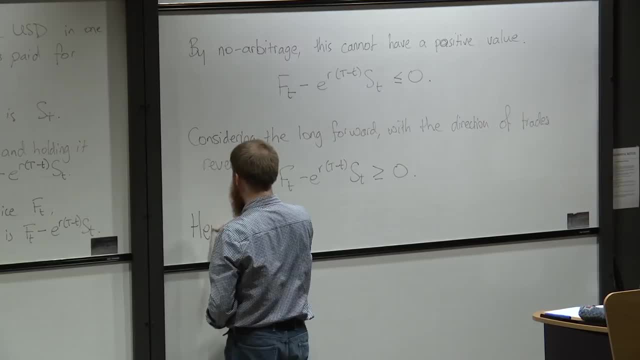 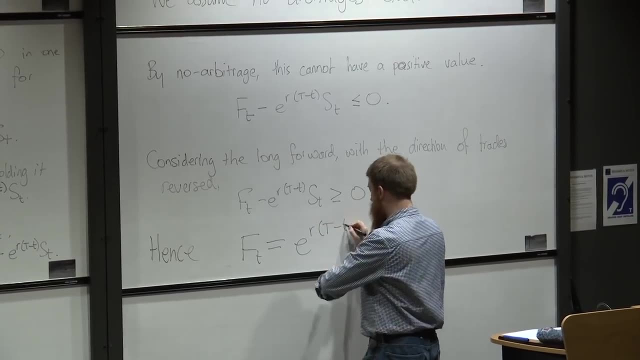 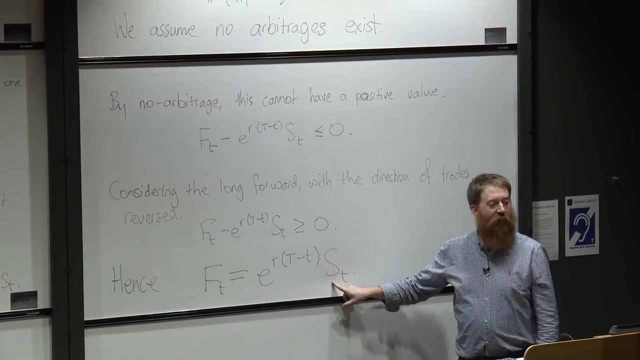 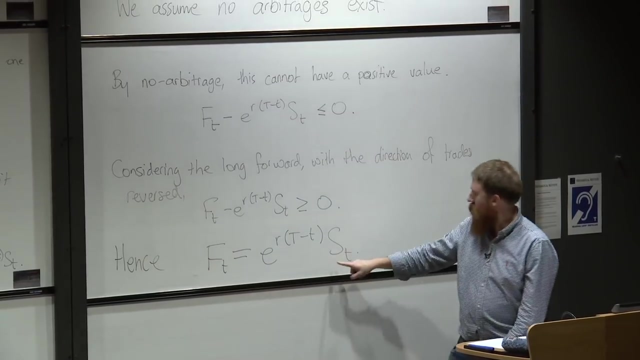 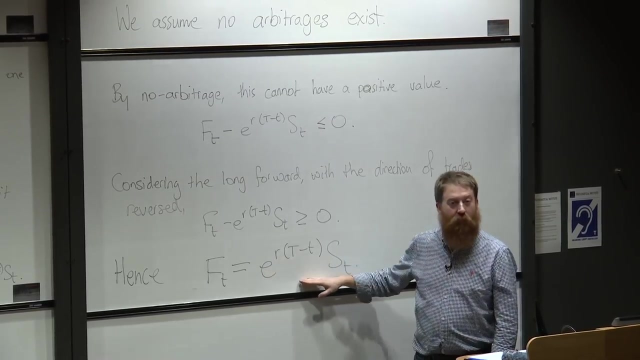 and we find that the forward price is equal e to the r? t. take t times st. That is the current price of one US dollar. So the price at which we agree to trade in the future depends on the current exchange rate. well, the current exchange rate and the interest rate payments. 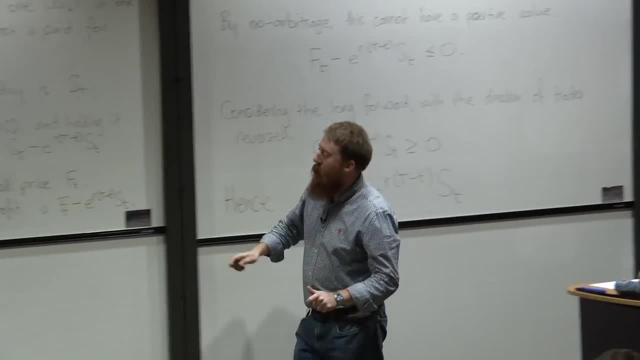 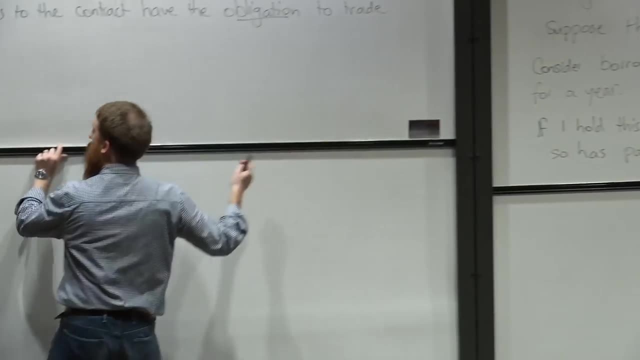 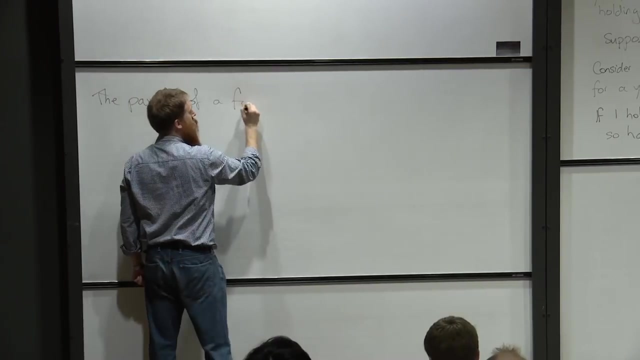 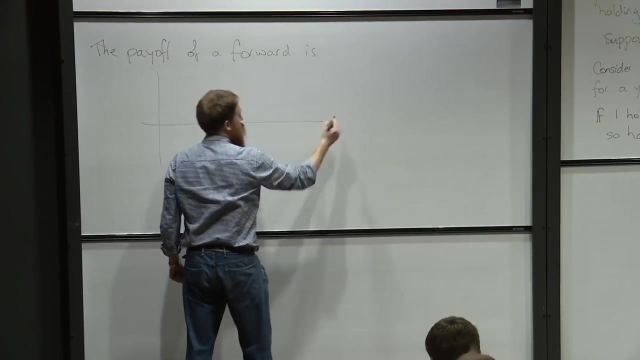 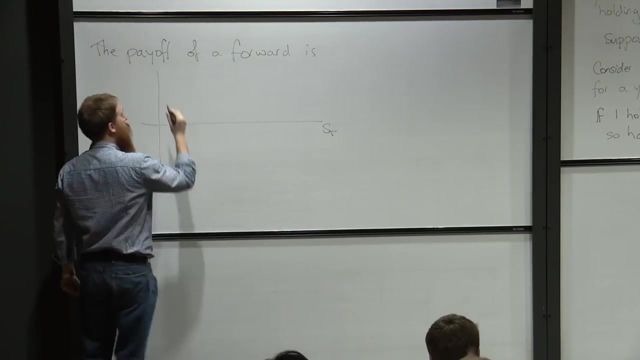 So, just before we continue, we should just think a little bit about this. this payoff here, So the payoff of a forward, is so, if this is the stock price, OK, this is the payoff. Well, if I go for the short forward, which? 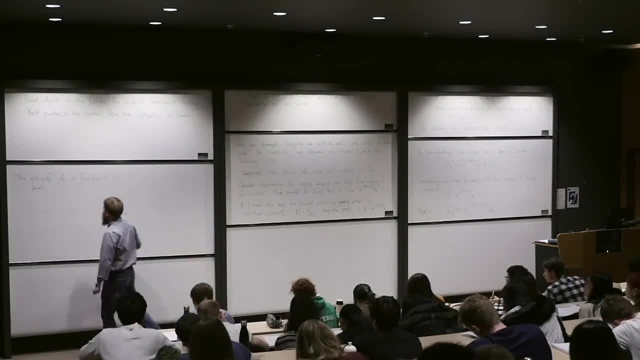 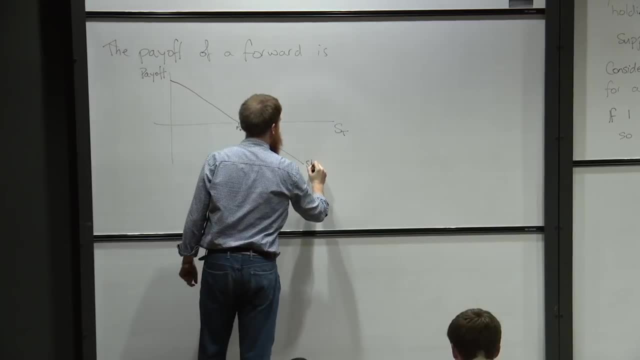 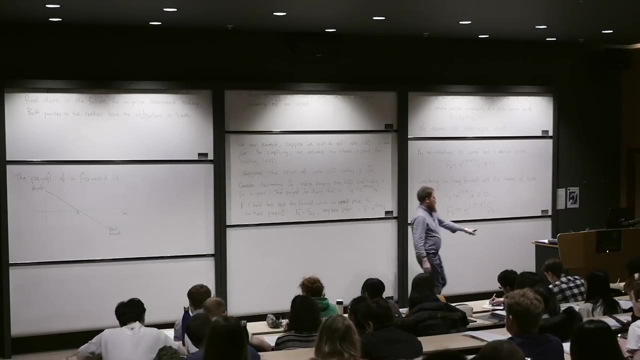 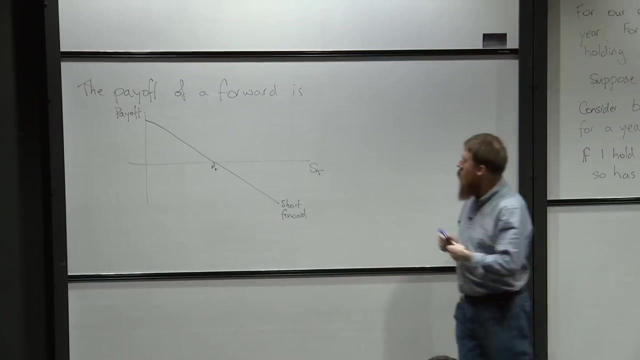 is what I've described here. So that's an agreement to sell the asset- Then the payoff looks like this. On the other hand, if I look at the other side of the deal- an agreement to buy the asset in one year's time- 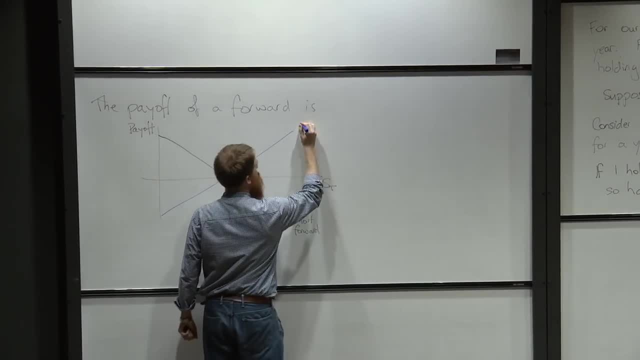 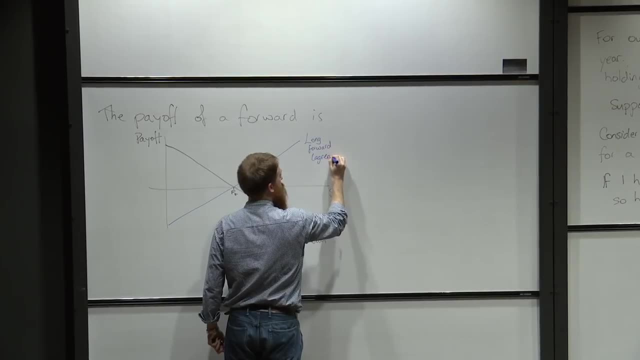 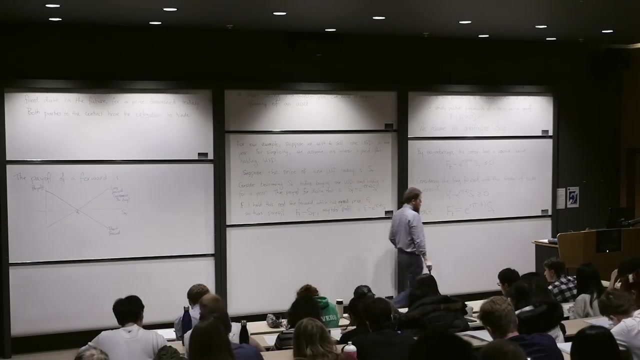 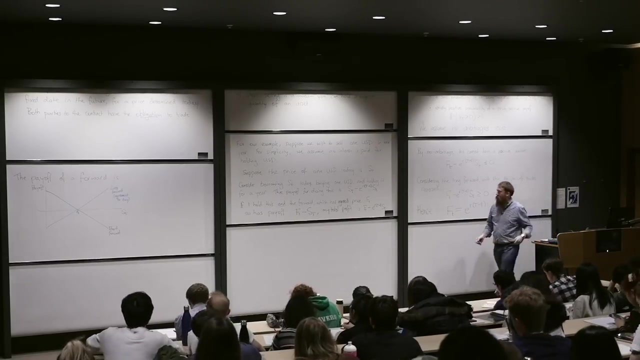 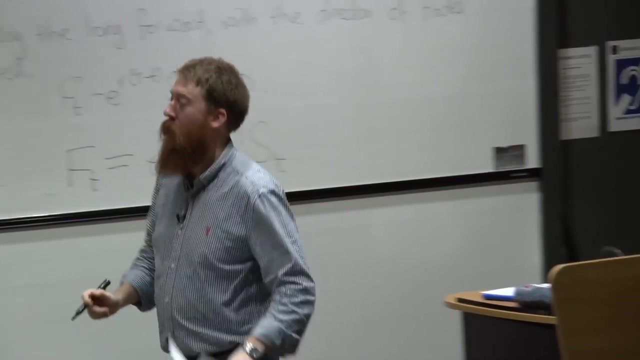 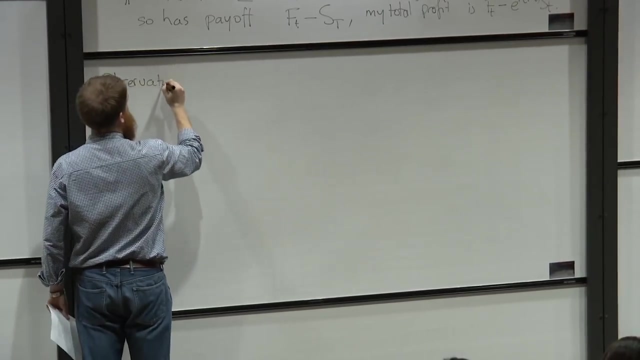 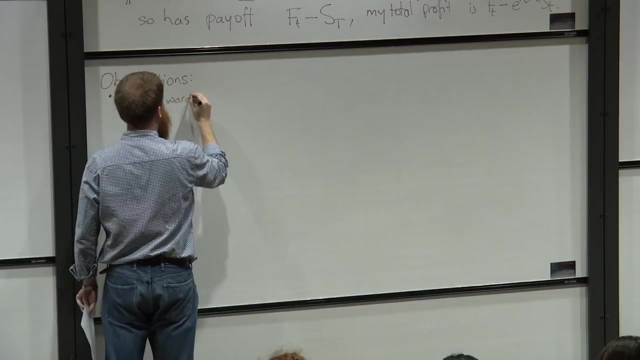 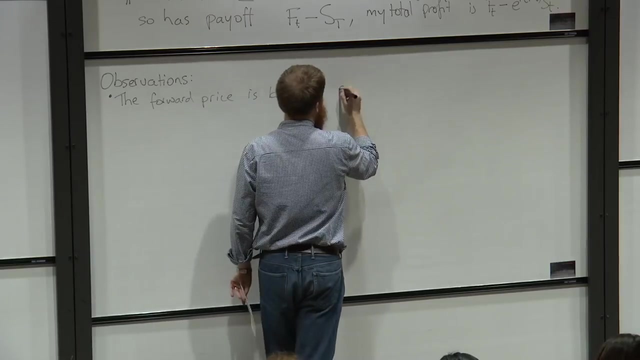 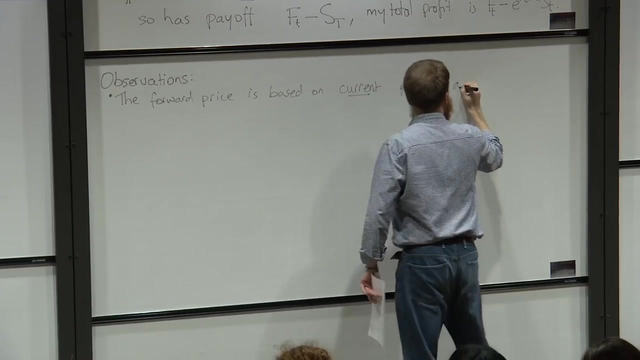 then I get the opposite. This is the long. It's just the felt forward. OK, So what are some peculiar things that we notice when we're doing this? OK, observations: The forward value, forward price, is based on current prices and interest payments. It does not depend on whether ST is a fair price or the asset. I have made no assumption anywhere that the current exchange rate is a sensible exchange rate, and there's something a little bit weird going on here that I haven't even assumed anything about the future evolution of the exchange rate. 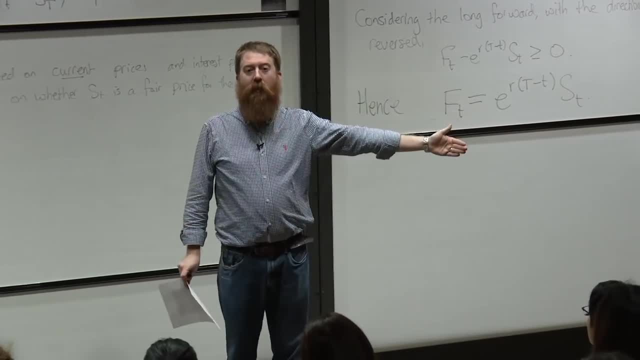 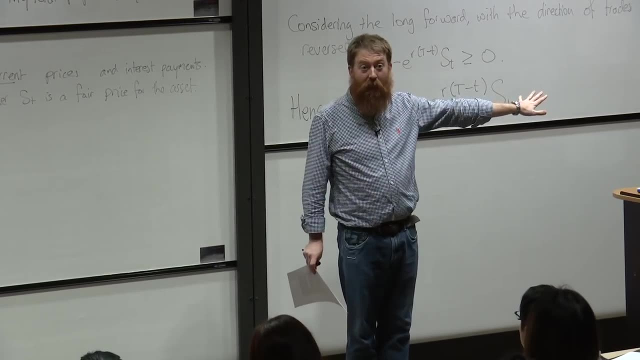 We're making an agreement for what's going to happen in one year's time, and I have told you nothing about what I think the exchange rate will be in one year's time. That has not entered into our calculations at all. So, even though we've 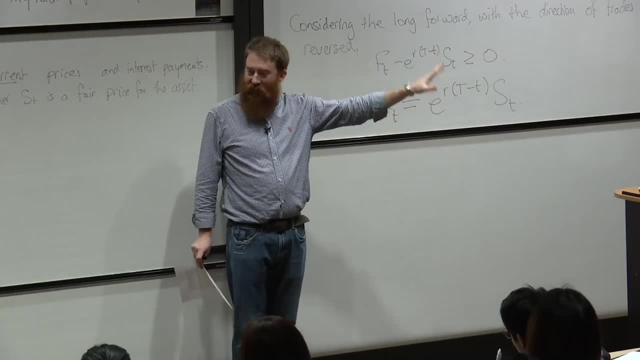 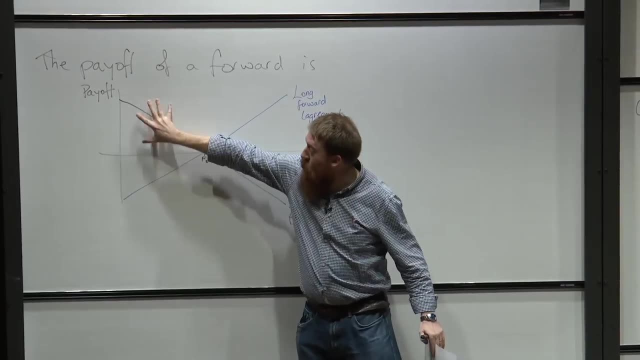 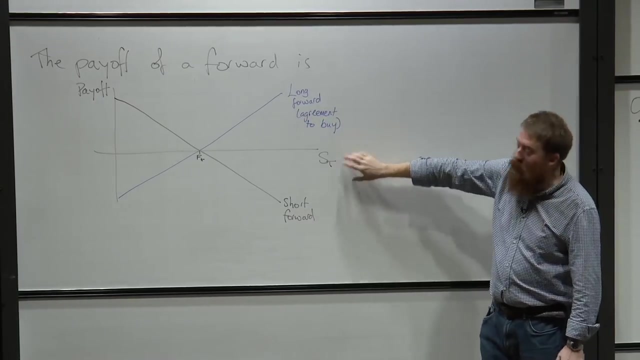 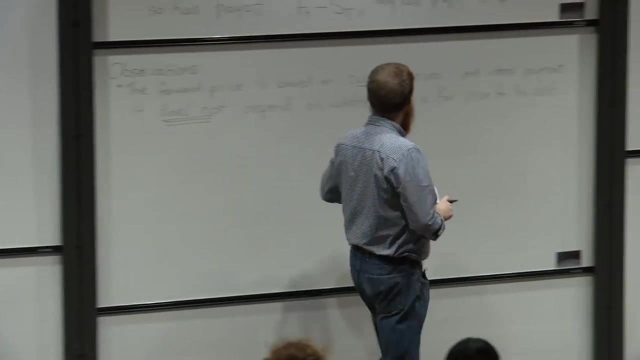 got a contract, the payoff of which depends on the exchange rate in one year's time. whether it's profitable- whether I make a profit or loss- depends on what the exchange rate in one year's time is. we have not used any statements about what I think. this is what I think the exchange rate will be Now. 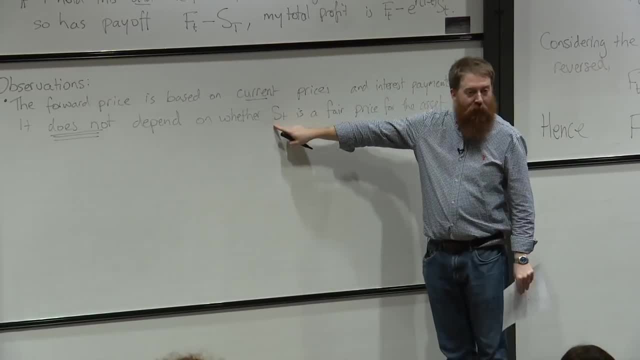 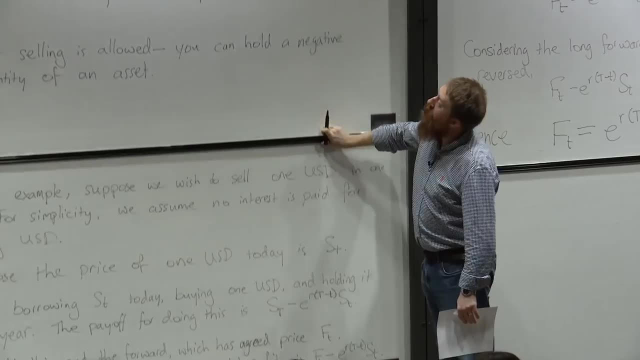 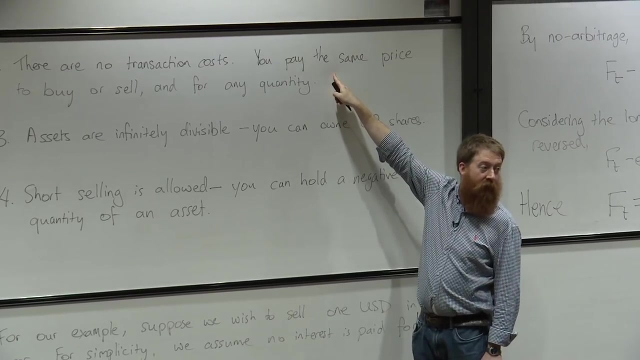 if you've got an efficient market, then this should be a fair price. And there is a secret assumption. it's not so secret, we made it up here. there are no transaction costs and I can buy and sell any amount for the same price. So because of that, if there was money on the table, if this was, 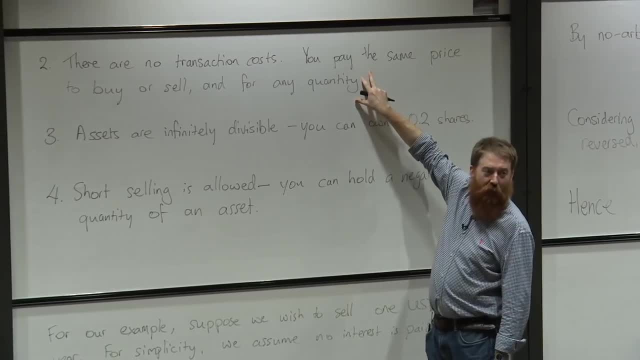 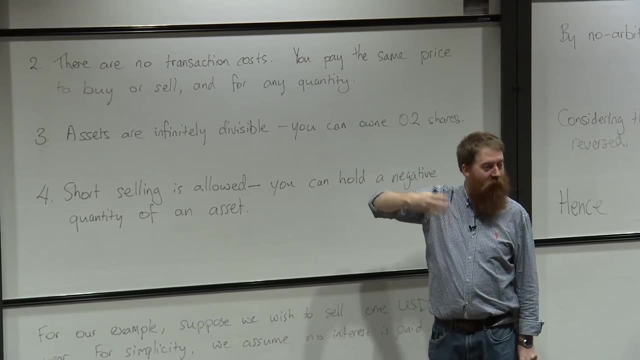 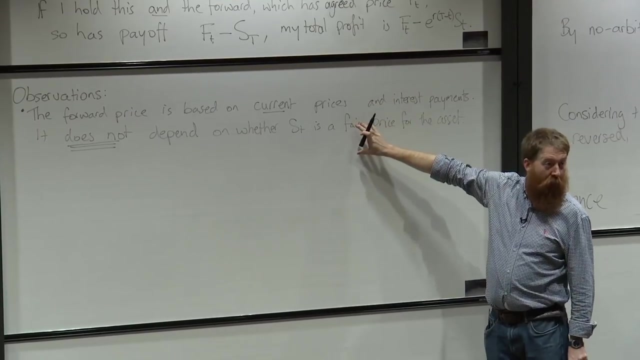 a bad price. this would be a very strange assumption to be making, Because what it's saying is: I can start just buying as much as I like without changing the price Anyway, but our calculation for the forward price actually doesn't depend on whether we have a fair price for the asset at all. 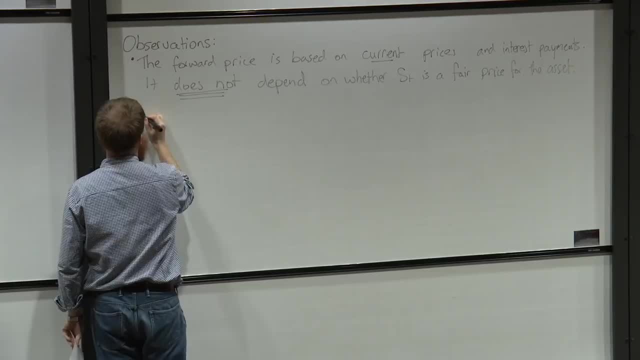 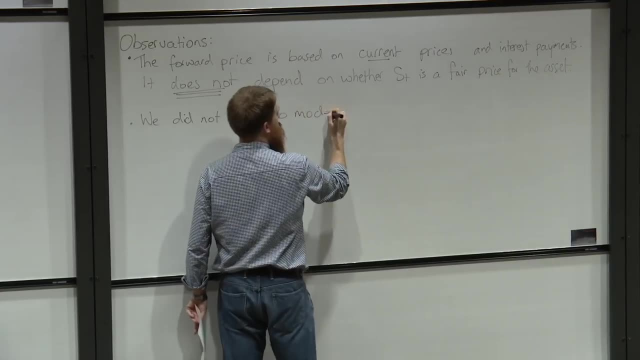 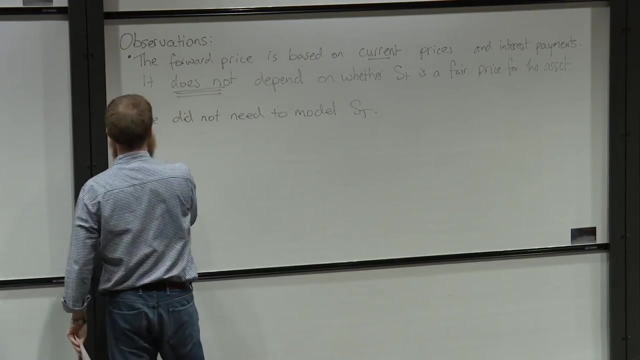 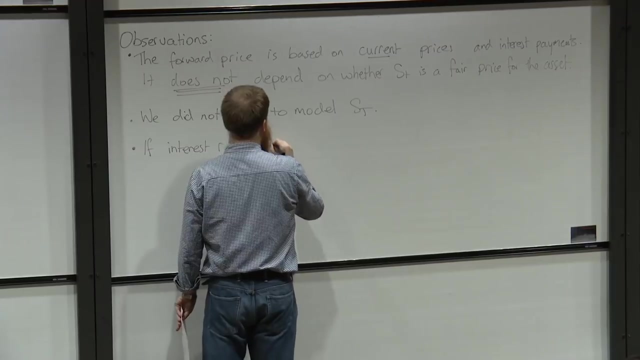 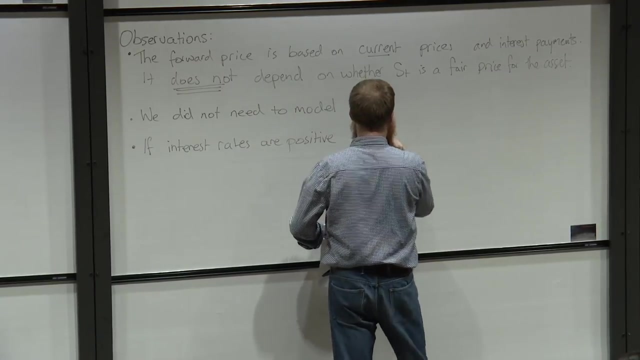 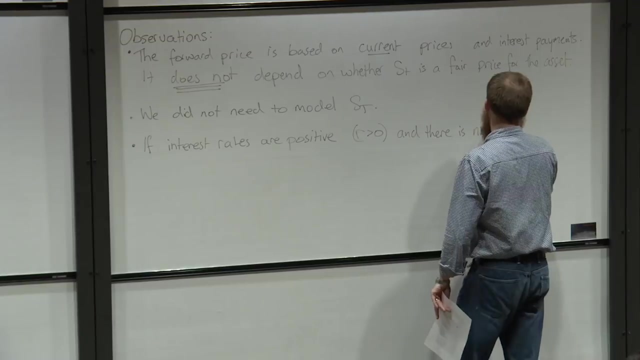 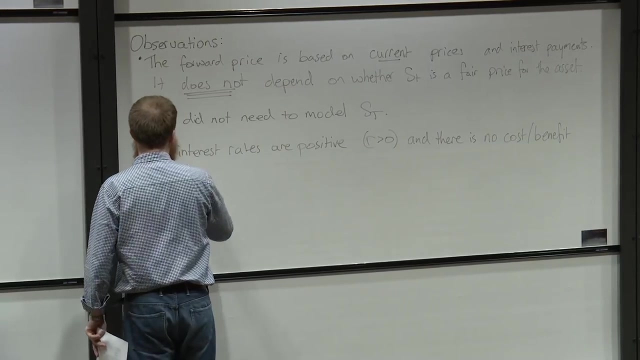 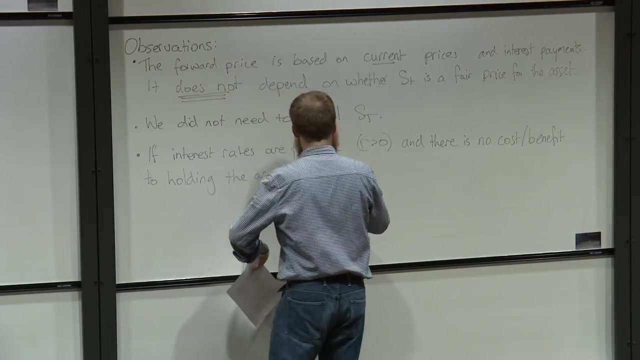 Okay, we did not need to model ST, Didn't need a model for what the future exchange rate will be. So if interest rates are positive- which is usually a good assumption, okay, and there is no cost or benefit, then what we're going to do is we're going to go back to holding the asset, Then FT. 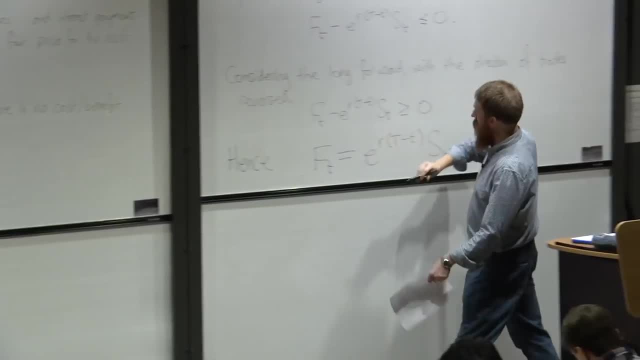 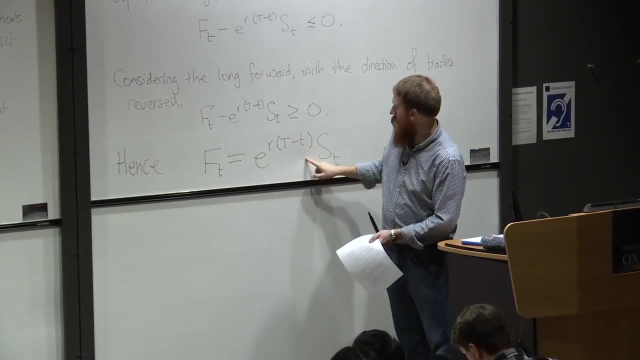 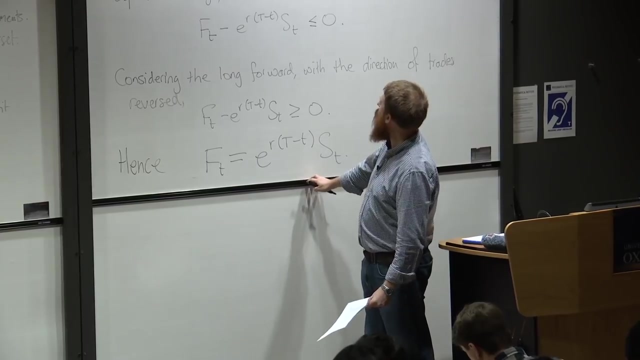 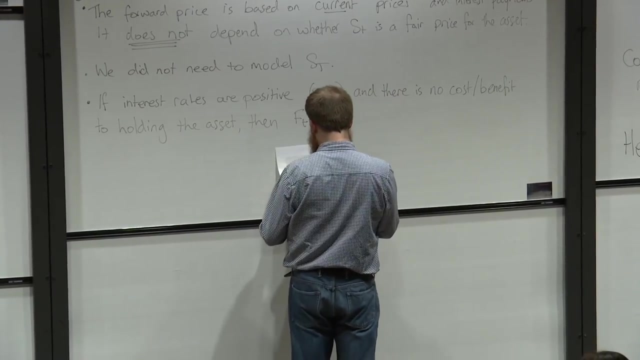 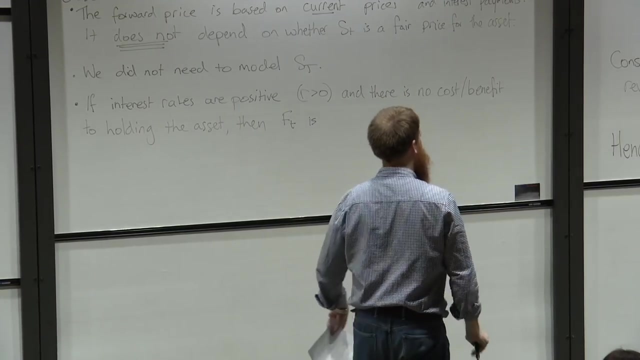 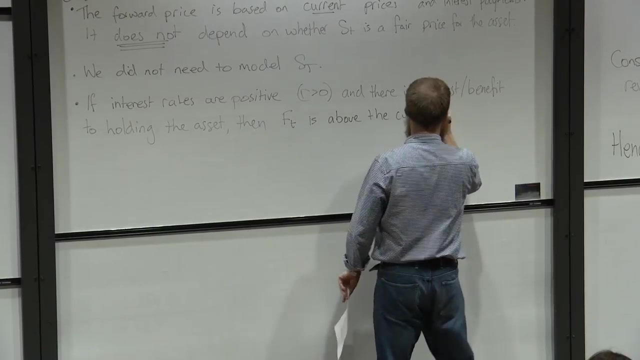 you look at this and you say, well, this is a positive, this is a number. well, if R is positive, this quantity is going to be bigger than one. If I made a silly mistake someone, Well then, FT is above current asset price. 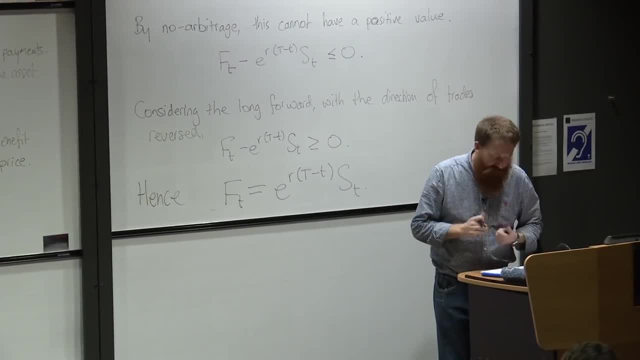 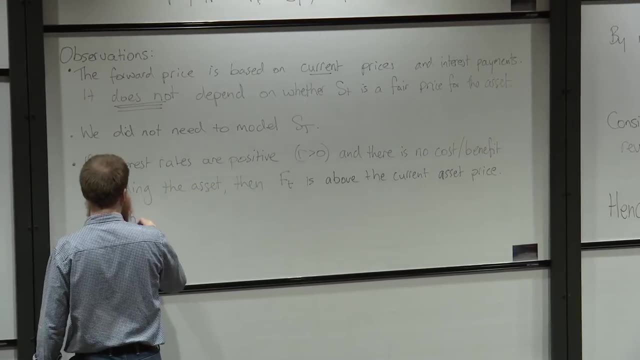 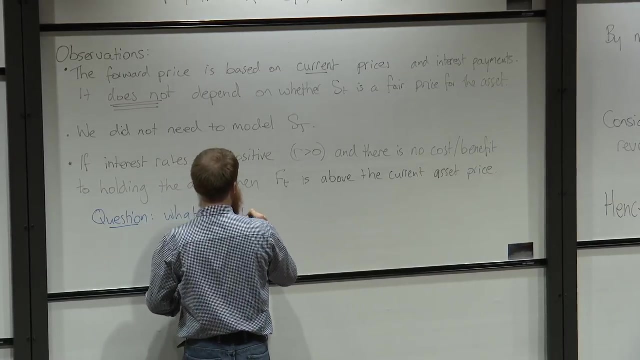 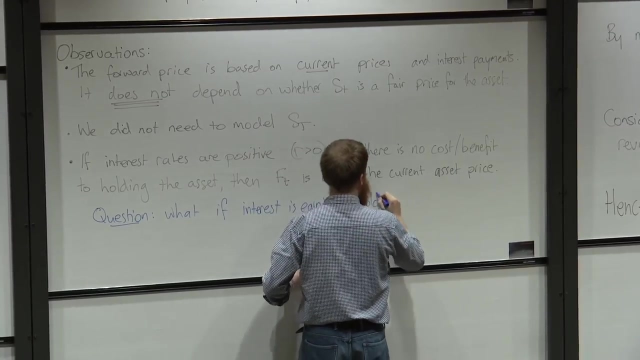 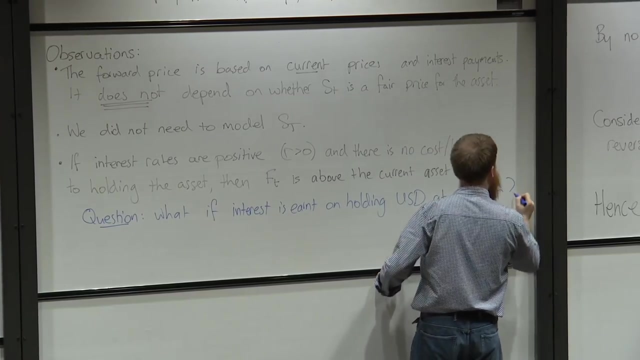 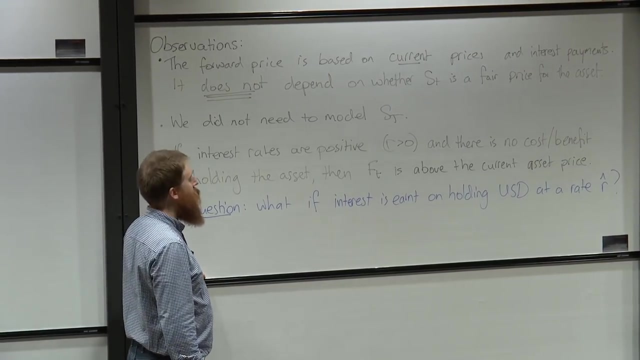 Okay, but we've made an assumption in there. So question: What if interest is earned on holding rate? So let's quickly, in the last minute, say what happens if interest is earned on holding US dollars at a rate R hat. 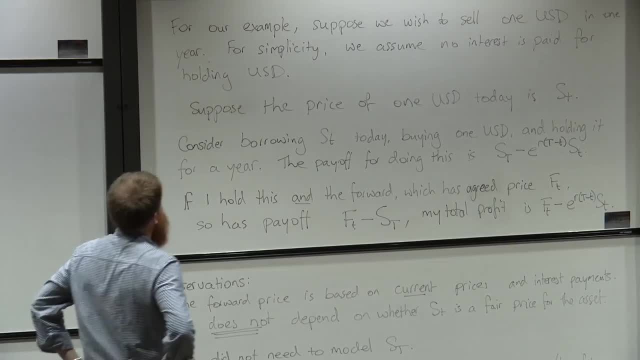 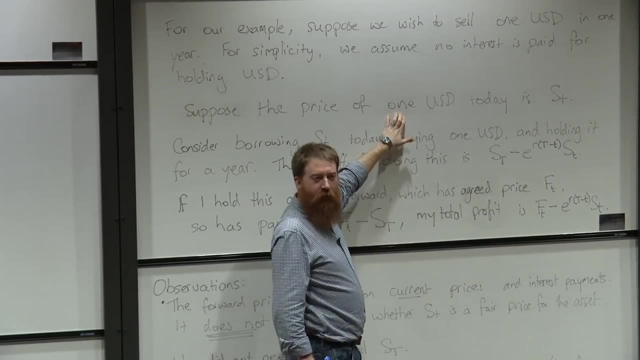 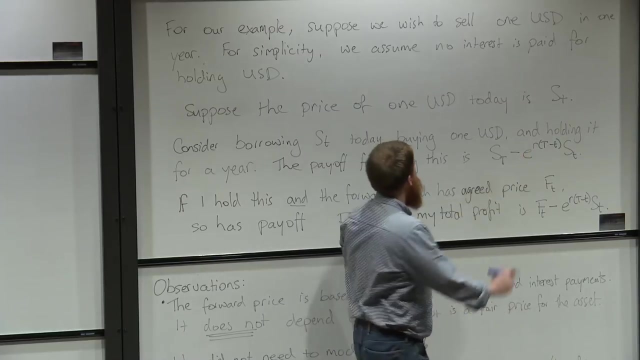 Well, okay, The thing is here. we made our contract about one US dollar, But if I'm going to earn interest on holding US dollars in this deal, I buy one US dollar and I hold it to the end.